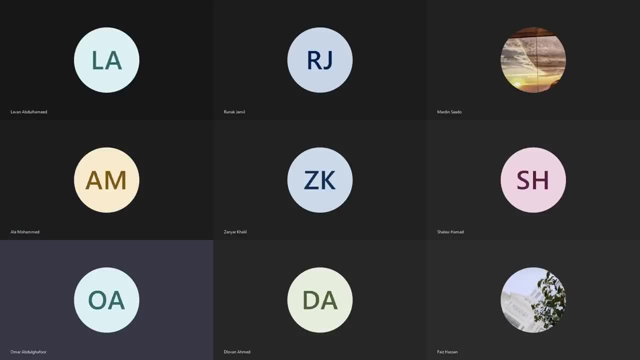 And you can text, I mean, all the points That we have highlighted. And, yes, I don't have any problem for online to be at 3, on-campus to be morning, let's say 9 or 9.30. 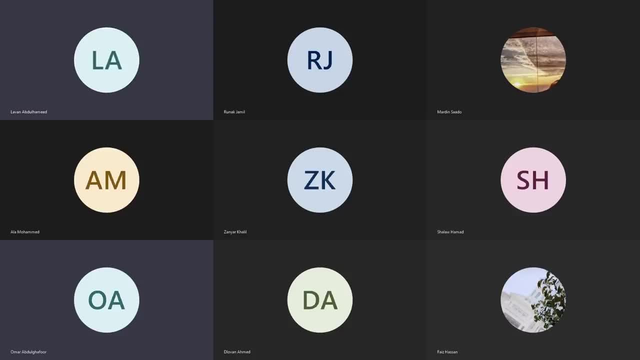 We can start even, no problem, But I don't have everyone's number. Who has everything? The admin Also, I don't have, I mean all I mean I have for Mardin Faiyaz and your number. 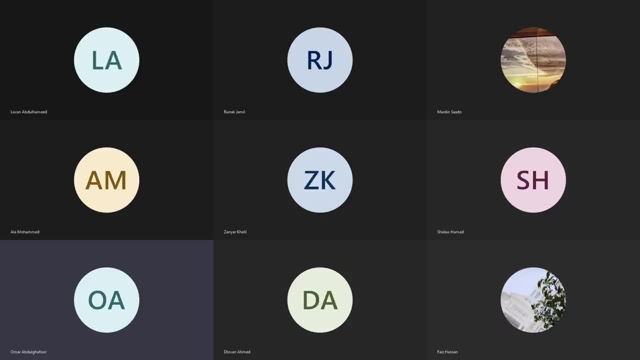 But the remaining I'm not sure. So maybe, guys, you can text your mobile number- if you don't mind your handphone number in our Teams group Advanced Telecommunication System, then LaVon. Or you can text LaVon in Teams. 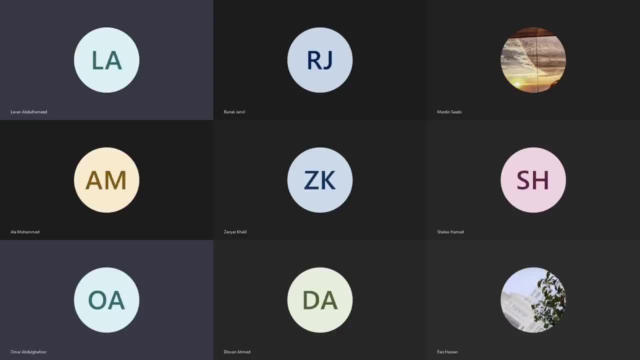 Yeah, please, I mean text your handphone number In Teams. there is a group chat We can talk. Oh yeah, yeah, I mean for fast communication. if you would like to create a WhatsApp group, then I mean, if you would like to keep- I mean- your communication in Teams, then okay. 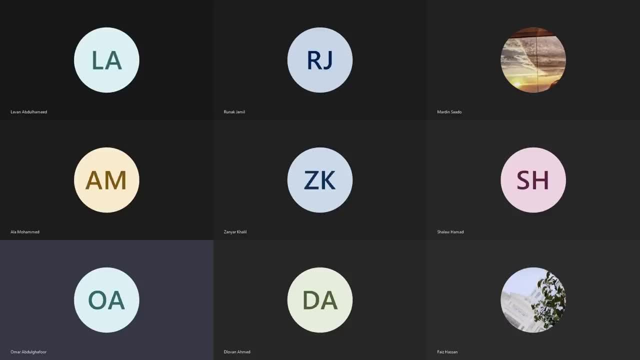 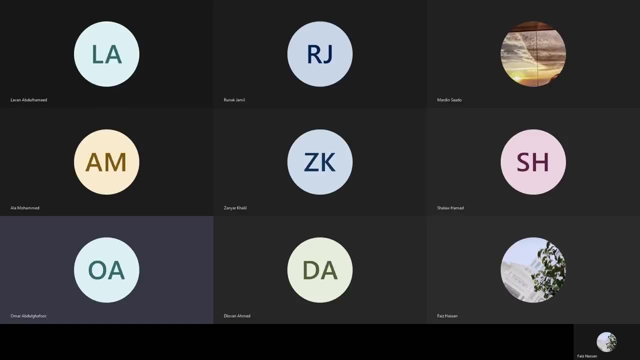 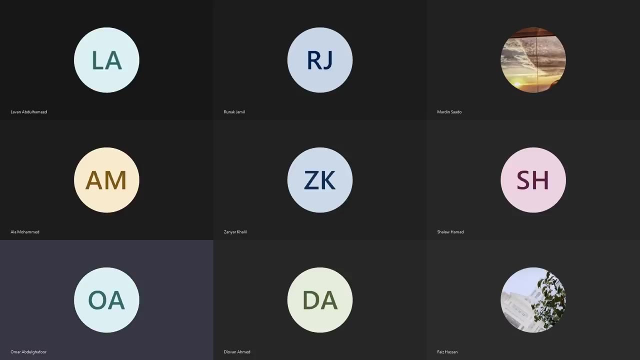 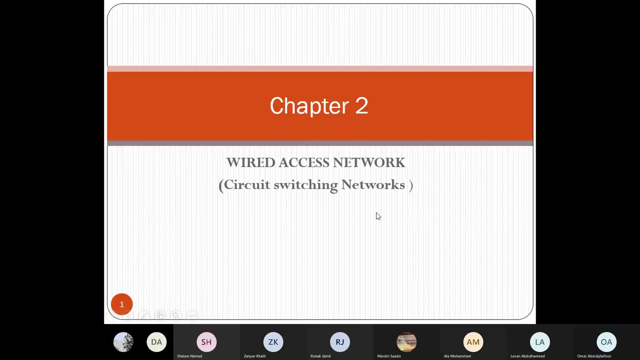 I don't have, I mean, any problem. You are the leader and you can, I mean, follow the approach that you really want. Okay, All right, All right, Okay, Okay, guys. So I think now we can start. 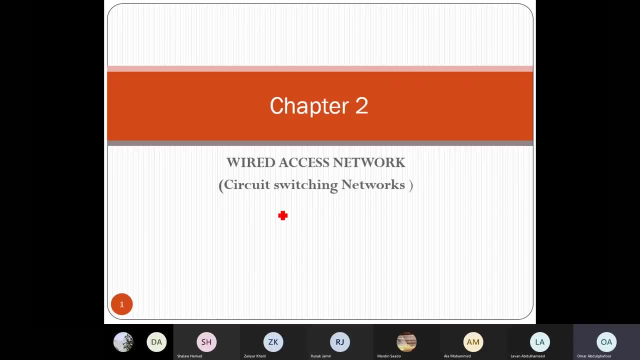 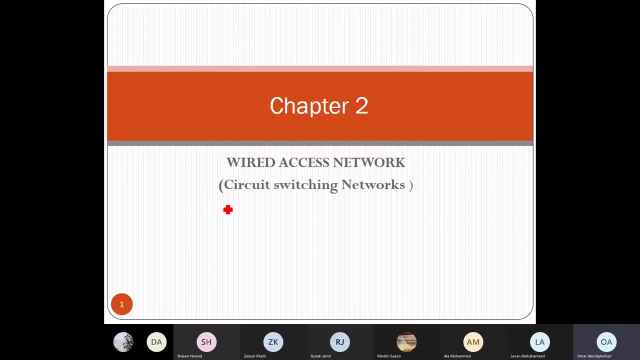 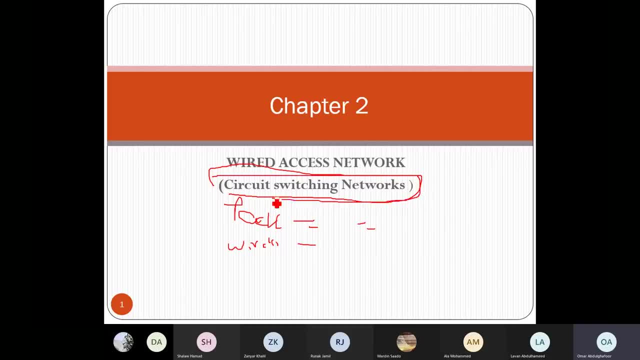 this one- circuits switching network- I will consider only the designing part, all right. so design how we can design a simple network by using some techniques and hopefully I can finish by by today. so next class on campus will be tutorial- all right, because I'm sure that you will. you will ask: 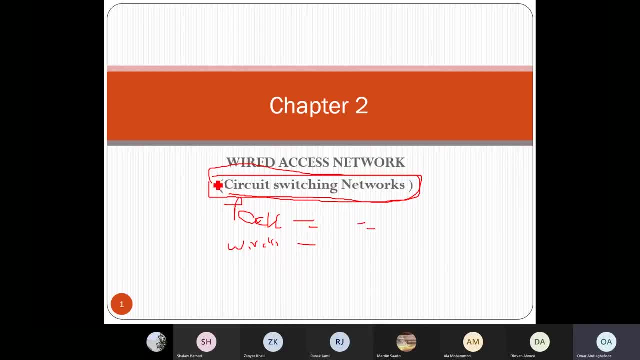 some, some questions here, like how to design, how about the on POTS output and the switches in between. so on campus we I will try my best to make everything clear for you guys, because this one actually, as I mentioned even last week's that in this chapter we will have design question, alright, 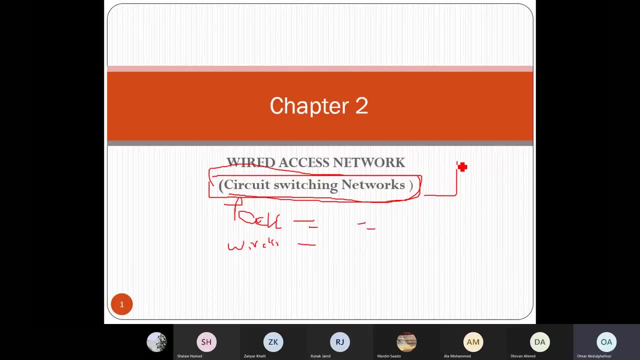 design a question and the level of design. I mean can start very simple: design, ofus design and design. the level of design. it is very simple, value is very simple. so design question and also we can design really advanced. okay, because this one actually depend on the concept that we have. we have. we have done it previously for 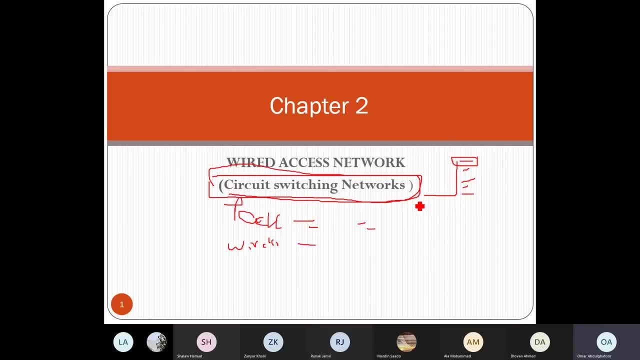 example in in analog communication and that telephony course, because you have some bandwidth, all right, and we're gonna divide this bandwidth for some users, all right. so each user for sure will occupy some bandwidth, and and after that we need to use some multiplexing technique like frequency division, multiplexing or 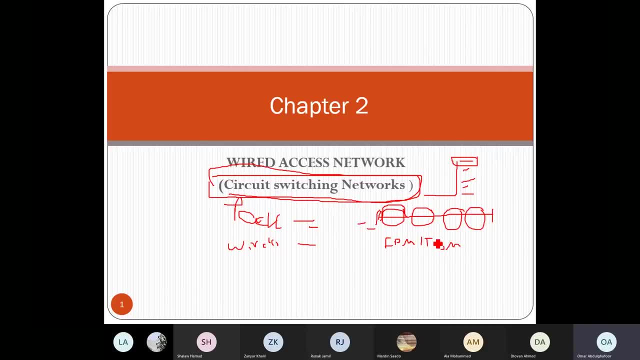 time division, multiplexing. then we have to recall some, some concepts. so I'm sure that you will have some, some concern related to concepts that we have done previously and also the design. so that's why I really prefer to conduct some classes on campus. I UK, especially for 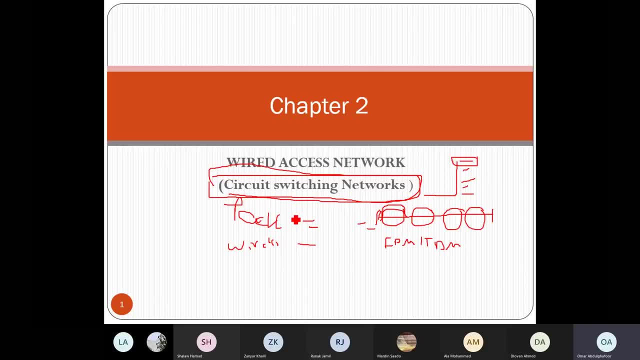 the tutorial. so we explain the concepts online, but when we would like to practice design, then I really prefer to have an face-to-face discussion with you guys for better understanding. similar to previous chapter, I have uploaded the tutorials, the tutorials. it was seems like it simple, some of of the questions, but some of the questions we when we explain on on. 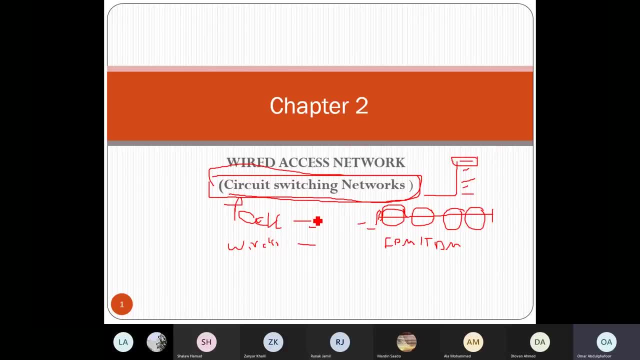 whiteboard. when we have more discussions, the idea I mean becomes clearer and clearer. all right, so this, this chapter, will be the first circuit, switching networks- and after that this one will be the second packet and we will move to the wireless. in wireless, as I mentioned this one, we have 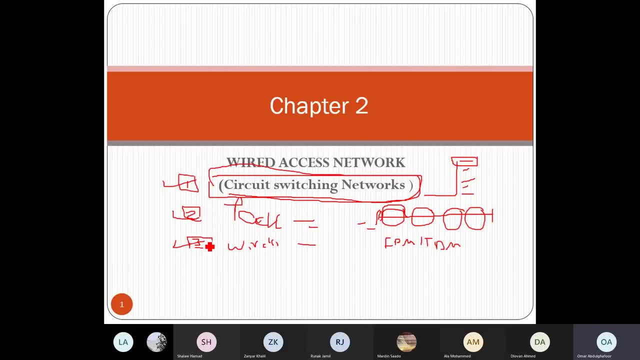 briefly discussed and this one we have briefly discussed and also this one we have briefly discussed, so in in packets also. I will not really go in really details. I will focus on the main concept and for wireless we will try to discover the JIS technologies, starting from 3 G and three technologies starting from Scott. that was y j punya. 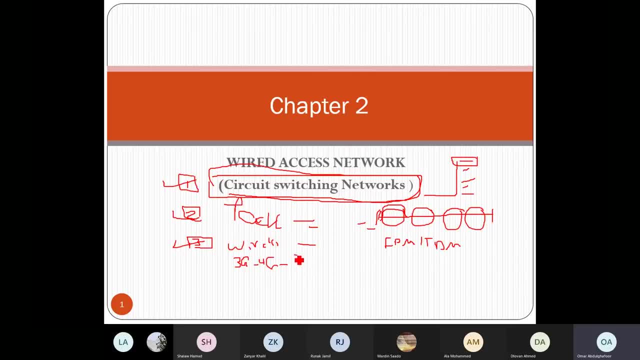 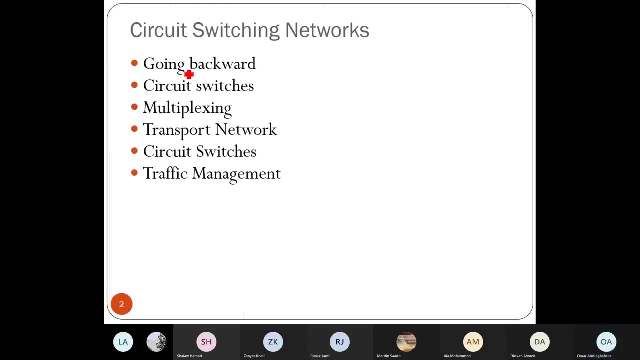 4g and we will try to, yeah, 5g and we will try to touch the latest uh technology, which is the sixth generation, because the research already started on on on this technology. all right, okay, so the um, what we call it, the content will be circuit switches, multiplexing. 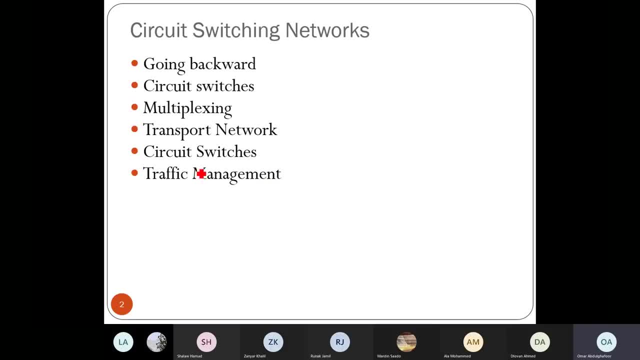 transport network or circuit switches, traffic management- this one actually i will, i will try for for this one, this one it's um uh congestion or traffic management, or error detection, all will be in this uh topic, but we'll focus mainly on this one: circuit switches and multiplexing. all right, so the design. 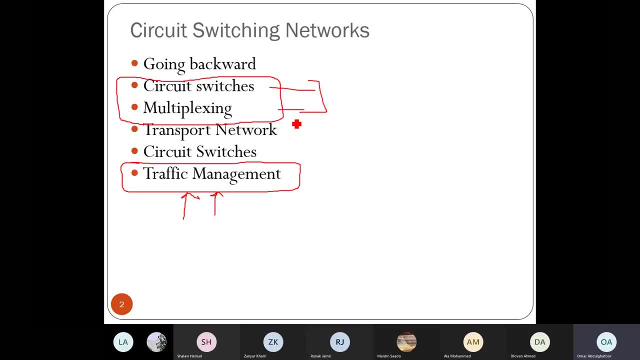 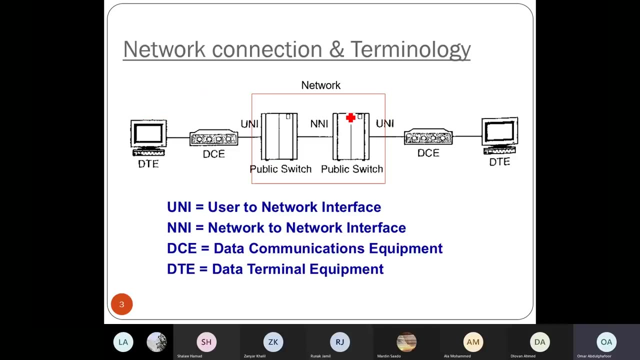 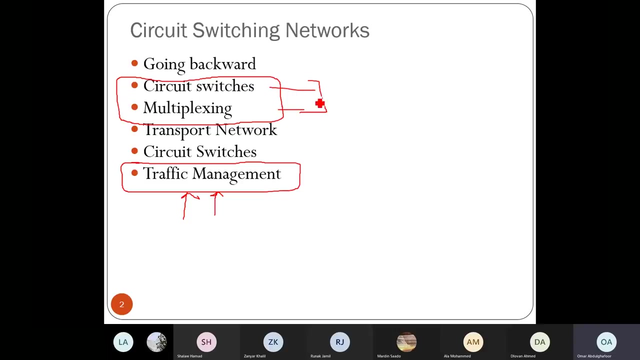 will be this one and this one. these are the most important actually, topics that related to circuit switching networks. so now you have an idea about. you have an idea about certain circuit, uh, circuit switches. if you remember, last last chapter we said that it's um, we have three phases in in this case. we need to establish all right, the 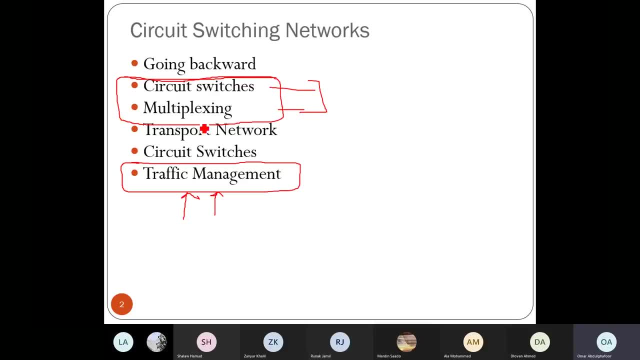 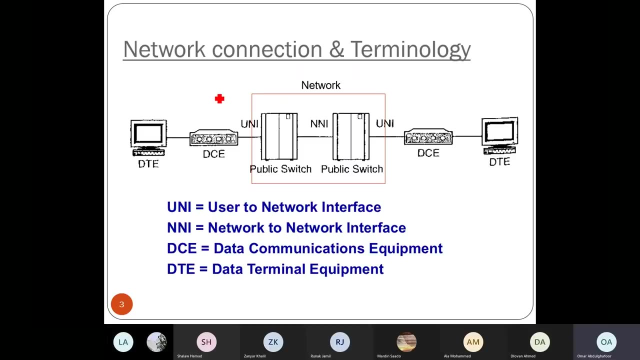 the circuit or the switches, and after that we need to link and after that we need to release. all right, so three main uh faces in this, um, what you call it, circuit switches. all right, so this is actually the general graphical representation. all right, so we have, for example, a two pieces i would like to 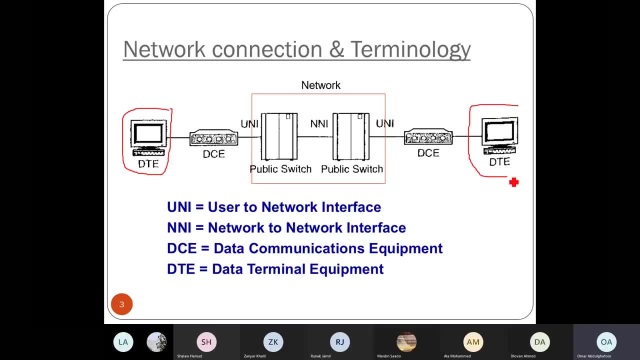 communicate all right with with each other. uh, so the the component and connections, either we can not, or terminal or or whatever. for example, here dte, it's data terminal equipment, but it's not necessary to fix with this number. with this i mean with this name, either node node a, node b or or whatever name. and we have a uh network here we have data. 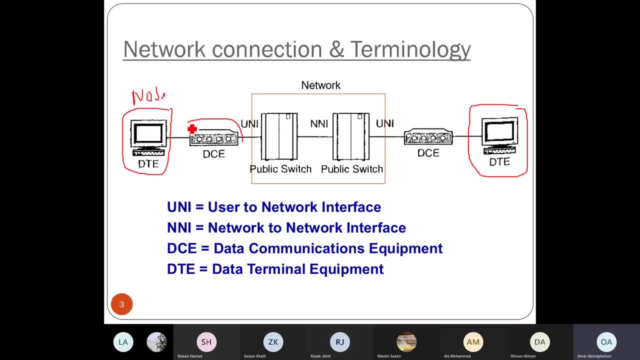 communication equipment. all right, so it depends. all right, data cop kobe is the little box for us that we're going to touch here. it's called method connected t balt, and we have user to network interface, this one uni- user to network interface, user to network interface and we have network to network. 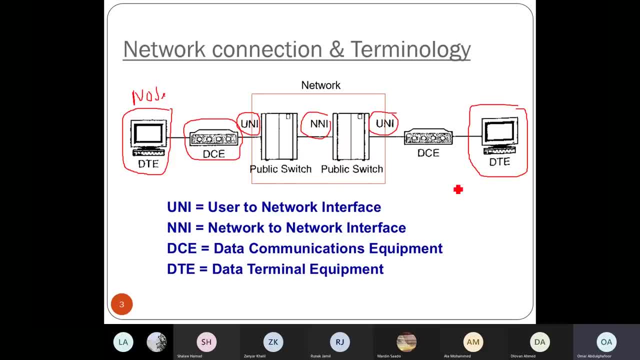 interface. if we have, for example, a remote, then from one network to another network, this one actually communication. if you, if you remember the figures that we have explained in wireless communication, if we would like to communicate within the cell, all right within the cell. so you need from base station to mobile, all right from base. 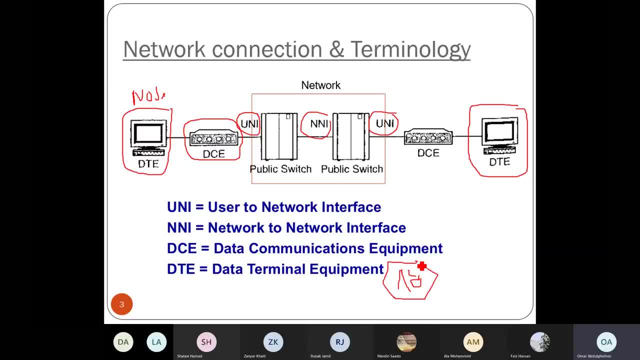 station to mobile. so if you would like to go for communication for another cells, all right, another cells, then this one will communicate with its base station. base station will forward it to another base station, another base station to another base station, then after that downlink to the mobile. so when we said network to network interface, if we are talking about 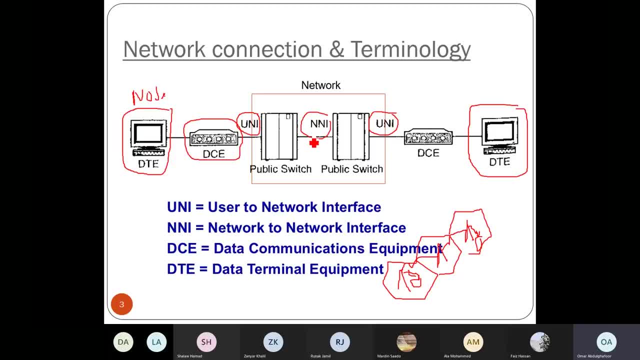 telecommunications network, in terms of wired, for example, will be same in terms of wireless. but, for example, here will be, instead of network to network, this one will be base station to base station, all right, and even, for example, in, for example, here we have user to network interface, also here we have in wireless. this is the 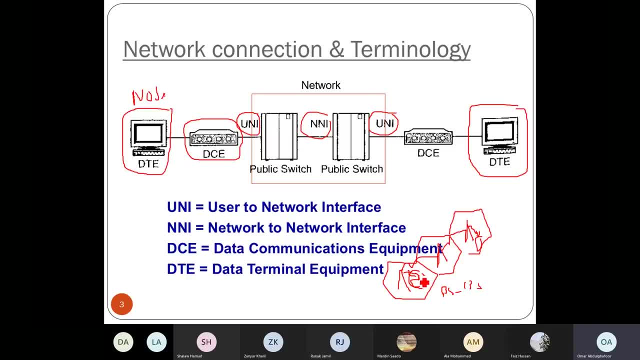 user to base station. for example, if you are using your mobile and would like to change your your cell from this cell to this cell, all right, then this one we call it the hand over. all right, so user to network interface in in wireless, we call it hand over. 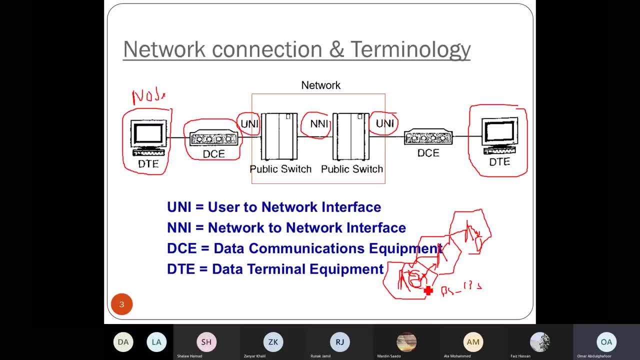 strategies. that mean this base station taking care about your call and you are moving away from this base station, moving toward this base station, then we call it the handover. so in terms of terminology actually is almost, almost like. i mean, i'm not saying is a standard, but it's really similar to. 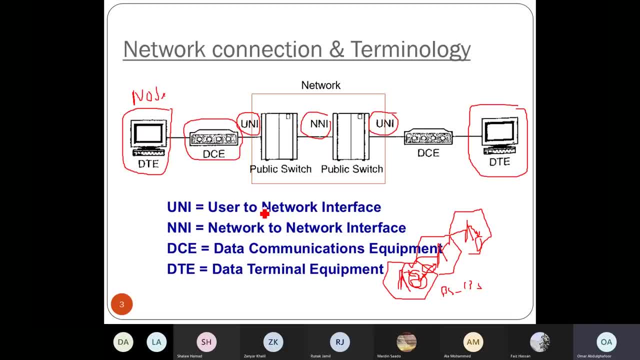 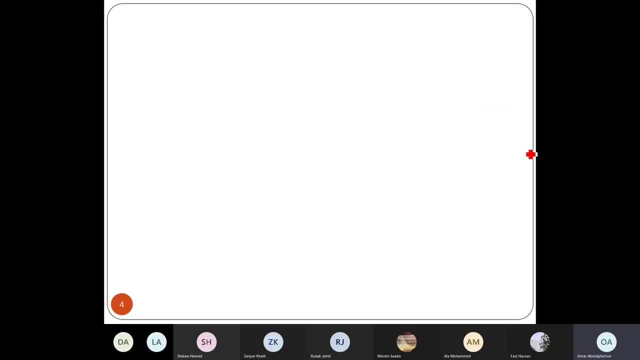 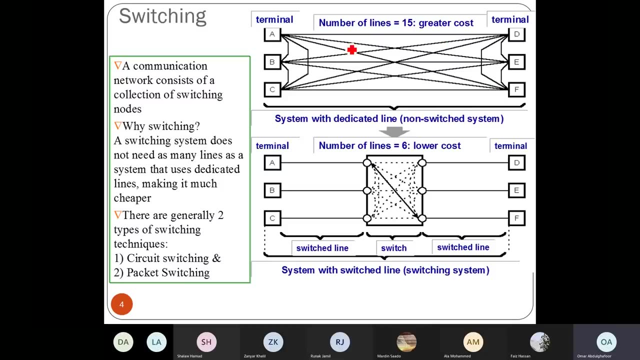 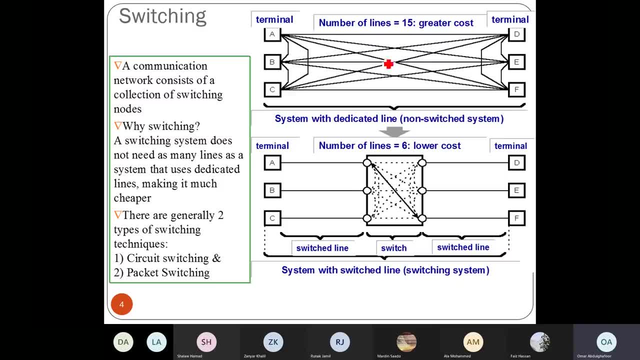 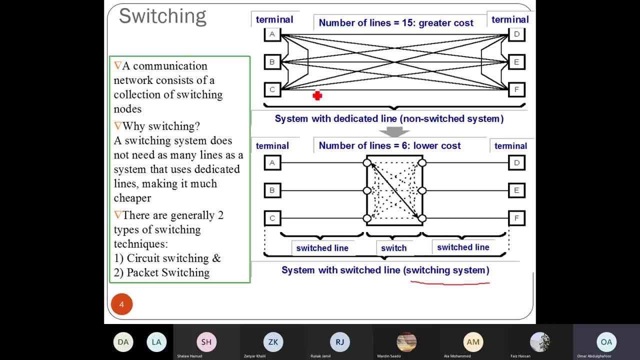 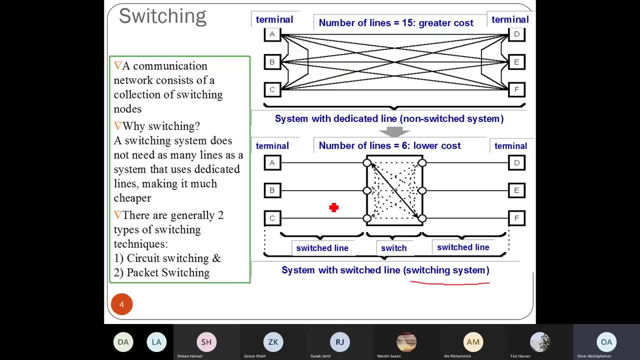 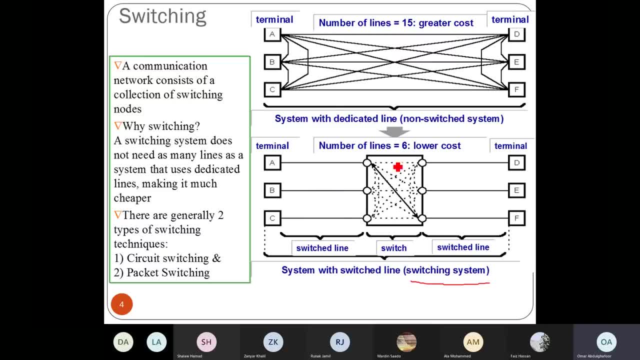 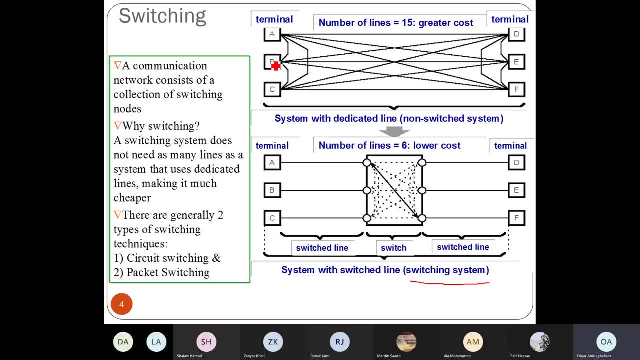 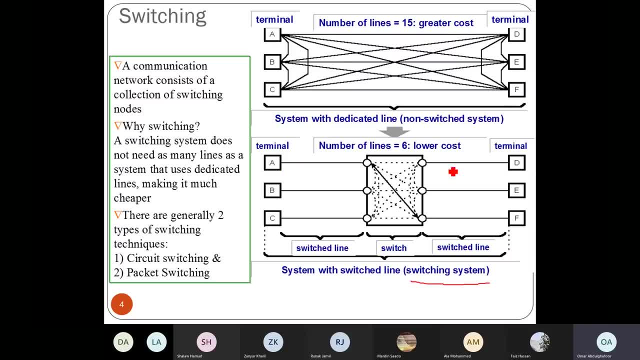 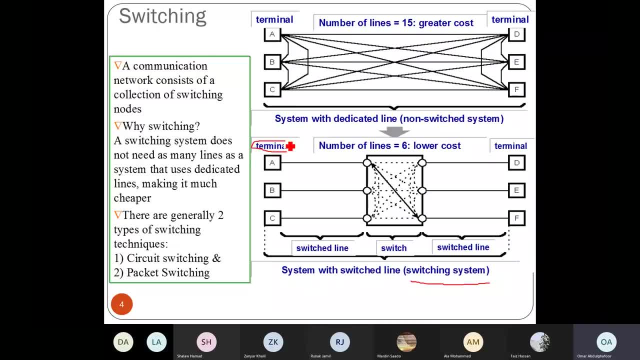 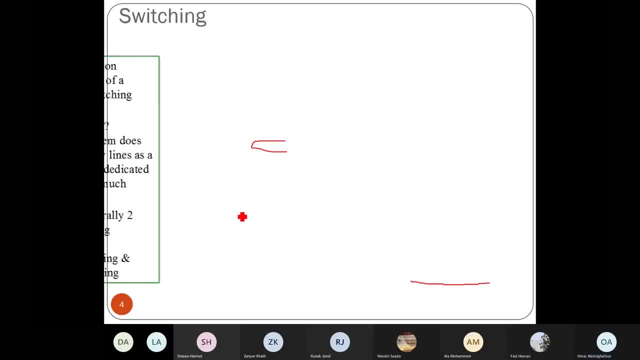 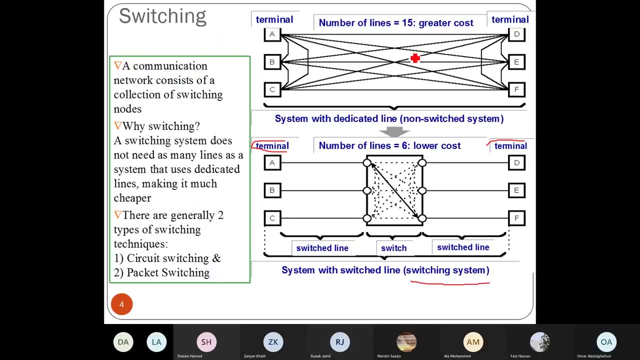 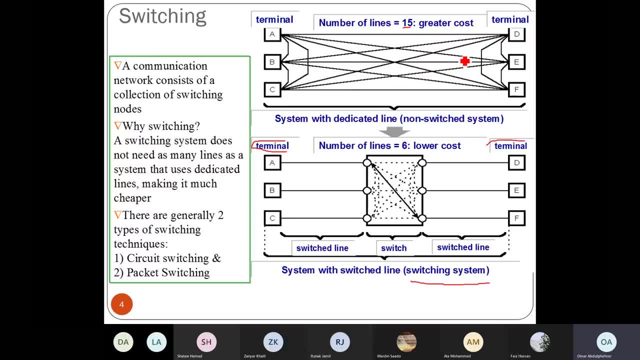 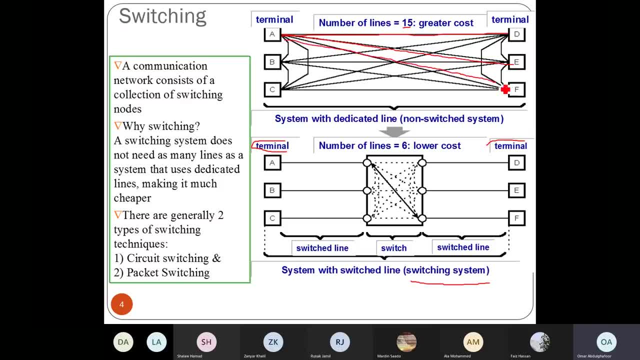 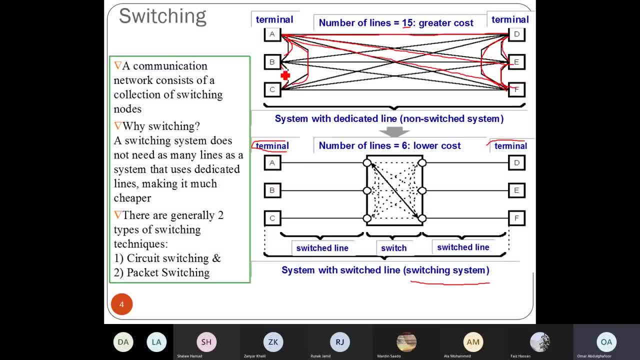 with c and a with c, and also same goes with b, also the gate line with d, with e and f, and so on and so forth. but in terms of switches, i can replace all this one by center switch in between, all right, center switch in between, and i have one, two, three, all right, one, two, three connections terminal a. 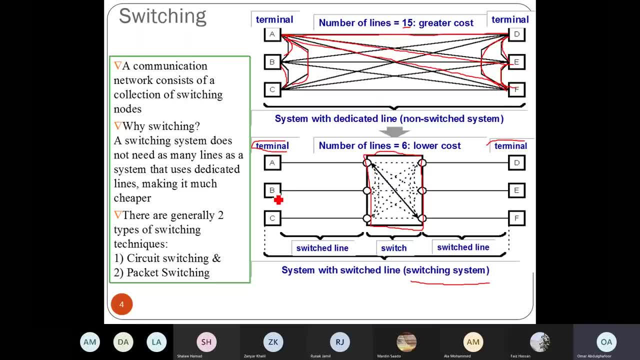 goes to the switching center by one line and terminal b goes to switching center by one line and c also goes to the switching center by one line, and same for the other side. d and e and f connected by one line. so, whatever, i don't care about the communication. for example, a would like. 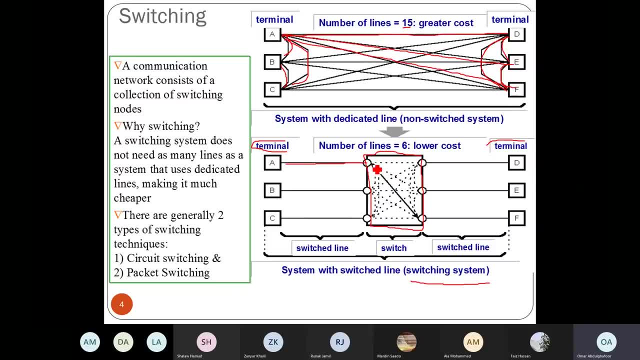 to communicate with f. this one line will be active and the switch in between can switch back to this line and i can reach here you. instead of the messy dedicated line, i can put the central switch or exchange office or whatever we call it, in between. then i care about the terminal here inside. the automatic switch will take care. 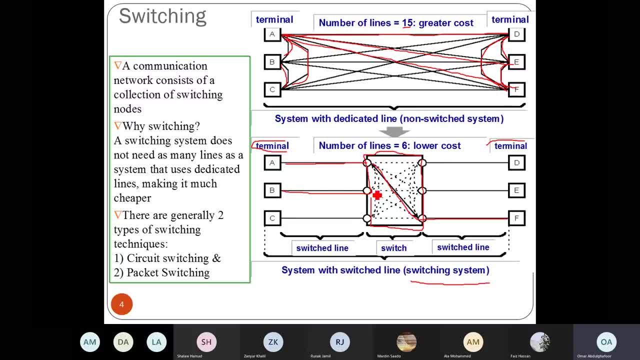 about the destination. all right. so coming from b, also, there is a switch. i would like to go to d, for example, switch here and i will go to d. from c, for example, i would like to go to e, to the central switch, and i switch here and i go to d. 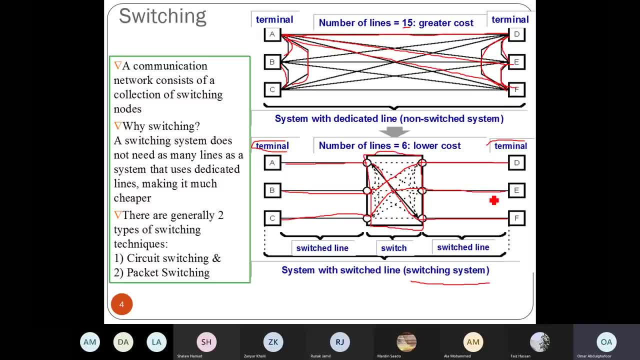 directly to E, and so on and so forth. So in this case, for example, this one is will be more efficient compared to the previous one. So this is our, our, our final goal? The answer actually is no. We have some other techniques that would like. 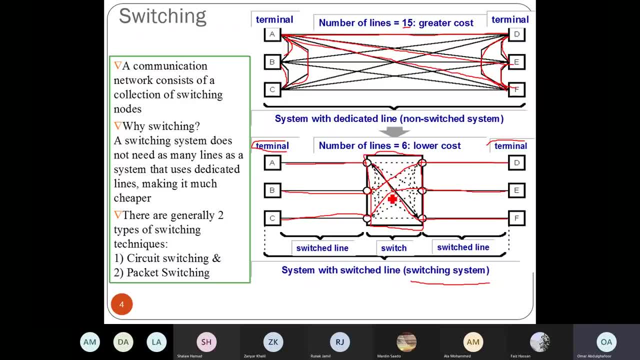 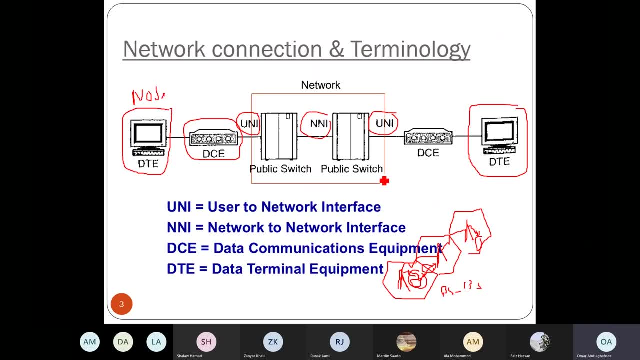 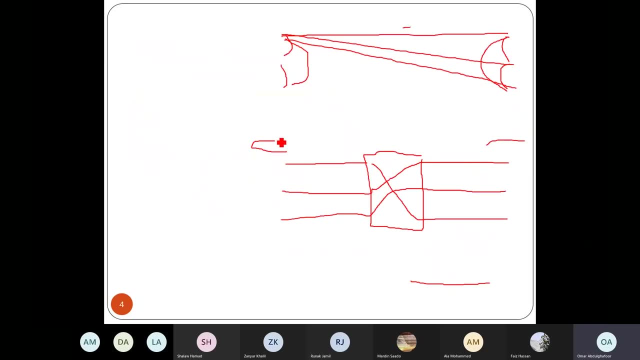 to to discover, because here, if you would like to, for example, increase this one and increase this one, Uh, the, as I mentioned here, Um, The design, all right. here I said we need to design, I'm right. so here is just a box. 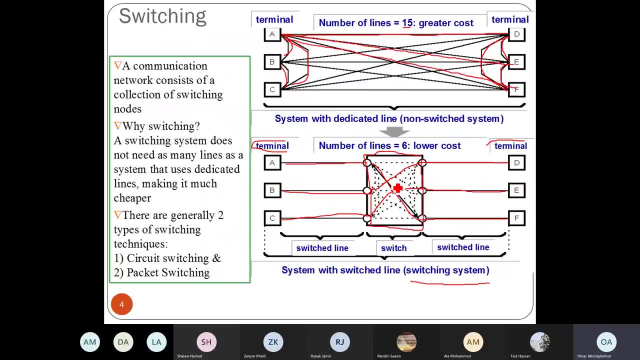 Is the box, but what is inside? We're going to discover and we want to design. So here also is a is we have what we call it, the in terms of computational complexity, in the complexity of the switching also will be high. So this is actually is not our. 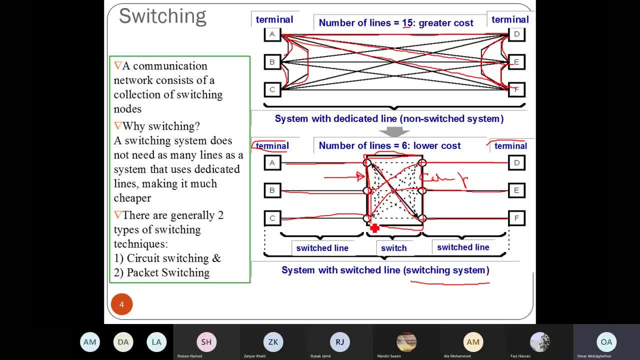 our final goal, The box. here We have Uh, many to do inside, All right, many to do inside, and different techniques. you will discover afterward And you will try to design our own. Alright, we'll try to design our own. So our communication network consists: 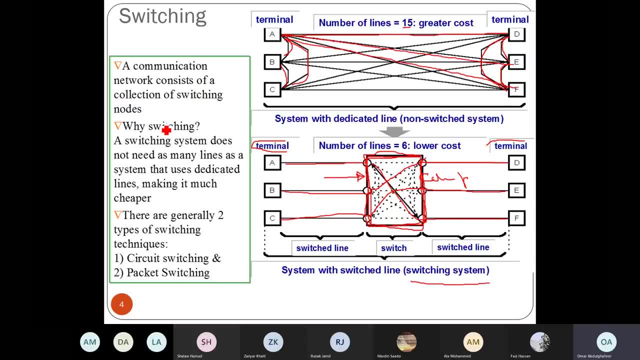 of a collection of switching nodes. And why switching? We said that the switching system does not need as many lines as system tattoos. in this one, The normal one, dedicated lines Make it much cheaper in terms of cost and also it's easier to handle. Alright, you can see that, two figures and you can. 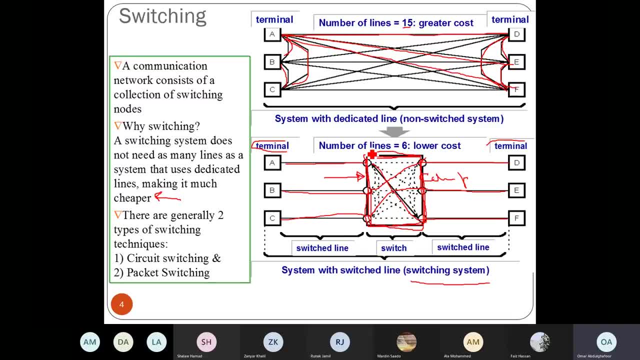 compare. Alright, how it looks like, And this one for sure will be more efficient compared to To the dedicated The lines. Alright, so there are generally two types of of switching technique. Uh, as we mentioned, circuit switching and packet switching. 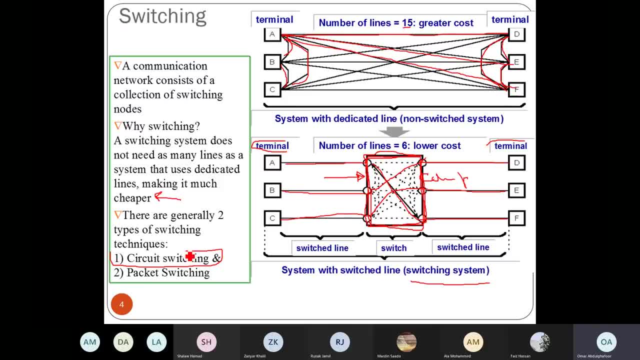 Alright. so we are here, actually We are here in this chapter and we have another chapter to deal with the Picket switching. we have, I mean, provided some Introduction about both in previous chapter and we compared circuit switching with the packets switching. but now 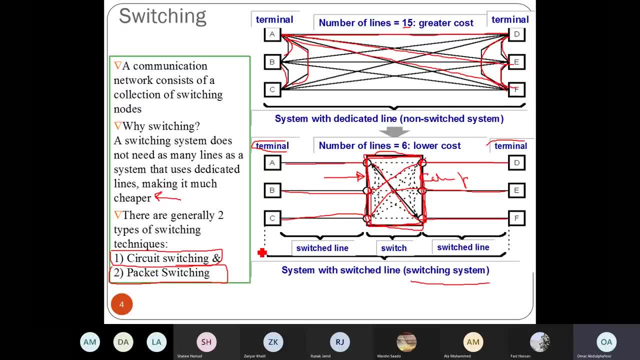 actually we're going to, Uh, Uh, discover some, some details related to both switching techniques. So this is actually general circuit switching back, switching inside. We have Some, some uh techniques, some details and some design procedures. Alright, OK, so this one, actually the switch line, This 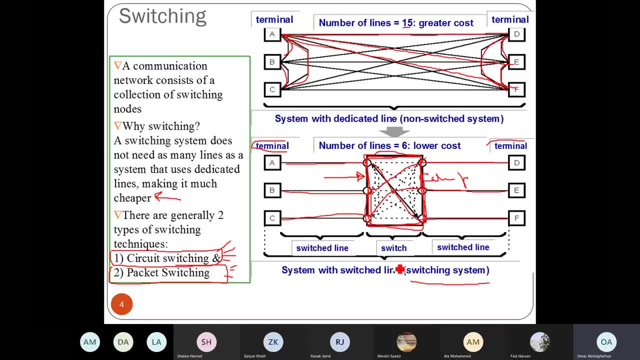 one, the switches inside, Alright, switches inside. and here, for this also, we have a switch line. This one, the switches inside, Alright, So we have a switched. Uh, switch lines. alright, So this one for sure will be Lower cost. alright, lower cost compared to the to this one. but 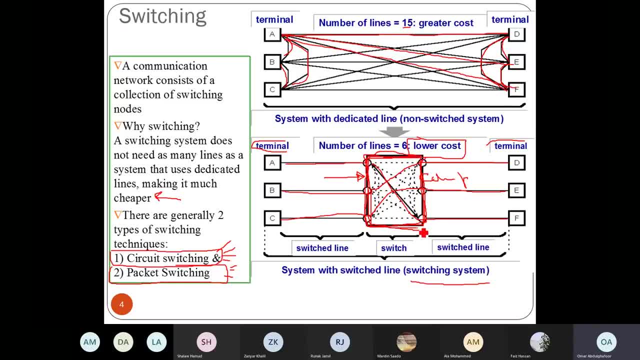 again and again inside the box, we gonna design. alright, we will have a design, Uh, this one, the switches According, different technique. we have different technique, either crossbar or Or space, alright, and The one that we briefly explained in the previous chapter. we're. 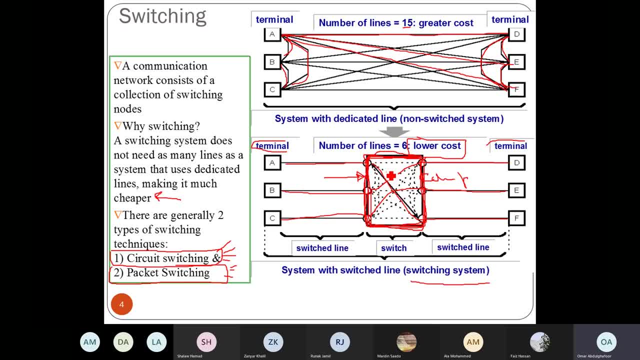 going to design in some details. OK, so again, we will. We will see that this one, Actually it might be very simple design Or it might be really difficult. OK, so I will provide you with a simple one, Maybe by today class, and 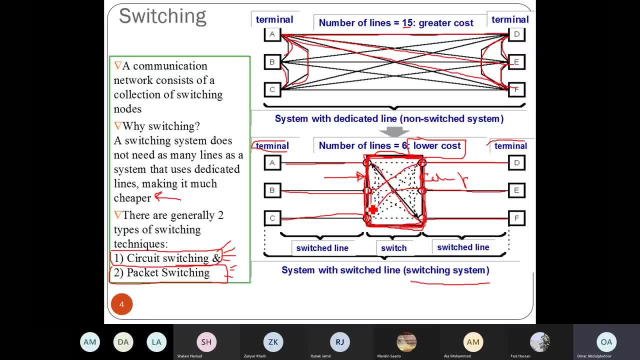 In in tutorial I'll provide you a little bit high and maybe in midterm exam will be Uh, some, Uh difficult design, um design equation. Then you have to really think and recall some, some concept that you have learned In order to provide a proper uh, a proper design. 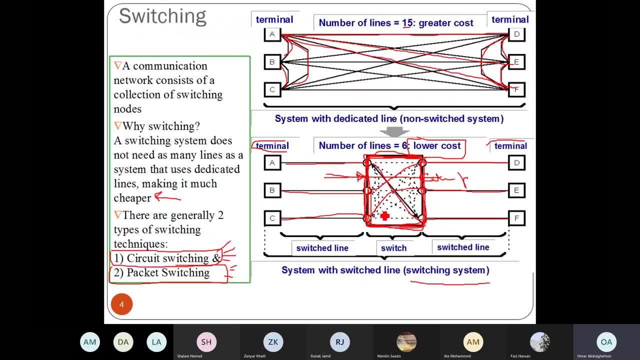 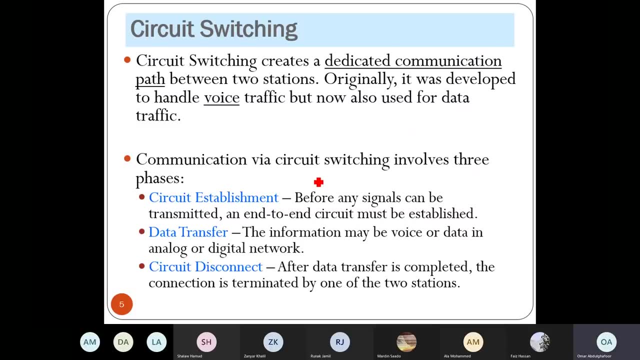 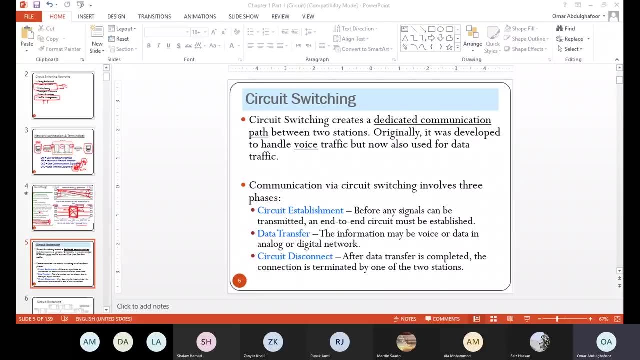 OK, anyway, And also, guys I'm planning to the midterm will be on the midterm, Uh, on campus, Um, uh, planning, and I will. I will let you know, maybe by end of this week. Alright, How are you having? 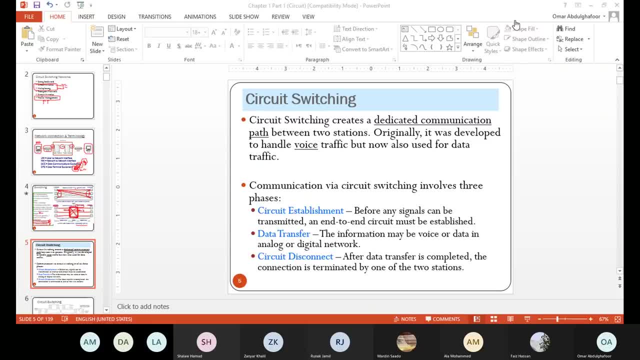 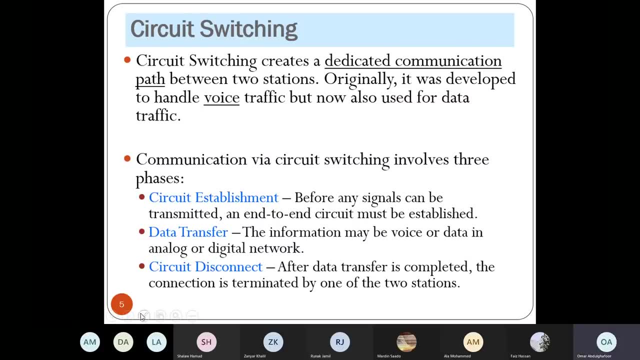 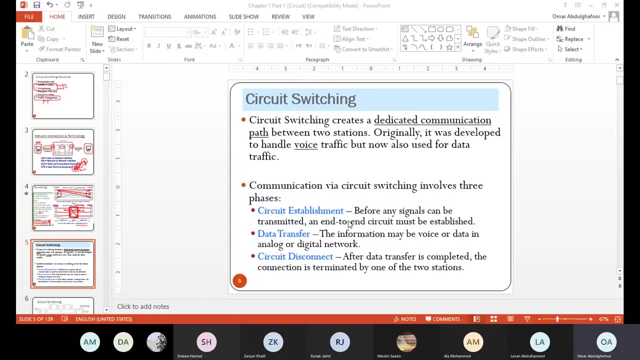 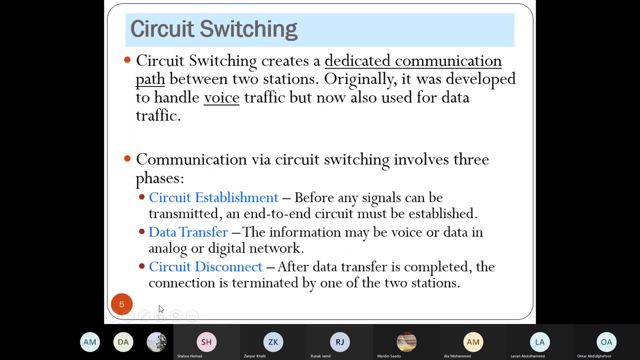 OK, Alvon, or love on, Sir. I think everyone is here. It's long time nosy haven't, Are you OK? Alright, anyway, OK, Okay, All right. So circuit switching: We said that circuit switching creates a dedicated communication path between two stations. Originally it was developed to handle voice and also can be carry data. All right, Like we said that in packet switching, we have virtual circuit switching. All right. 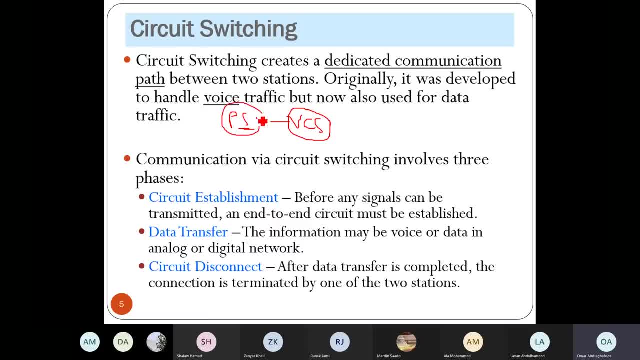 So we have virtual circuit switching inside this one, So this one packet- actually it's for the internet and this one can be part of the packet switching So it can handle, I mean, voice and data And this one the faces. if you remember that we have highlighted in previous chapter circuit establishment. 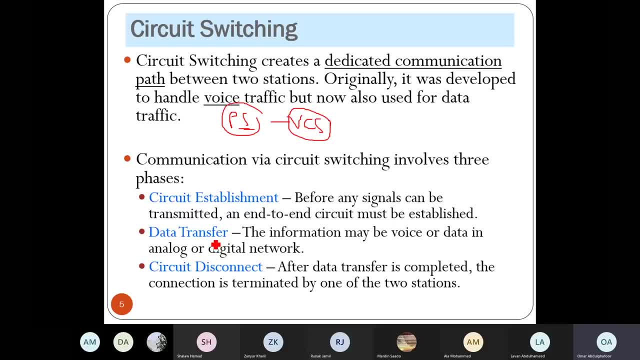 And data transfer and circuit disconnect. So that means we have a procedure when we are dealing with circuit switching and packet switching on demand. If we have a data to deliver, then the link. after that there's like we have a pool of links available if we have no data. 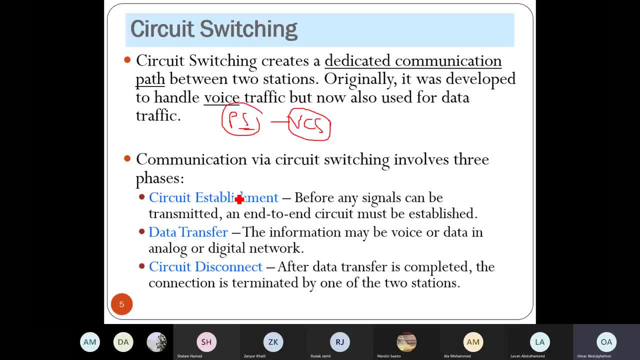 But this one actually is a procedure. we must actually follow exactly Establishment before any signal can be transmitted, And end-to-end circuit must be established, All right. If there is no available, then we have a block, All right. There is some blocking probability and we have some another technique to reduce the blocking probability or to avoid some blocking probability. 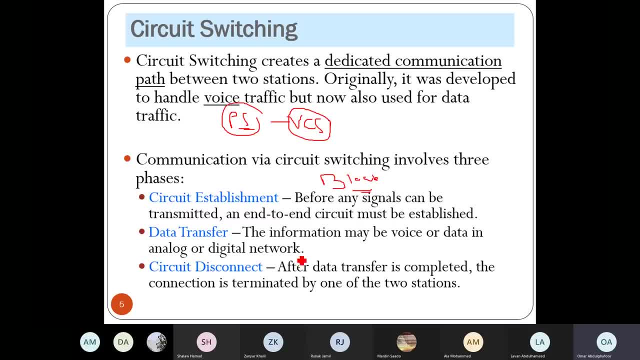 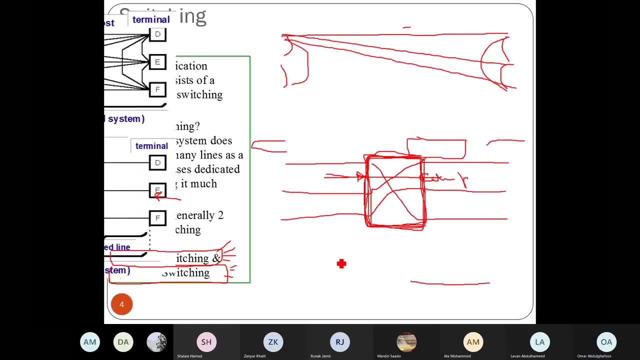 And data transfer. the information may be voice or data in analog or digital networks and circuit disconnect after data. So the data transfer is completed, The connection is terminated by one of the two stations. All right, So like here, If you would like to communicate, then this one must be established. 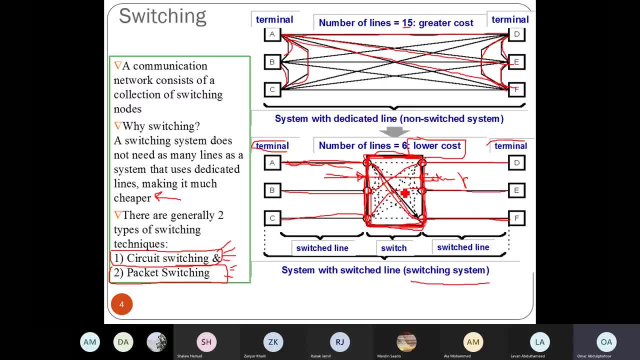 All right, And data will follow, And after that, this is, the switches will be terminated. All right, So the switch. this line will be available again for any other node or terminal That would like to communicate with another terminal. Okay, 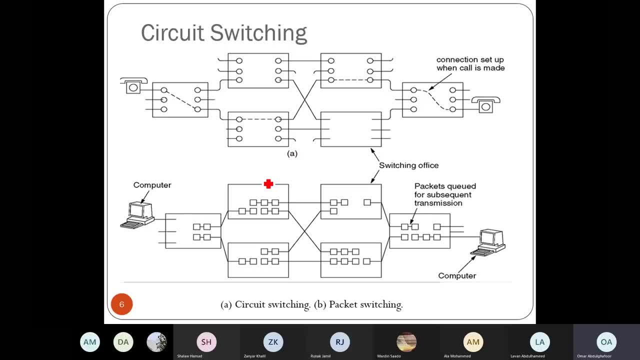 So this is an example actually of both circuit switching and packet switching. All right, So here we have a terminal. All right, We have a terminal or node would like to communicate with another terminal or node, And this one same goes for packet terminal. would like to communicate with a terminal. 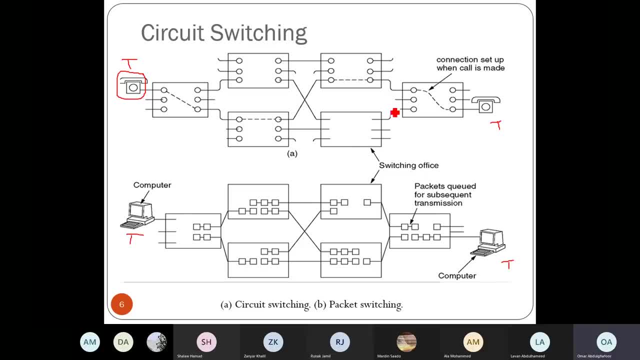 So, in terms of switches, you can see all these are switches, switches, switches and switches. All right, So this one, this one, the one that I already mentioned to you, we need to design. Okay, So we need to design, depend on some giving information inputs. 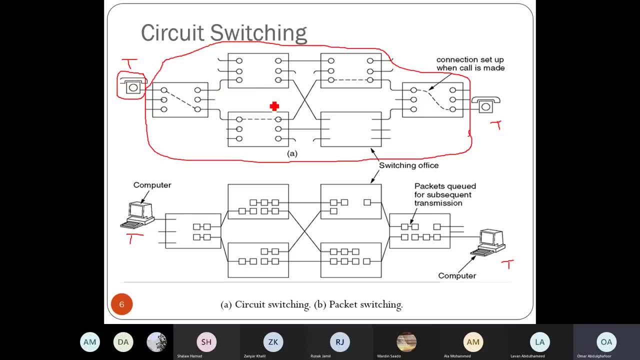 Then we have we have to design And we can calculate the computational complexities And we can redesign. I mean design by using some procedures, And we redesign in order to minimize the blocking probability. And also we can combine this design with some multiplexing technique, like frequency division multiplexings or time division multiplexings or any other multiplexing technique. 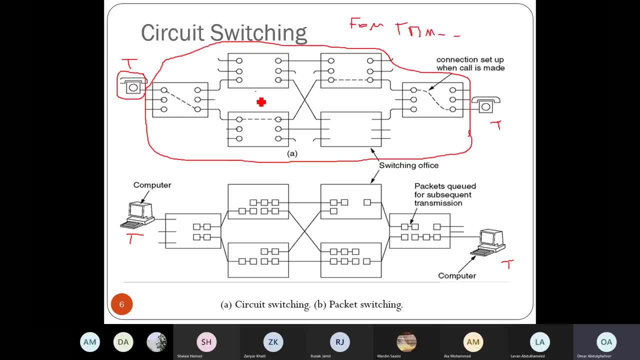 So here Here our design looks like blocks, some blocks. Each block has some output and output, And in between also we have some blocks that connect the first and the second. All right, Or the last stage, We have stage. 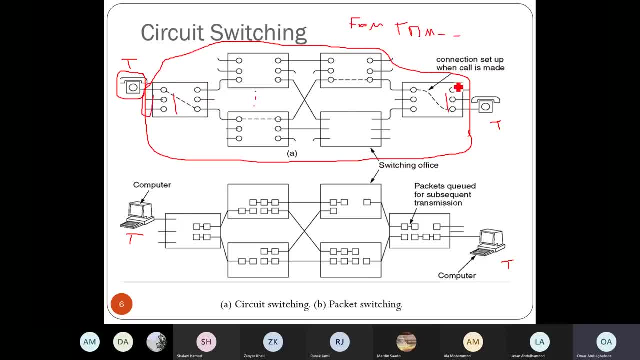 We have stage. The output here must be the same of the output. So, for example, when I said 200 times 200.. All right, Then I assume that this one is: I have From 1 to 200.. The output from 1 to 200.. 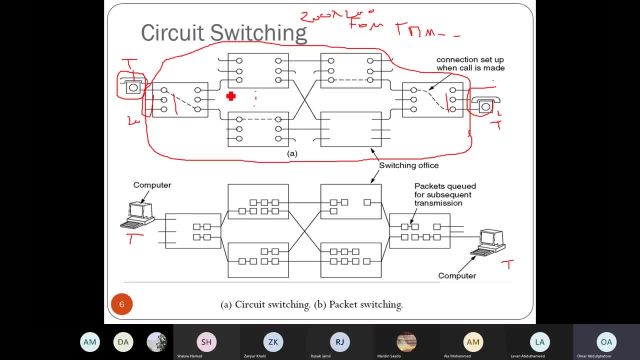 And in between I need to design- There are some procedures, All right- And the block in between until I reach. I mean connect the input stage and output stage. So this is the input and this is the output, All right. 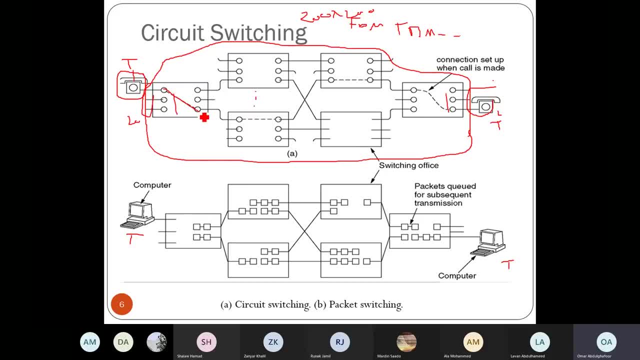 So when this terminal would like to communicate, then the switches connect. For example, I can connect to this one Or I can move to this. All right, If I follow this one, there's some connections, All right, It depends on the availability. 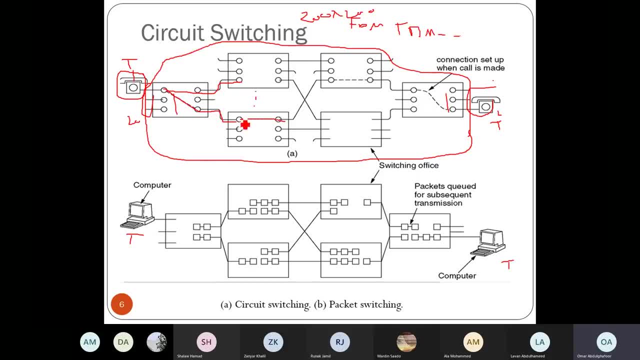 All right, It's not necessary to follow this one. You can follow this one. You can go to this one, Connect here and connect here. Connect and directly go to this terminal. All right, So it depends on the availability of the switches. 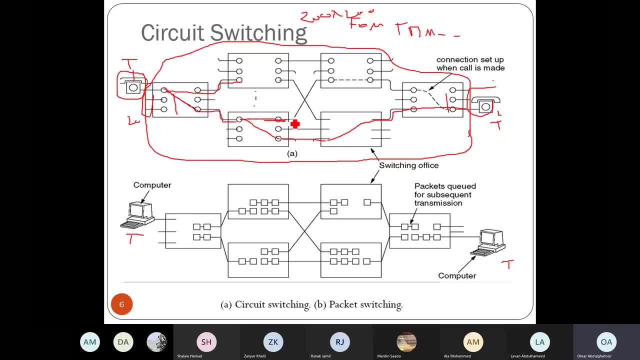 So I'm following this All right From here. I go to another. So I go to another stage and connect switches. connect to the last stage, all right, or the output stage then goes to the required terminal, All right. 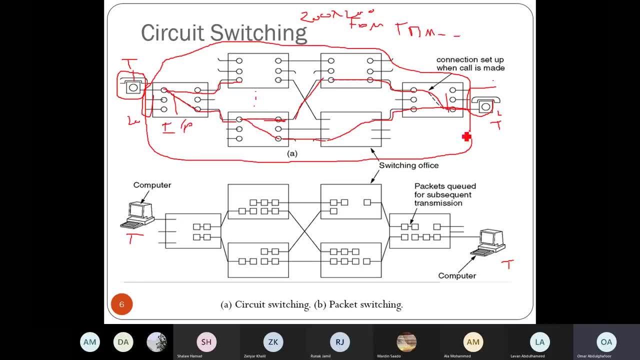 So this is the input stage and this is the output stage, And in between we have some stages. All right, We have some stages. We're going to design. We're going to design similar to this figure, based on some techniques that we have. 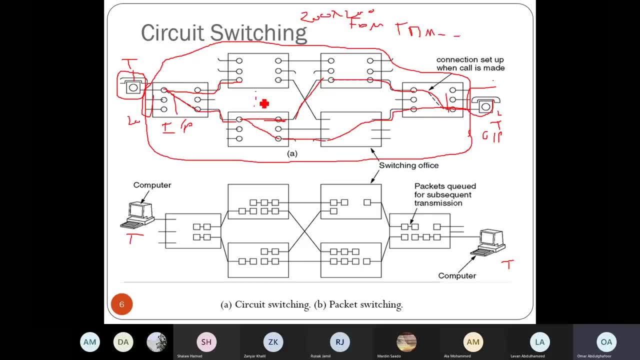 And also, as I mentioned, we're going to calculate the computational complexity and also we redesign to have a better, what we call it switching circuits with little blocking. All right, With little blocking. So this is actually interesting. So, in terms of circuit switching, 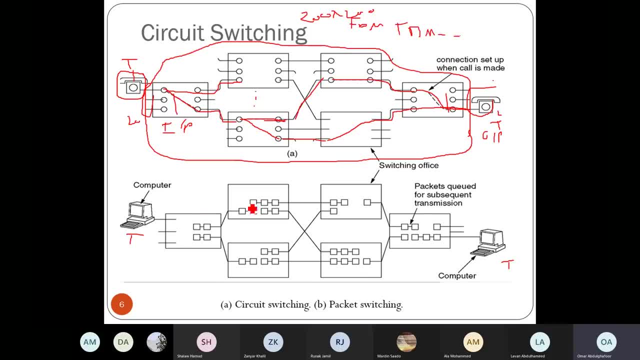 In terms of packet switching, you can see the data actually is divided into packets And it's not necessary to follow the same path. Here is same. All right, I cannot send some data in this path and the remaining in another path. No, 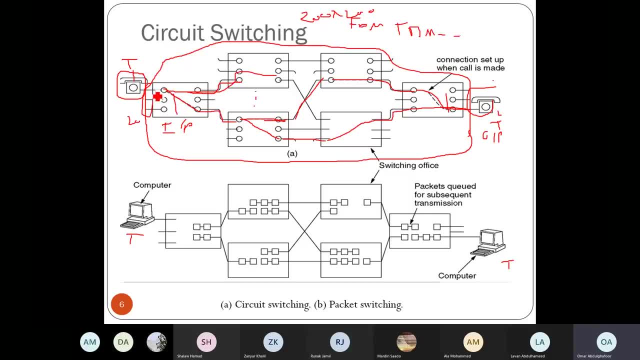 This one, the established, All right, And after that the data transfer will follow the established line between input and output. And after that, once done, Then the circuit will be disconnected. But in the interesting point in packet switching, in this one, that the data actually divided into packets. 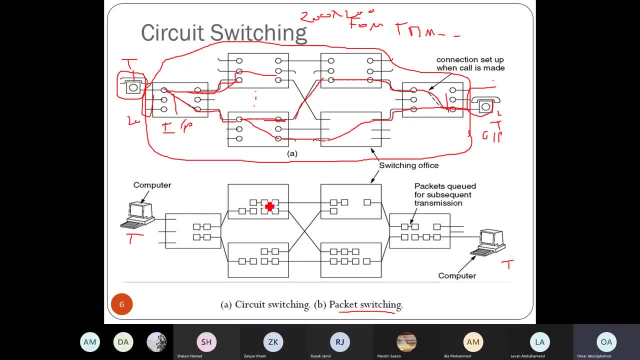 All right, Divided into packets, And these packets will travel using different paths. All right, Different paths. And at the terminal, All right, At the terminal, all the paths recombine again. All right, It's not necessary. For example, I send packets. 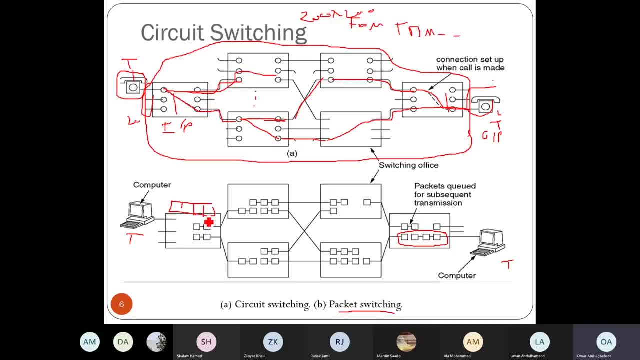 This one, let's say one, two, three and four. This is my own sequence, All right, So here it's my recombine: three, four, one and two. Okay, So here after that, we have what we call the error corrections and the traffic and some technique in order to rearrange and reordering the packets. 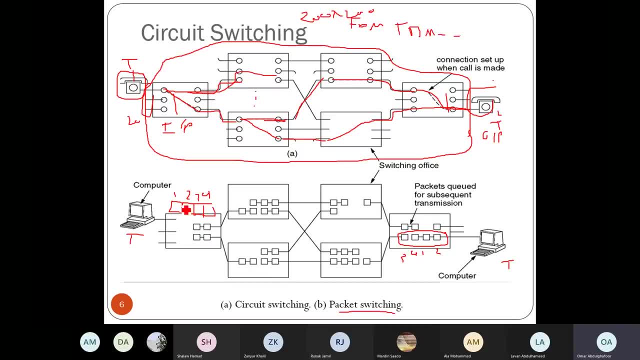 But the main concern about this one, Or the main concept about the packet switching, that the data going to divide it into small, small packets And, for sure, if I divide it into small, small packet, the processing time will be high compared to circuit switching. 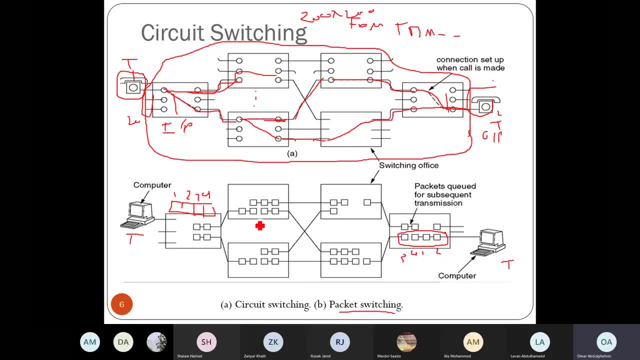 So this one will be faster in terms of processing compared to circuit switching, And the packets will follow different paths between the two terminals: terminal sender or receiver, or two nodes. Okay, And this is the main differences between the two types of switching. 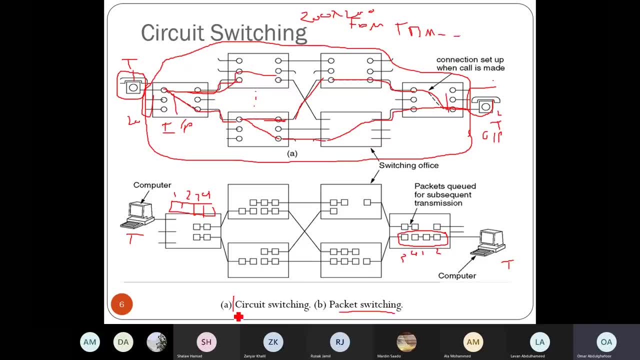 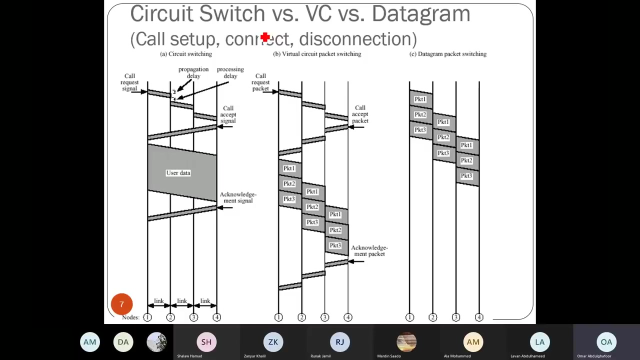 Two types of switching, Because we said the switching can be divided into two broad techniques: circuit switching and packet switching. All right, All right. So this is the like comparison between circuit switch- virtual circuit- all right, virtual circuit. and a datagram- all right, datagram, packet switching. 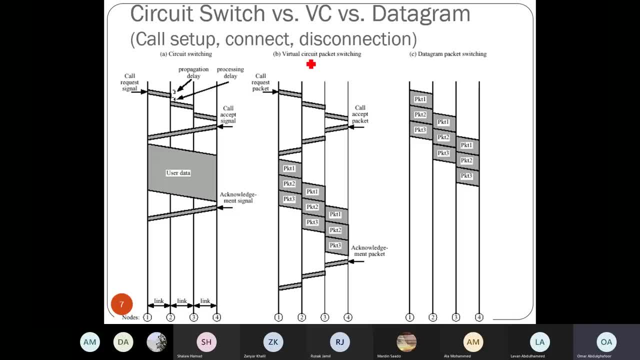 And this one virtual circuit packet switching. If you remember, we said That we have circuit switching And in packet switching we have can be divided into two. if you remember, virtual circuit packet switching, That means it's a mixed concept of packet and circuit. 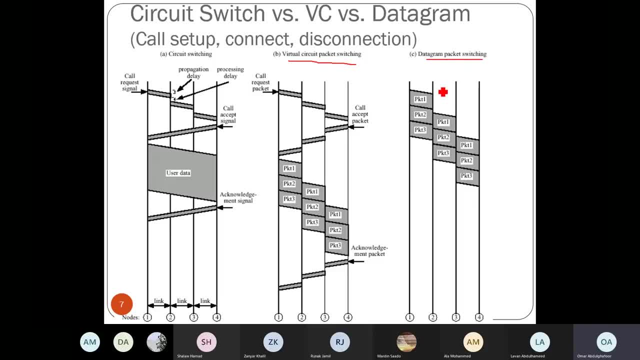 And we have datagram packet switching, which is a pure packet switching techniques. Okay, So this one actually will be in, Not in this, not in this chapter. This one and this one, Because this one actually B and C. it's related to packet. 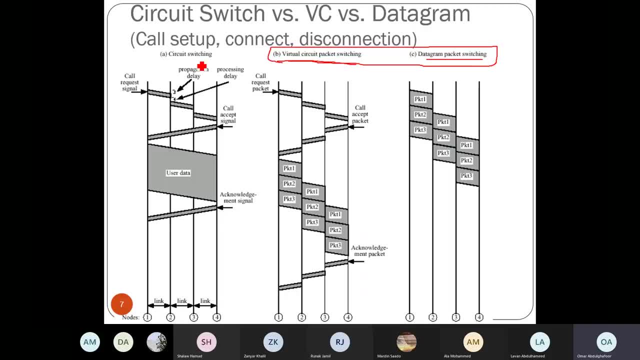 All right, This one is related to packet switching And this one here is related to What we call it the circuit switching technique. All right, So in terms of call setup, connect and disconnect, you can. you can see the difference. 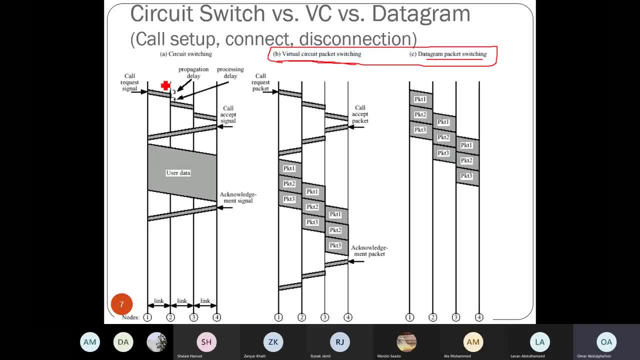 All right, From the figures, for example here In terms of, in terms of circuits, then call request signal. all right To establish this one, all here. we have a propagation delay, We have processing delay. This one call accept signal would be sent. 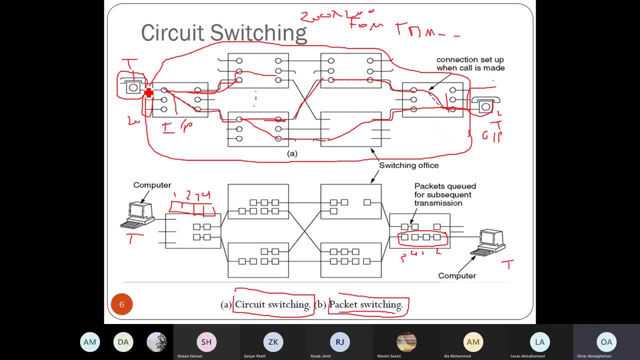 So that means the the link is established, This one when when this one tried to connect with this one. then we have call request signal. Call request signal to the. here we saw that we call it exchange office Or or switching office. 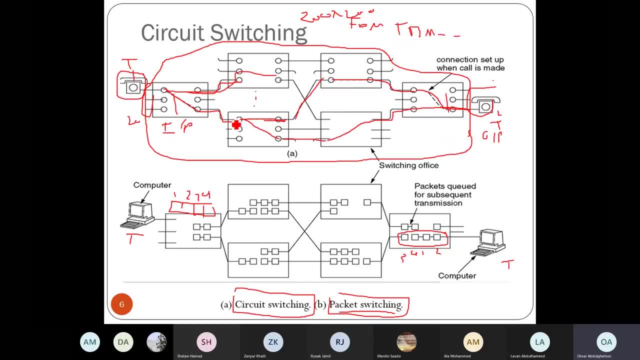 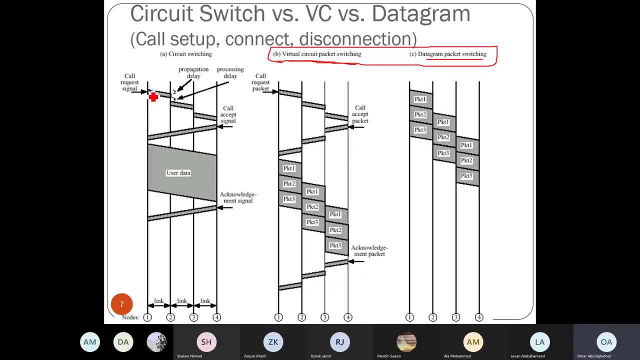 Okay, Then after that call, accept once this terminal actually is available, not on call or all the switches are. some of the switches are available, All right, Then this one will be accept and send back. All right, Then after that the data will be move. 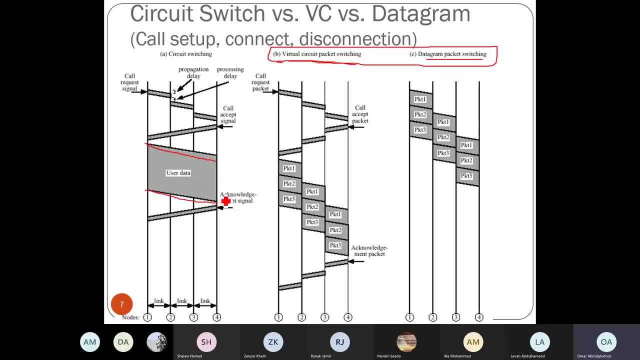 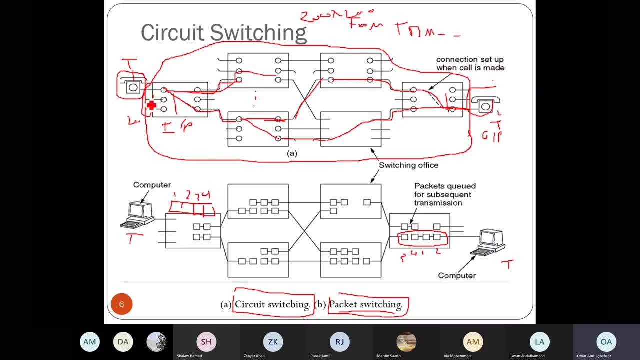 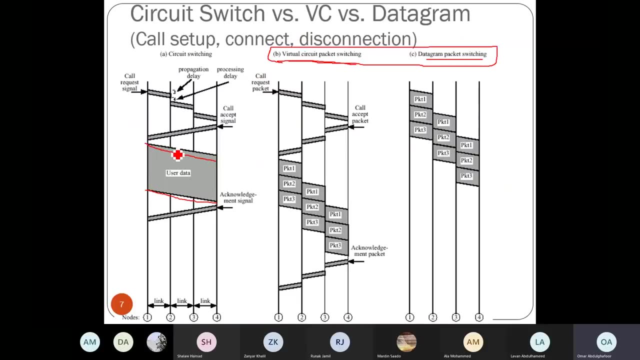 Data will be move And once the data is, For example, there is a, this actually is really details, details, the mechanisms, how the how the data move from this one to that one, So this one actually, if we would like to go, it's really details. 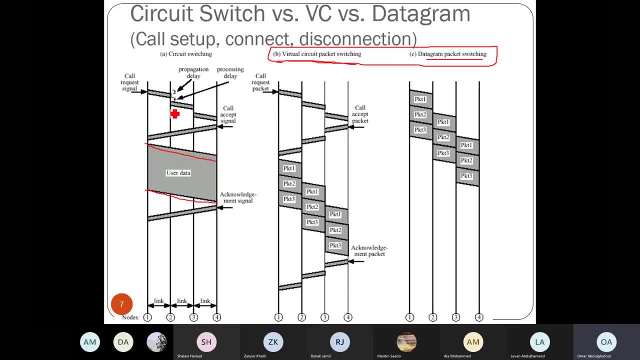 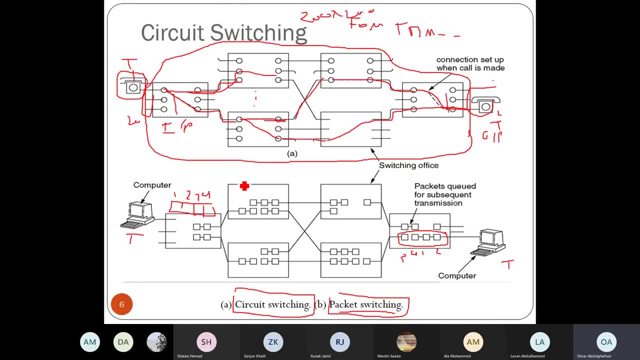 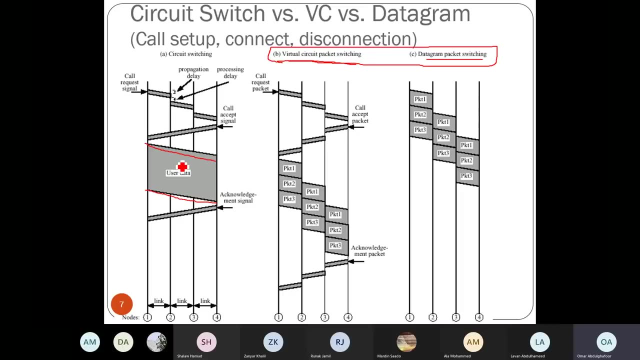 We need another, another chapters. All right, Because circuit switching, we have the concepts which I'm going to explain in this chapter And we have some mechanisms and procedures which need, For example, another chapters that are related to traffic management, congestion control and error correction, detections, et cetera. 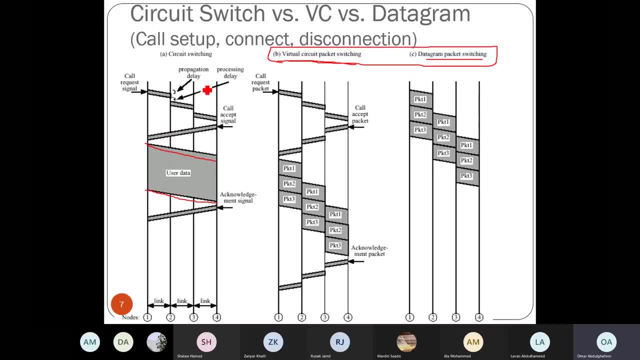 So this is the way that call set up, connect and disconnect. So let's see, compared to this one: Okay, Uh, you can see virtual circuits, virtual circuits, packet switching. Okay, This one call accept, uh, send request. 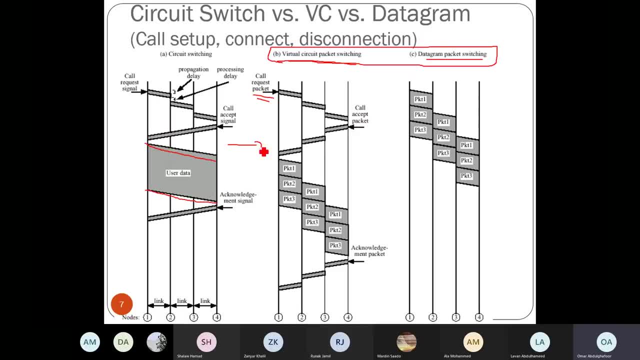 All right, And this one call accept, Uh packets. You can see, here is a signal, All right, Here is a signal, Here is a packet, All right. And after that the data gonna send in terms of, in terms of packet, and acknowledgement also in terms of packet. 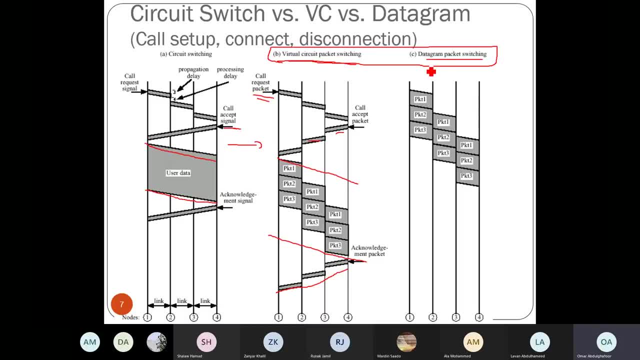 In datagram. this one we call it connectionless. If you remember last chapter- we call it connectionless technique. When I said connectionless, that mean it's equal to this one datagram packet. So that means there is. there is no. 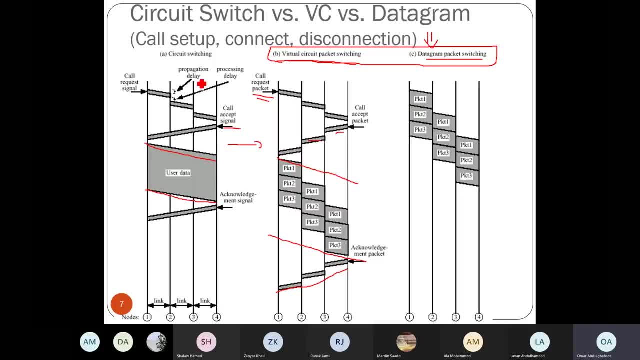 I mean um uh connection. There is no link- Actually there's no, but is available between terminal and uh sender and receiver, This one on demand. If I would like to communicate, then I immediately send packets on the network. 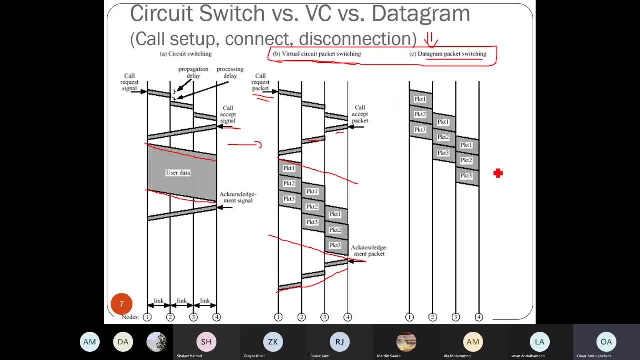 If there's both available, then my packets will will will I mean gonna deliver to terminal. So this one, for example, terminal and this one is terminal. So you can see, in terms of processing, it's obviously this one actually is uh. 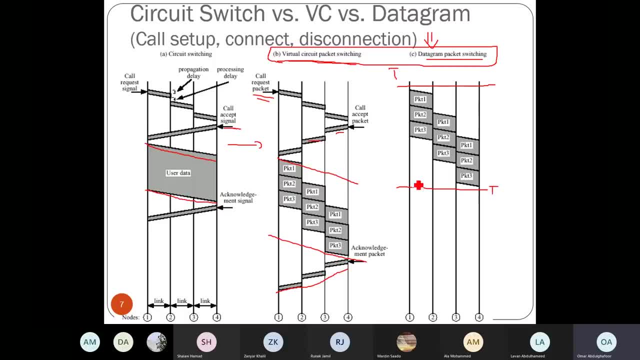 is the best, all right, this one actually is the best compared to compared to this one and also compared to the this one. there is no propagation delay, There's no processing delay, all right, like in the circuit switching. And also there is no some uh request and accept and acknowledgement. 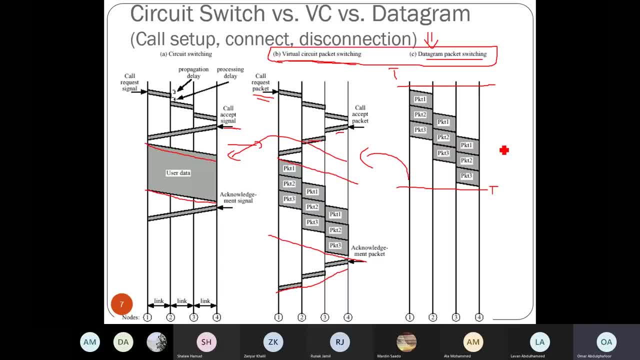 I have a packet. I can send it straight forward. So all of these actually will uh again, if I would like to go in details for this one, then, Uh, we will. um, we'll draw a timing. uh, like this one: timelines. 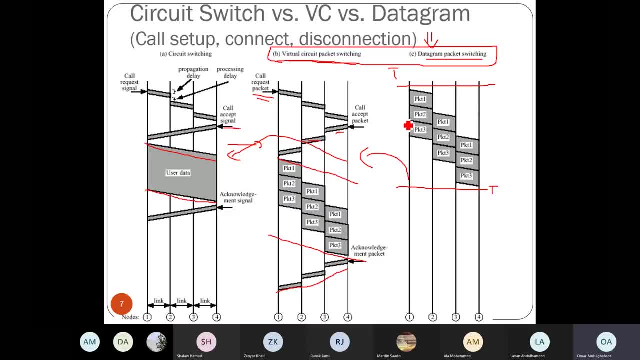 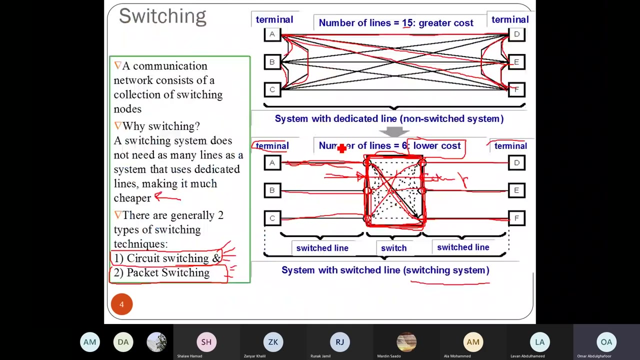 And uh, for example, I can give you a scenario and you can trace, for example, what happened and how many packets we have And the time, for example this one, how much time is required. So this one actually is related, for example, to traffic, traffic management and, uh uh, error correction and detection, like here: 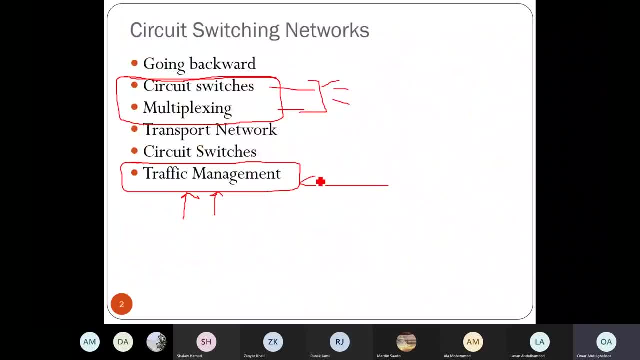 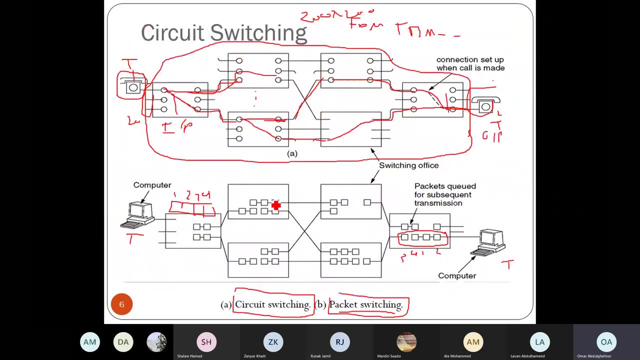 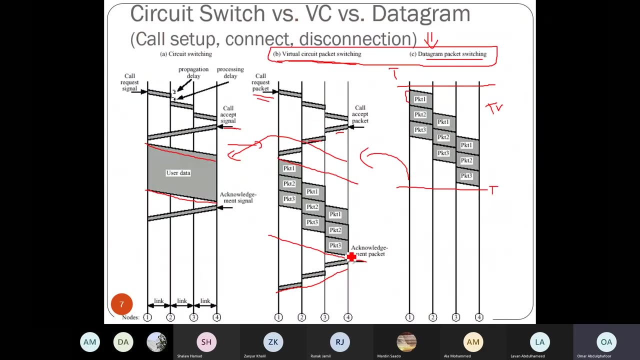 And the one that I this one all right. in in this technique, uh, we can study all that um mechanisms and procedures. All right, Mechanisms and and the procedures. So these are the main techniques. So in in this chapter, again, we are here, but in coming chapter we will study, I mean, the virtual packet switching and the datagram packet switching. 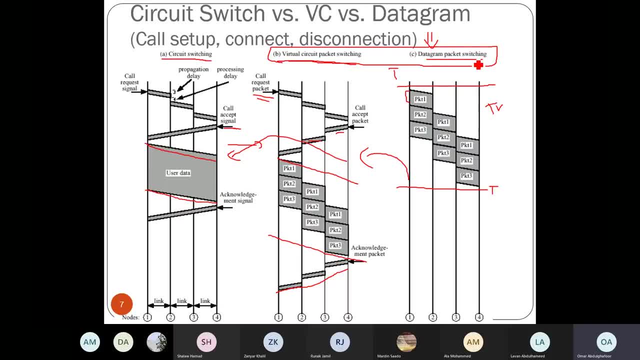 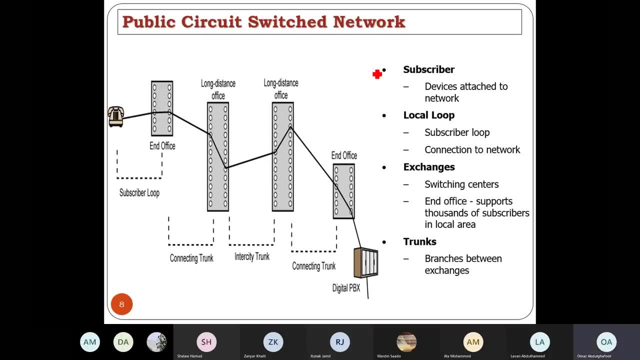 All right, Uh, virtual and and uh datagram. All right, So this is also the shows, the general um procedures, mechanisms. All right, So we have subscriber is a device attached to to network, So we are all, for example, using mobile. 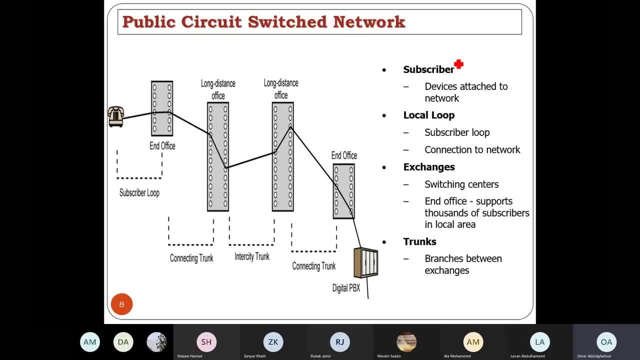 So we are referred to subscribers. All right. So even in mobile communication and mobile um well communication, we are subscribers. All right, So subscribers- device attached to network. So, for example, this one is a subscriber. or if we are using a wireless, we are also a subscriber. 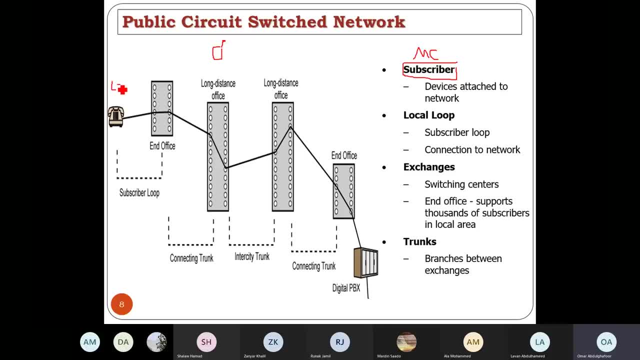 All right. So this one we call it telephone or landline- All right, Landline, Um. and this one called mobile station or mobile device or subscriber, So it depends actually. So a local loop. We said that this one is a connection between, between the, the device, that subscriber, and the end office, um connection. 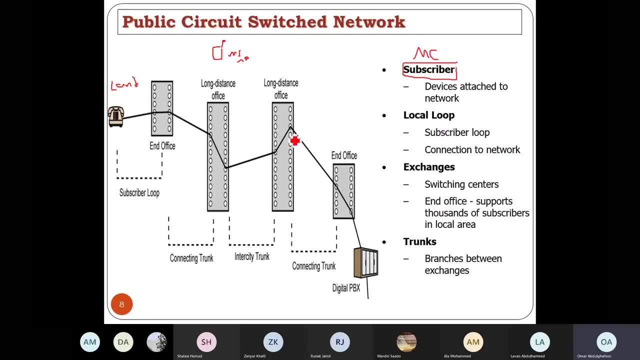 Yeah, Subscriber, subscriber, loop or connection to, to network And in between you have exchange, uh, we have exchange. All right, We have, we call it the exchange, uh uh office, or switching center, or switching office, the office that, uh, we have all the switches in the inside and in the central um units that take care about the establishment of a path between two, uh, between two terminals. 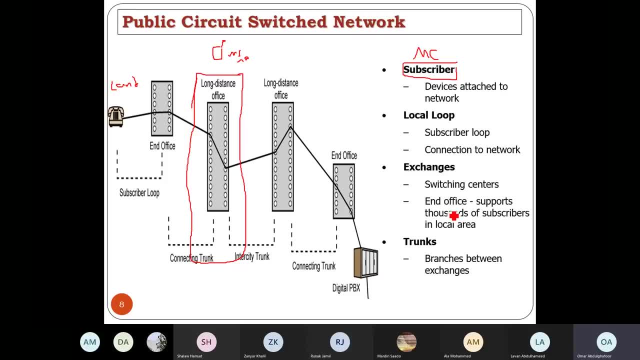 All right And uh, switching center and office support thousands of subscribers in a local area and if we have again, if we have, this terminal would like to communicate with another terminal. they are, and not in the same area, for example, different region then, from center to center, all right, from center to center and after that. 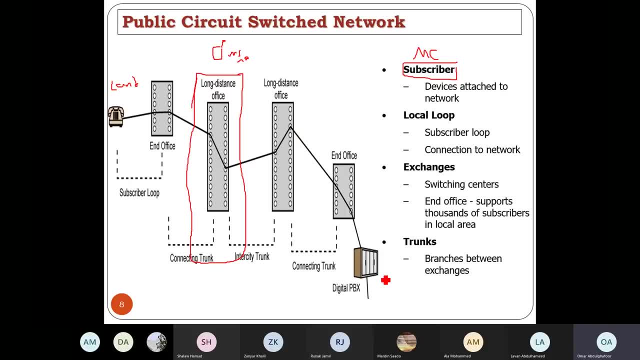 once we reach and office and from end office to another terminal- alright, this one, if we'd like to compare it with- who is wireless, the procedure will be almost same. for example, if we have a mobile alright, the one that I would like, the idea that I would like to highlight it, that the procedures is almost similar. 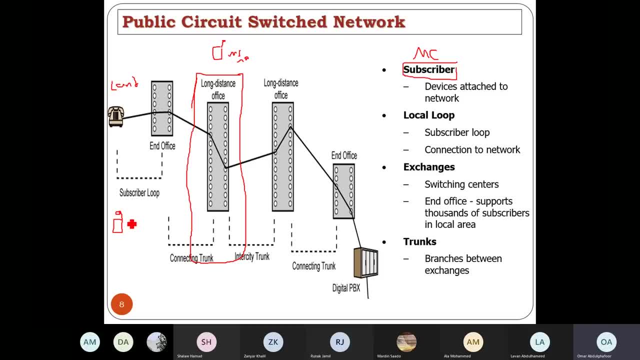 alright, but we have here wireless. so if, if mobile would like to communicate with anyone mobile, okay. for example, you would like to call your friend and your friend in in Erbil and you are in in the Hawk, so you will send your message to your own base station. all right, and base station will forward it to one office. we call it. 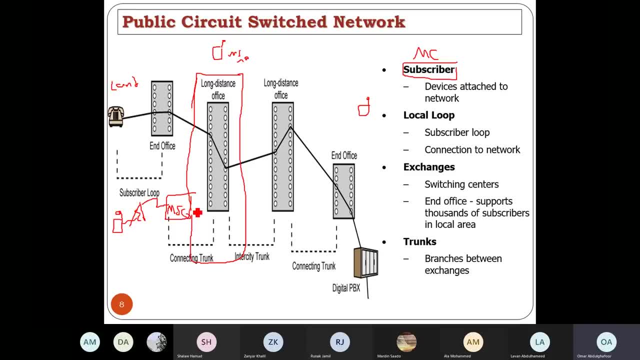 mobile switching center and this mobile switching center will take care about all the base station in the Hawk City. this one- we have some huge tower- will forward it to mobile switching center- Erbil site, all right, and from this one, this one will forward it to this base station and the base station will take 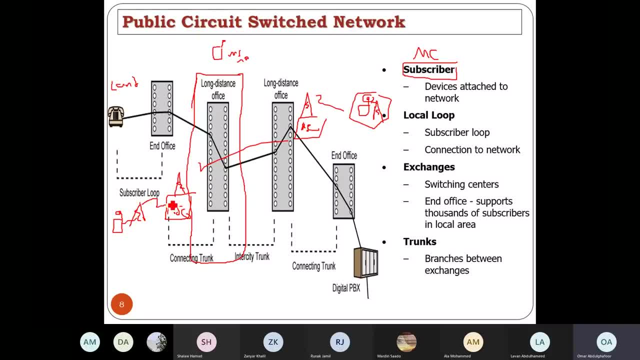 care about this mobile device. so you can see it's almost same. instead of mobile switching center here we have exchange exchanging center. all right, this one exchanging center. so if we have a long distance you can see one center and another Center, for example the Hawk and Erbil. we have one mobile switching Center and 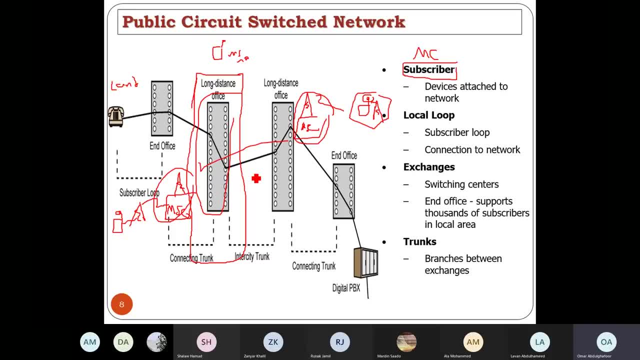 another mobile switching centre. so it's all not same. but in terms of wireless we will gonna discover different terminology and some. the mechanism actually is a little bit different compared to 2n, but generally speaking, general speaking, the component here is, for example: here we can name it as a: 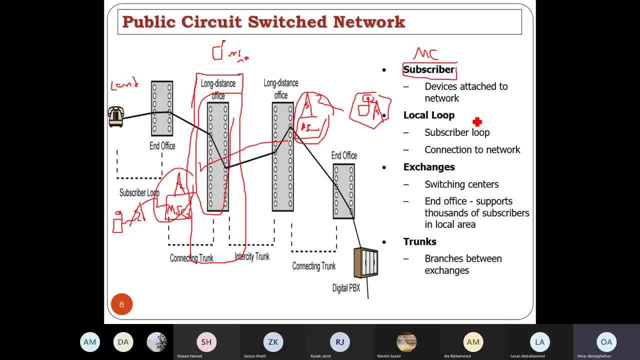 mobile. here we can name it as a, what you call it the air interface, all right, air interface. here we can call it mobile switching center, and here also we can call it the base station, base transceiver station, all right, so the terminology is different and the the way also. 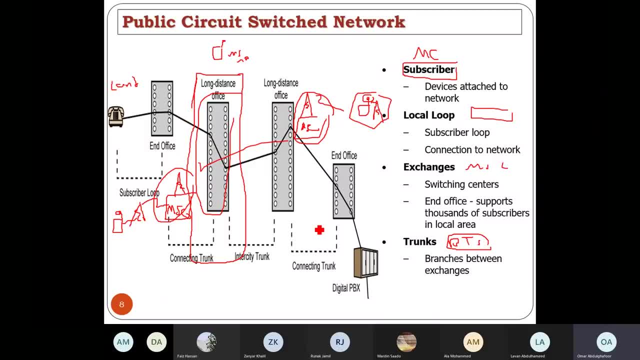 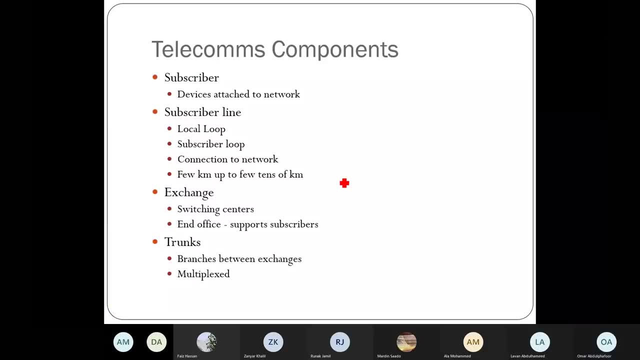 different in terms of wire and wireless, but in general, we can say that similar, similar procedure we're going to follow. all right, so this is the telecoms or telecommunications components: subscribers or subscriber line exchange, or and and trunks, which is the branches between between the exchange. 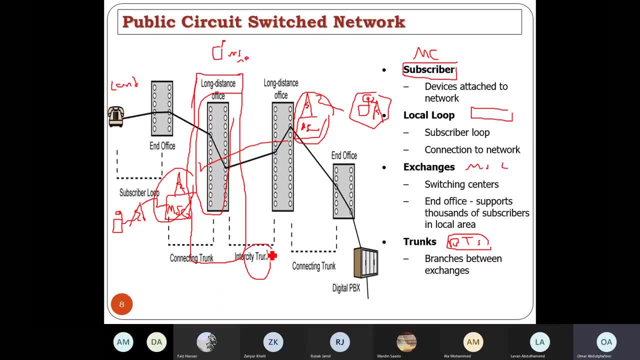 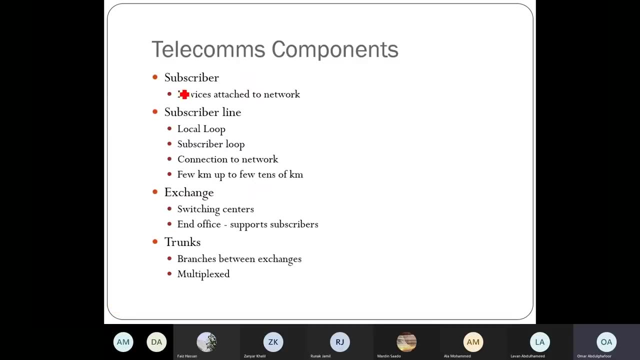 multiplexed this one here, the trunks, all right, which is the branches between between exchanges switching center. all right between this one and this one. so this is the component: subscribers, the subscriber line and exchange switching center, and the trunks, which is the branches between exchange and multiplexed. 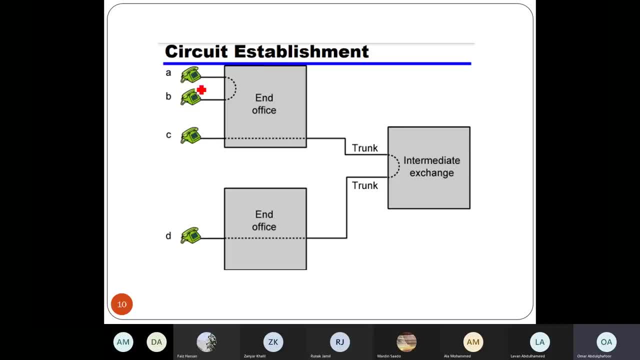 all right. so circuit establishments of this is actually as a an example. for example, if i would like to communicate a with b, which is same, so you can see, only within end office, only within end office, but if i would like to communicate c with d, which is, i mean it's. 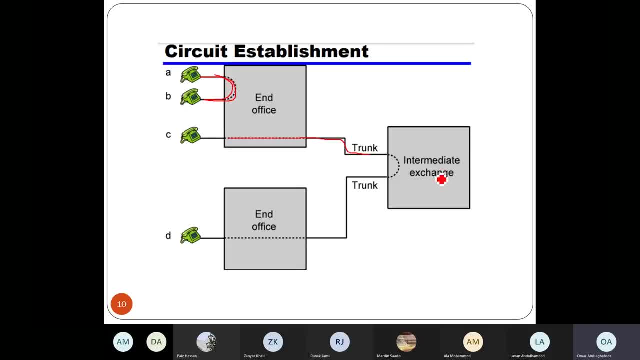 different region, then this one will go to the trunk. all right, intermediate exchange and another trunk then move back to this one. so depending on the ecosystem, here we can say that this we can set actually on the position, depend on the location, depend on the distance that you would like to reach. 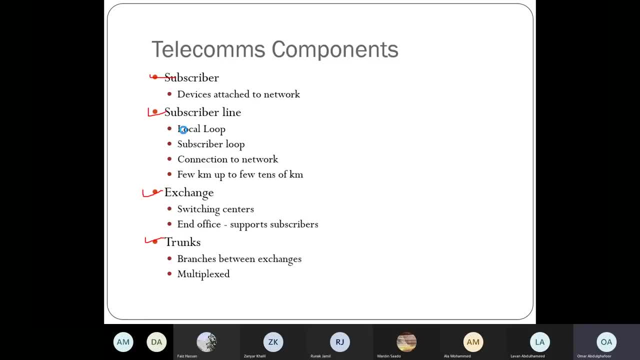 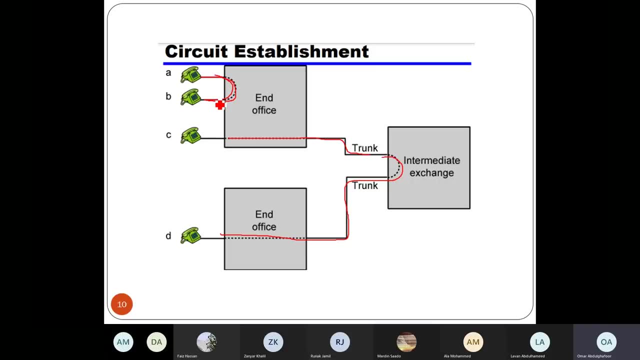 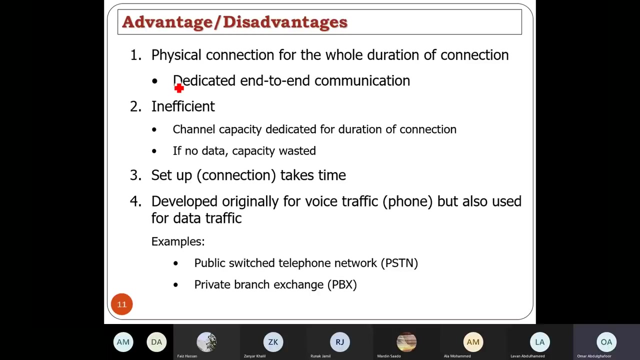 all right, so in wireless also. in wireless also we can draw similar to to this one, but the connections will be between mobiles and base station. if we are far for sure, we need some, some help from the mobile switching center. um, all right, so the advantages and disadvantages um for the uh circuits, uh switching. 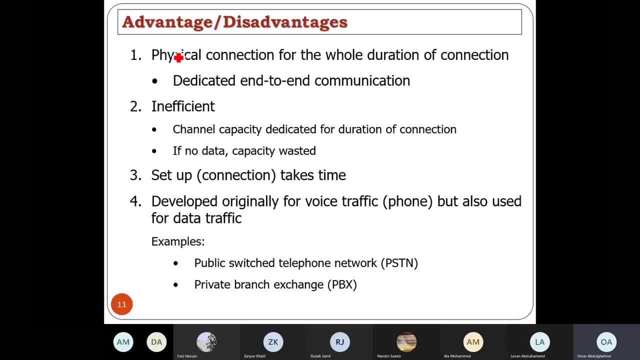 the physical connection for the whole duration of of connection, i mean, once you the the physical path is is established, then that path should be active. uh, all right, so dedicated end-to-end communications, and, um, i mean any when we said this one, for example- that mean any problem in between, uh, the? 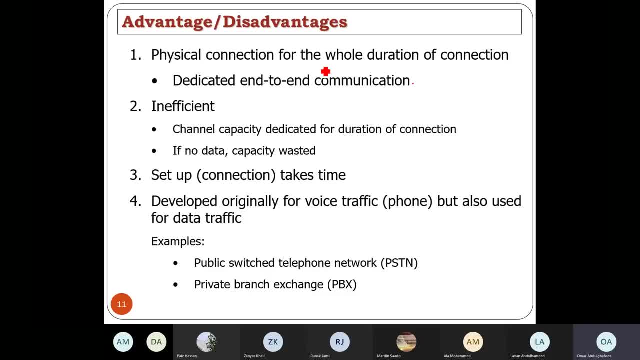 the uh call or the data transfer gonna be terminated, not like a, a wireless, and in a wireless, um, we have one dedicated. yeah, that's right, but if you uh, you are, i mean driving, for example, along the highway, so the connection is still active and you are changing your, your cell, you are changing your, your uh. 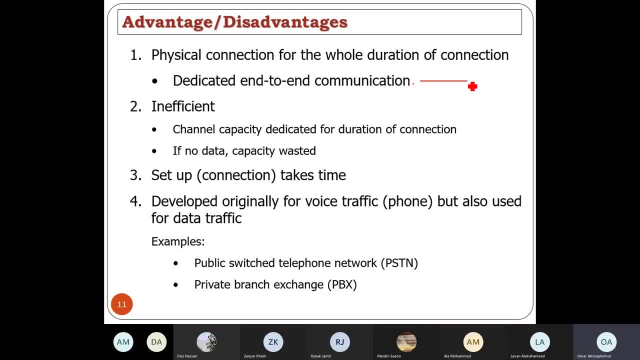 frequency and base station. so the the connection is still still active. so this this features is not available in in in circuit switching techniques. so the path is path. any problem in between you're gonna lost your call or you're gonna loss your data transfer and uh inefficient the channel, uh capacity. 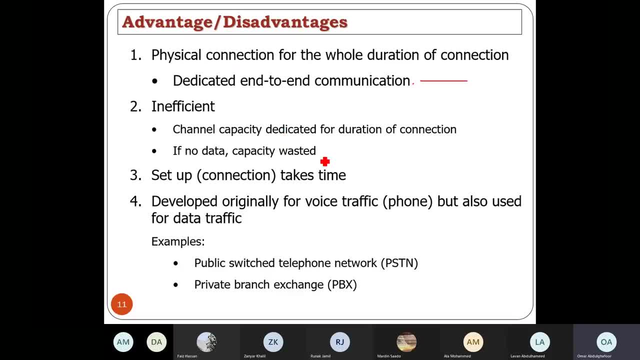 is indicated for a duration of connection. if no data capacity will be wasted, all right. if no data to transmit, then the capacity will be weighted, not like a packet switching on demand. if we have a data, then this one will be active. no data, this one will be remain or return to the available status. 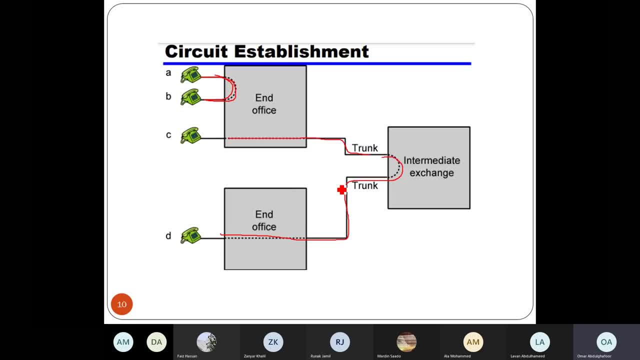 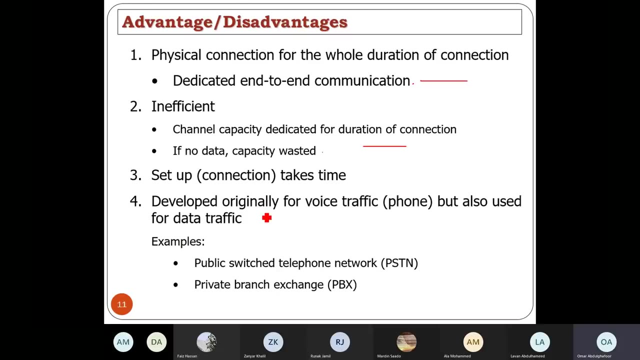 and the setup connection takes time, all right, especially if you have a long distance. this one need a time, all right, in order to set up and checking for the switching. and, um, yeah, this one is for voice but also used for for a data like uh, public switch telephone networks and private branch exchange. 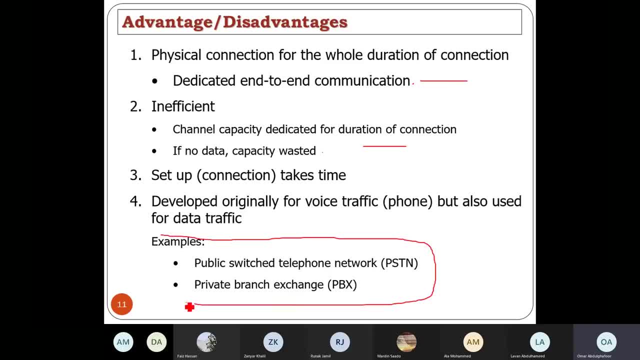 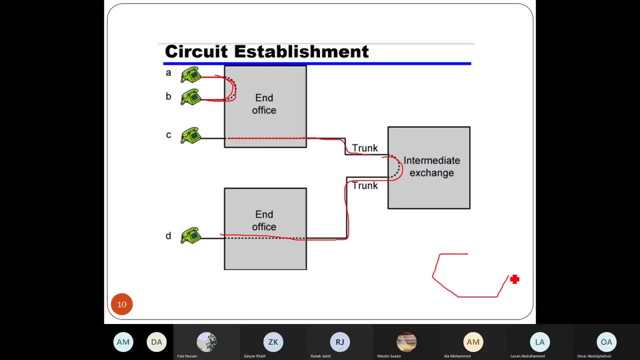 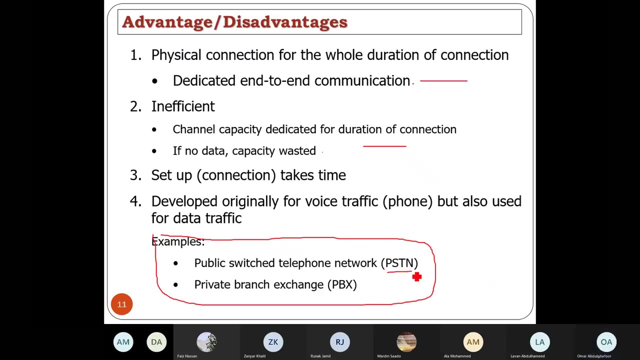 so also can be used for for data and also can be uh, two ways communication. for example, if you would like to communicate, uh, you have a, you have a cell here and you have a mobile and you would like to call this device. all right, so the procedure will be go through this one: pstn. all right, the 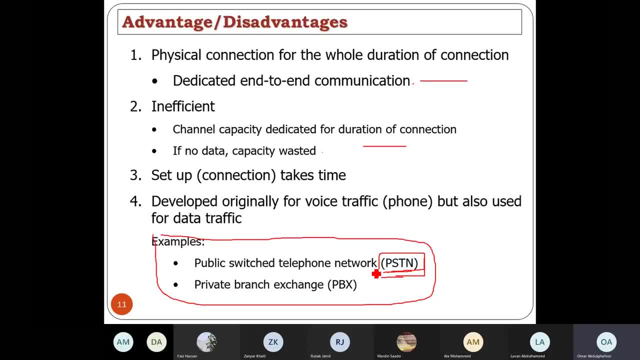 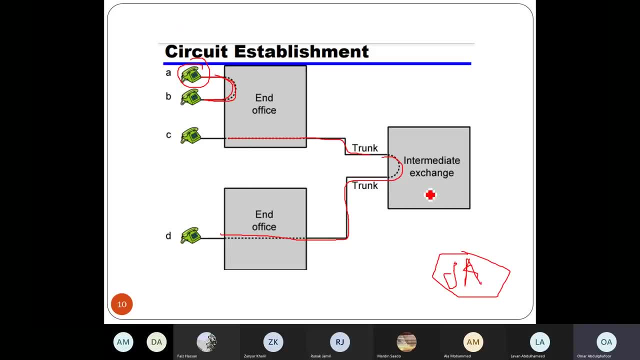 procedure will be by this one, pstn, which is public switch telephone, uh telephone network. this is the main connections between mobile and landline. all right, so this one from mobile will be to mobile switching center and from mobile switching center will go to pstn, pstn and after that you will follow. 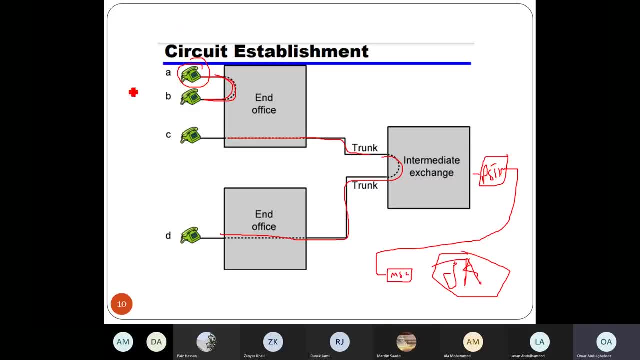 the same procedure, all right. and if you would like to call from landline to mobile, same procedure, pstn to mobile switching center and after that, all right. so, but the complexity actually will be a little bit high because we have different modulation techniques and and will be here and here, so in terms of complexity will be a little bit. 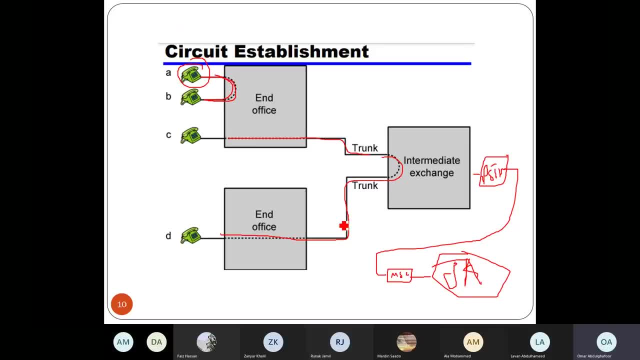 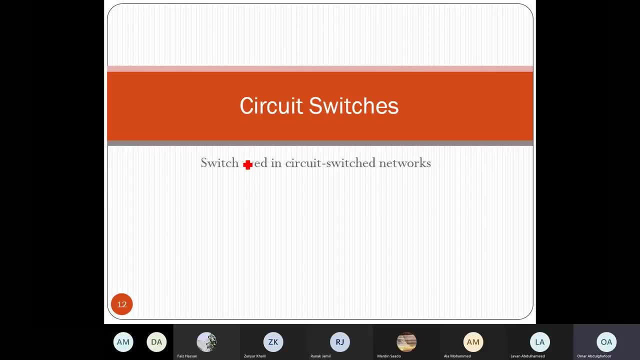 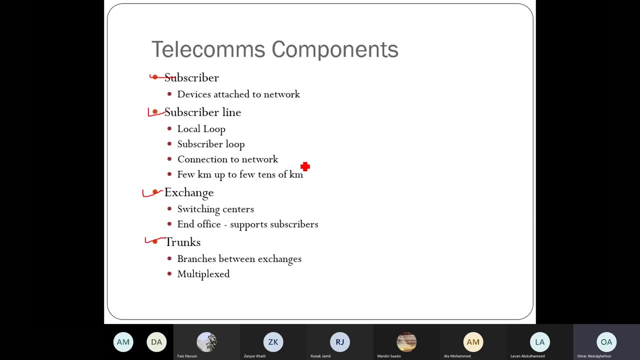 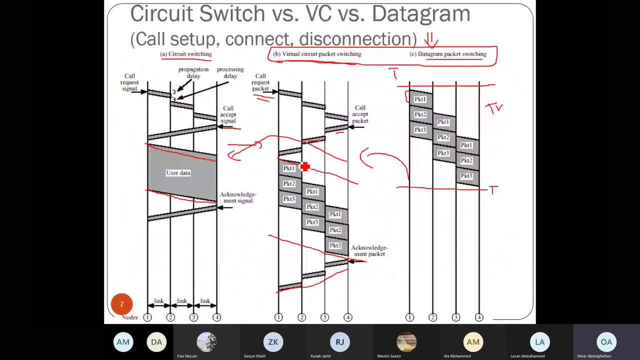 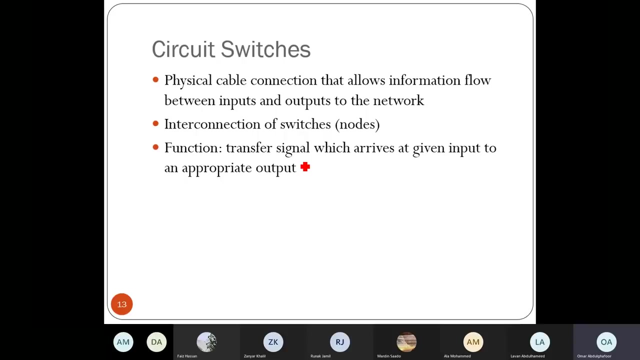 high compared to landline to landline or mobile to mobile. all right, so i mean what we have done previously. it's a brief introduction about the circuit switching. all right, the uh brief idea about the circuit switching and for upcoming, if i'm not mistaken, we're gonna uh try to design. all right, try to. 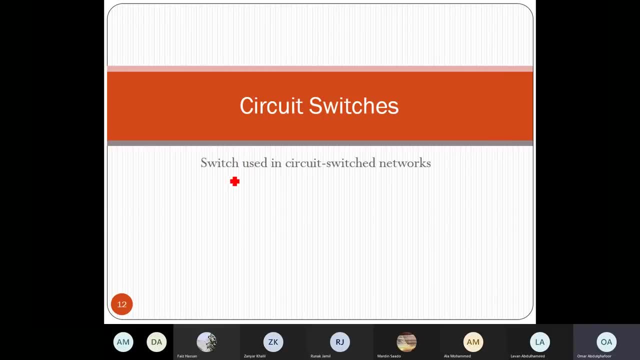 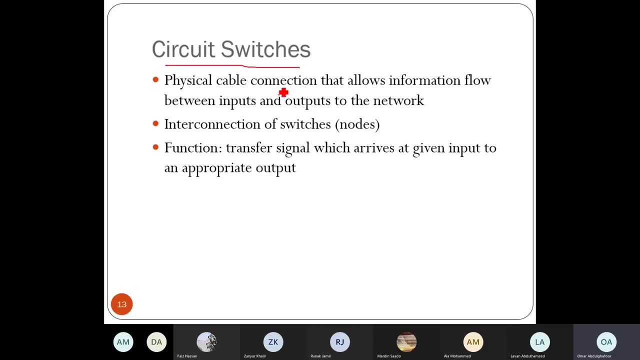 try to design some uh switching network, all right. so again, circuit switches like a physical cable connections that allows information flow between inputs and outputs. all right. so input, which is which is terminal, all right. output, all right. it's a terminal to the network. so we have depend on the number of inputs, depend on. 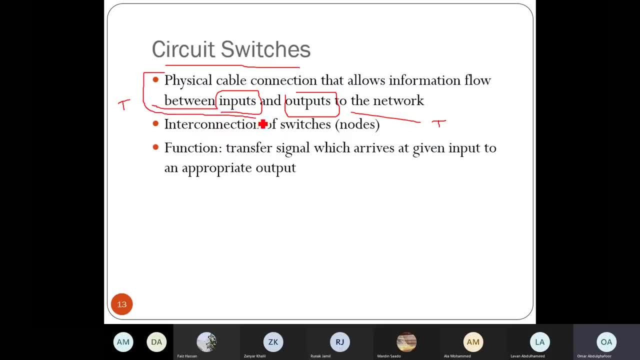 the number of outputs, then the complexity can increase or decrease, all right. so sometimes you have thousand times thousand, all right, and we have, for example, ten times ten. so for sure the complexity, computational complexity, for this one will be really high compared to this one. so if you keep increase on portend outwards, the complexity also gonna increase and it's the 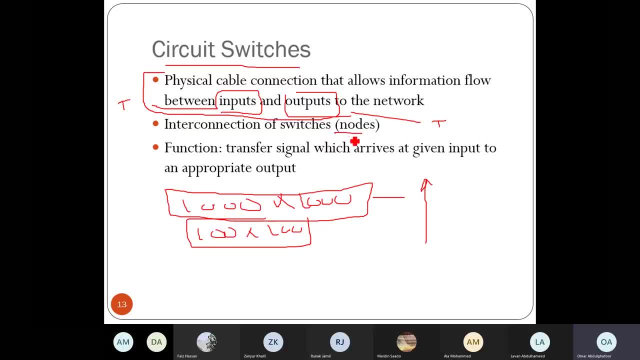 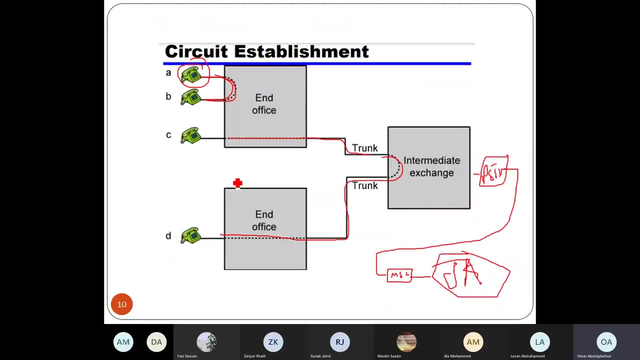 like an interconnection of switches, nodes, and the function is to transfer signal which arrives at a given on port to an appropriate output. all right, similar to what we have showed previously, like this one: the connections of some on ports, connection with some outputs, all right. so, for example, here we have one, two, three, also here we can have one. 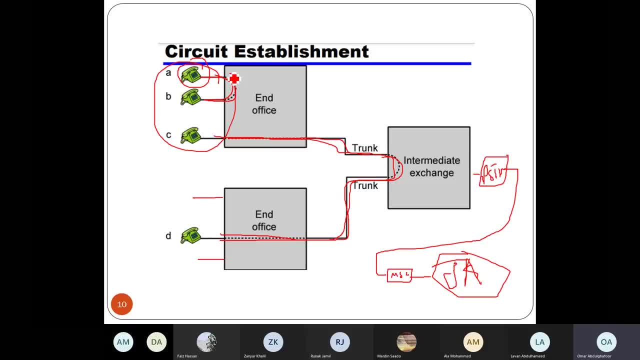 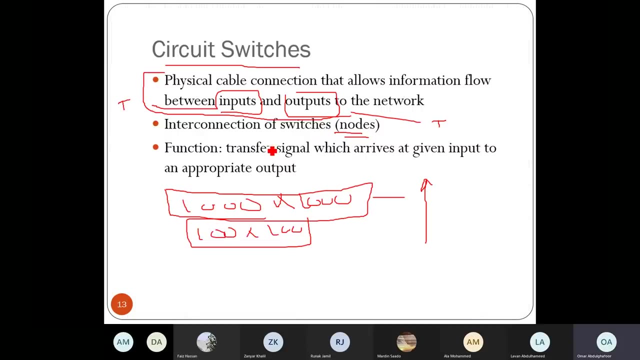 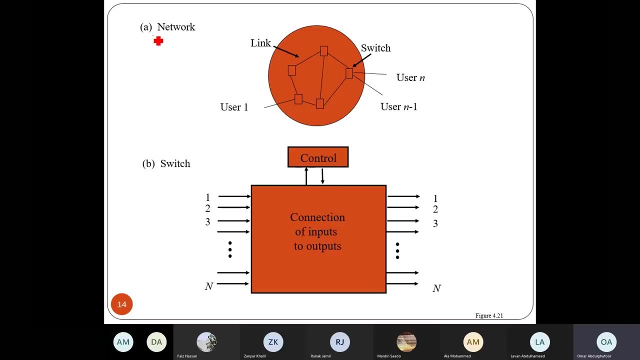 two, three. so we can assume this one is there like an, an output, and this one like in an output. okay, so, for example, this is the if we have a network and here if we have a switching, all right, switching center. so you can see, for example, here how many nodes, how many nodes we have. 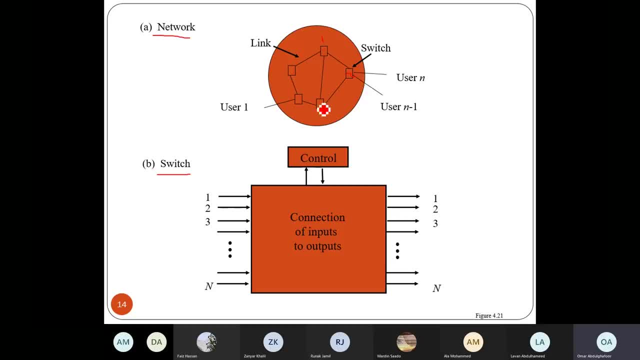 one, two, three, four and five. and in this particular scenario we have one, two, three, four, five and six. so for sure, depend on the, the connection, for example, star, ring, line, drop or whatever topology, but in this particular scenario we have the users n minus one. the n actually is a link. so we have one, two, three, four, five and six. 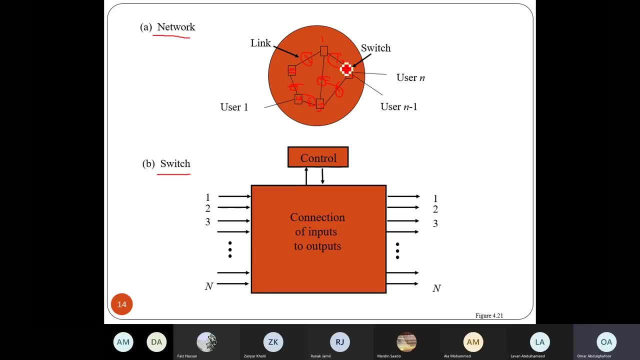 and we have five users: one, two, three, four, five. so in terms of of users we can say n minus one. that mean n- here actually is referred to the links- minus one. so we have six minus one will be five. we have five users, n minus we have one, one, two, three, all right, so this, that the way that network connect. this is actually just. 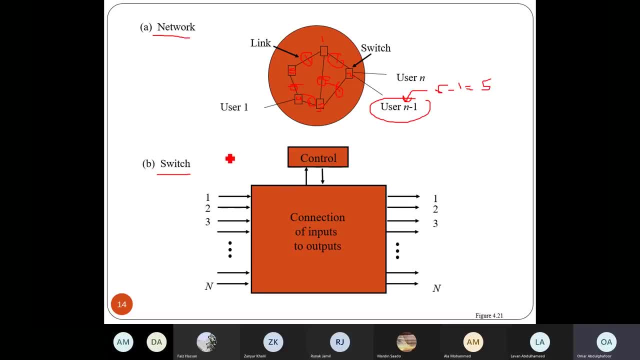 an example, guys, as i mentioned, because it depend on the topologies. we have different, different topologies how the wired networks connects to each to each other, but this is just an example. if we'd такого 've f�må parëét? with the, with the switching techniques, in terms of, in terms of switching, we have・・ all N. 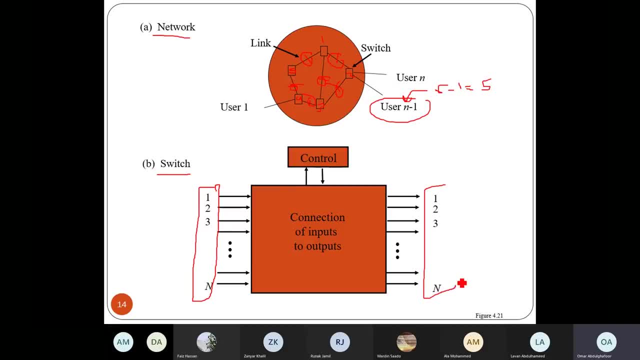 right, we have on put and we have one coach and we have. we all know that the actual performance of this will decrease depending on the whatever responsibilities of our situation. this is VERY, you know, because if you're have output, you can see n times n. all right, so from one, two, three, until we reach to n, it's 150. 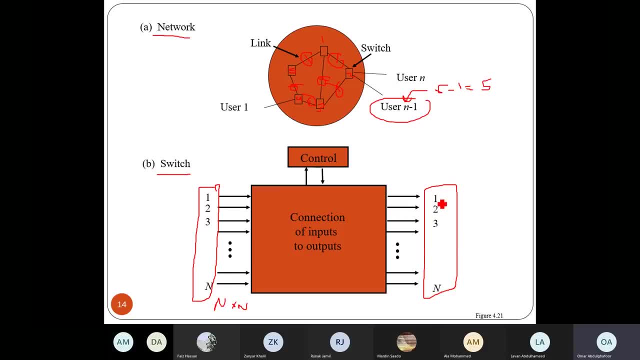 20, 10. it's depend, and this one also one, two, three, so depend on the uh n value that we're going to choose. and this one here is the connection of input and output. so in between, here we have switching. we have switching. for example, if i would like to communicate one with n, then here i have. 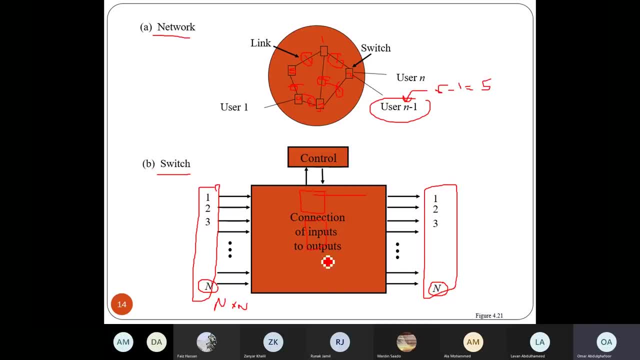 some, some blocks, all right, some blocks, some blocks, okay. and here also i have some, some inputs, some outputs, some inputs here, some outputs. so depend actually on the design procedure. here we have, for example, one, two, uh, and divide by n- we're gonna check it afterward, but i mean we have some. 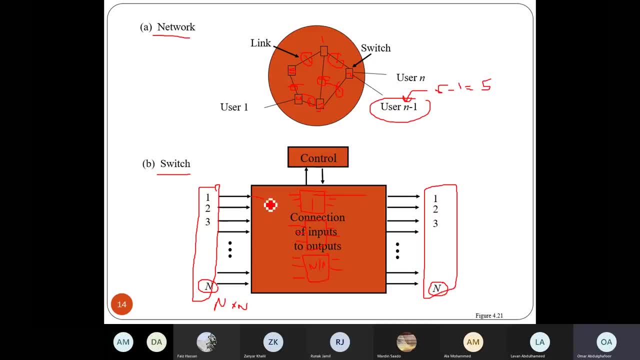 box inside and each box we have some switches. for example, i can my, my, my call establishments can follow this one and from here i can reach to this one, or from i can choose different, different paths and again, this one will be uh automatic, uh establishments by the exchange, uh exchange unit or the switching, uh switching center. 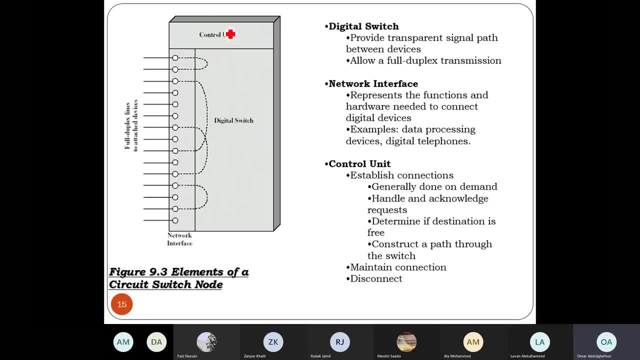 all right. so the the element, actually, we have um three: one, two and three. all right, one, two and three. we have digital switches- this one. we have network interface- this one- and we have control units. all right, three main elements, three main elements. all right. so for the digital uh switches, this one, which is allow full duplex transmission. 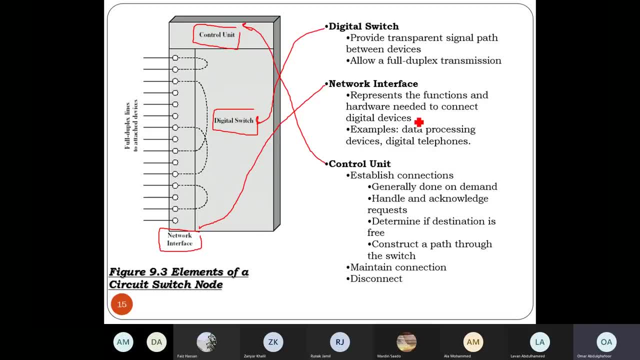 and for the network interface represents the function and hardware needed to connect digital devices, for example the data processing devices, digital telephones, etc. etc. in terms of data processing, um, this one actually, it's um, uh, like signal processing, okay, analog signal processing or digital signal processing. i mean all the processing that related to data in order to provide 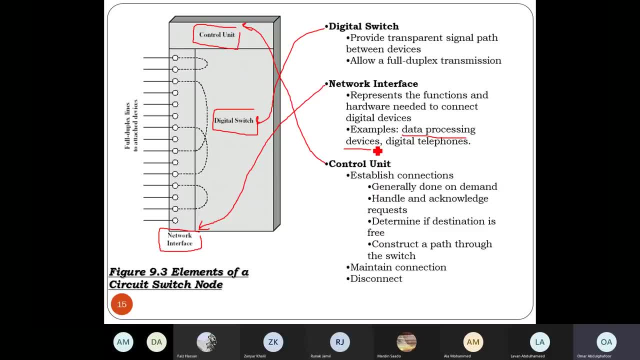 the data in an inappropriate way, remove noise or or provide analyzing. okay, and for control units normally take care about the control process like handle and acknowledgement request, determine if the destination is free and to construct a path through the switches and take connection disconnect. i mean all the control. 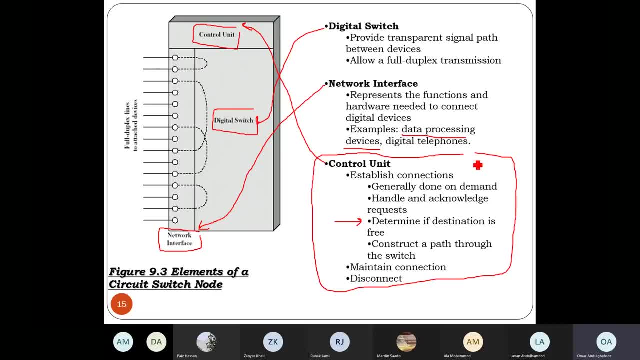 uh procedures, all the control procedures uh will be handled by this one, the control uh, control uh units. all right, so this is actually is the is the heart of the uh circuit switch node, like a, like a microprocessors that's, or microcontroller that can take actions, for uh can provide many 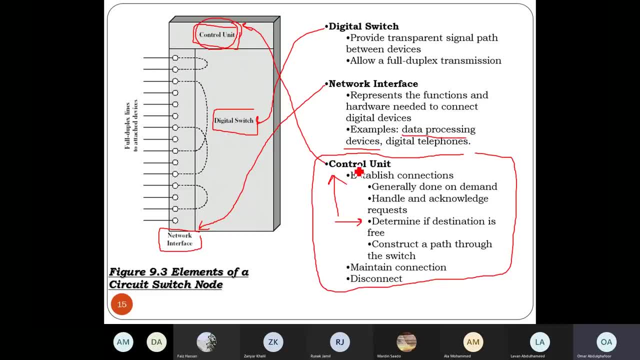 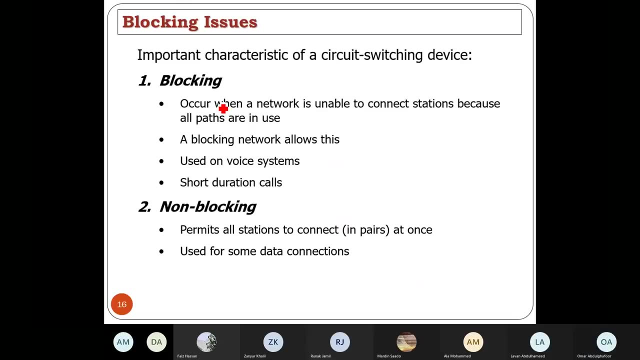 functions all right to some devices. so this one actually will take care about most of the procedures inside the circuit switching all right. so this one actually is very important blocking issues. so important characteristics of circuits switching device. we have low Glasgow In-Way Timothy lebuck. 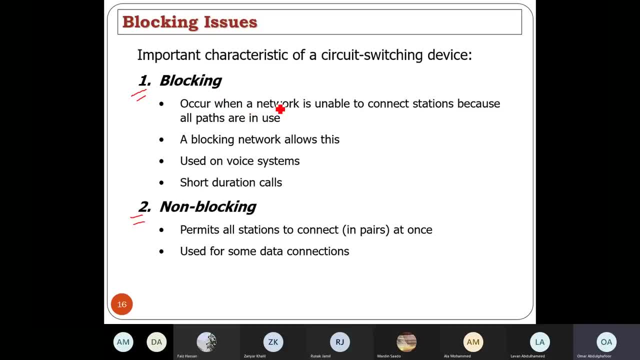 crypto blocking, assistance of blocking. but in terms of circuits, since the, the path actually is established, like by switches, by transistors or by some electronic devices, then we can. we can, let's say, um control this one, the blocking, so this one, the blocking occurs when network is unable to connect stations. 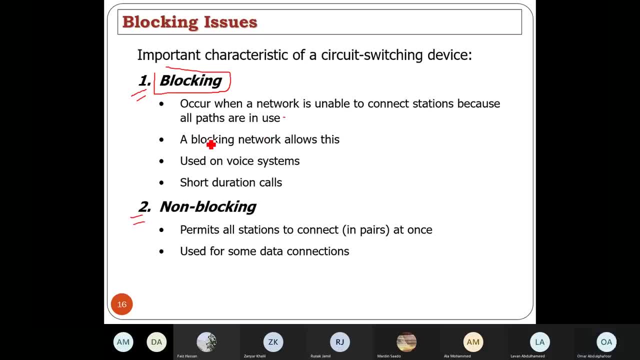 because all paths are are in use and a blocking network allows, uh allow this. that mean there is some probability of blocking, used on voice system and short duration call, but for non-blocking circuit switching permits all station to connect in pairs at once and used for some data connections. all right, so this one- actually that's all connections- will be connected. 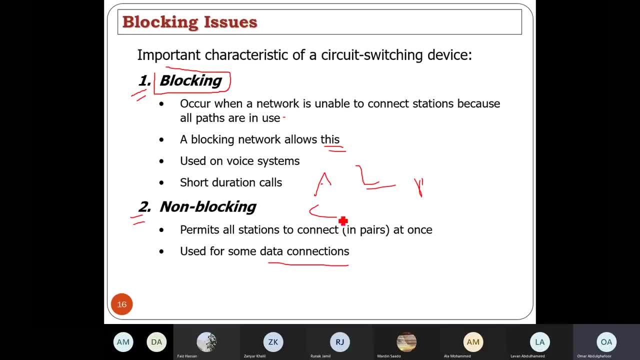 to each other in pairs. for example, a goes to b and c goes to d and all that one, the one that we provided previously, but this one actually will be um, but also that is the one that will be the most likely to be used for the by some type of. 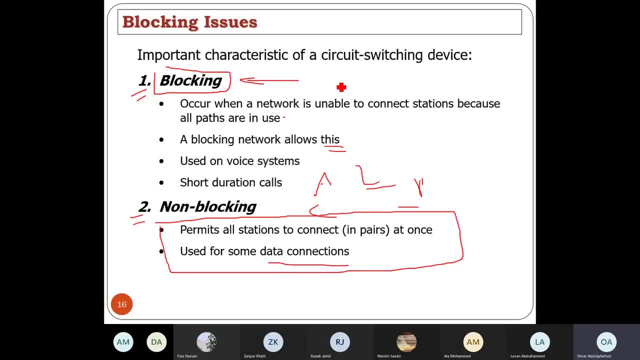 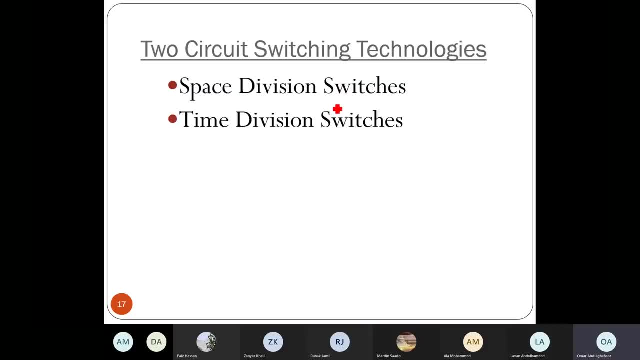 blockage and so in terms of project thickness it will be high, in terms of cost will be high, all right, in terms of cost high. but we'll try to to treat the blocking via some techniques. we will. we will check it, uh, afterward, all right, so i will. i will stop here for for a break. all right, for, let's say, 15 minutes. 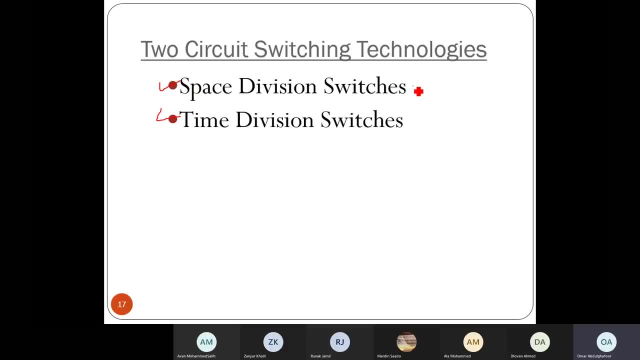 this one, the space division switches and the time division switches. all right, one and two also. we highlighted this one, actually, briefly in previous chapters and today we're going to use it, we're going to try to to design, to design at least this one, the space division switches. all right. 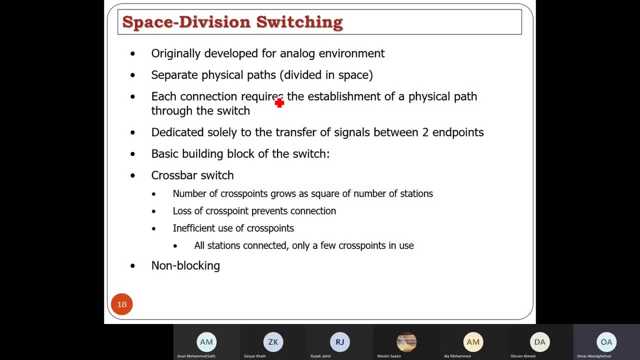 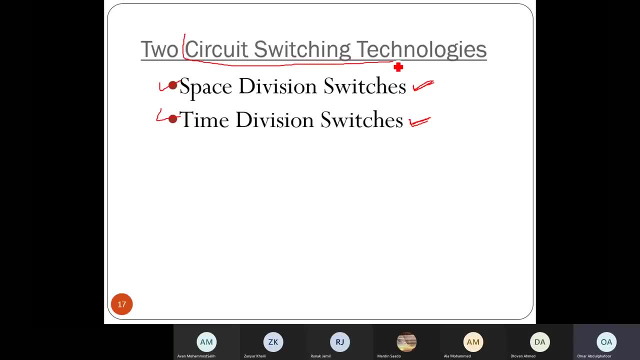 so this is actually the structures, the structures of circuit switching technologies. the structure: we have, yeah, two, two technologies in terms of structure, either this one or or this one. so in in space, this one in the space. the structure: we have two technologies in terms of structure division. uh, switches, uh the path in the circuit are are separated from uh one, uh another spatially. 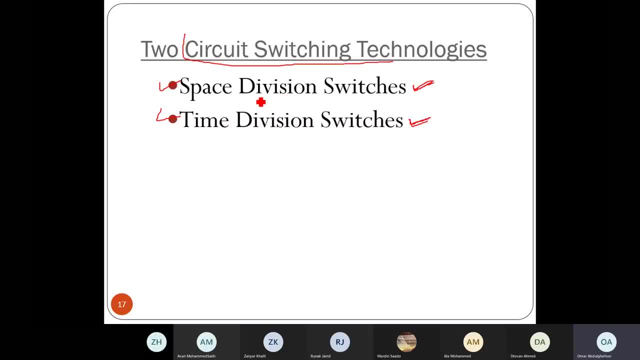 all right. so it's like when you have, when you have, two terminals would like to to communicate, then the path will be gonna established between two terminals exactly. but in terms of time time division, we have some, some flexibility in terms of rearranging, reordering, for example. 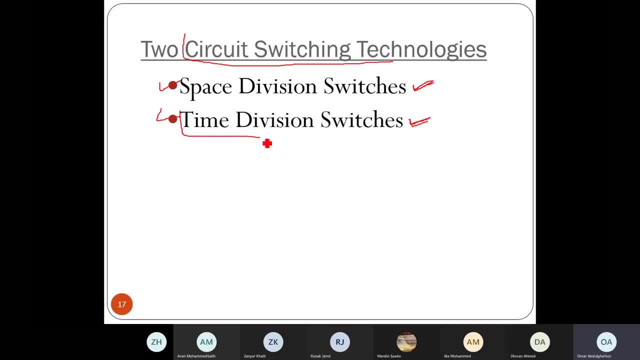 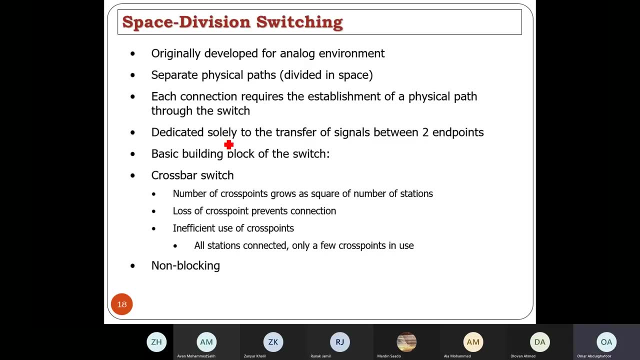 different node would like to communicate with each other. so we have some some flexibility in in the time division. uh switches, all right, so this one, the space division, originally developed for the features for analog environments. so separate physical paths, okay, divided in space, and each connections require the establishment of a physical path. 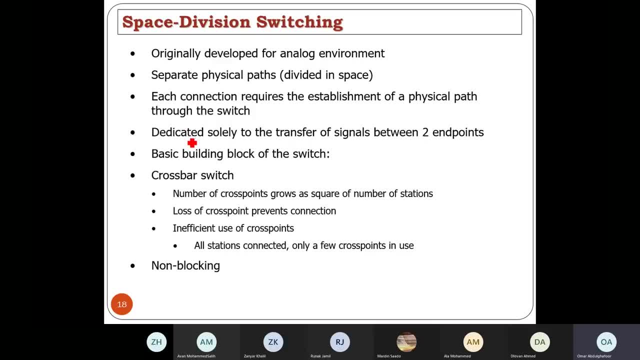 through the switches and dedicated slowly to the transfer of signals between two endpoints and the basic block, our building block of the switch. we have the crossbar crossbar switch. all right, this is the main, the main point. so when we say the crossbar switch, this one connects. 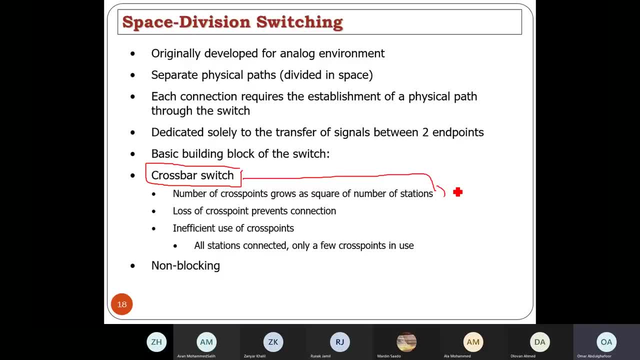 um, this one crossbar switch connects n inputs, all right, to, let's say, m outputs in a grid, in a grid, all right. so this is what you call the crossbar uh uh switcher. so how they can connect this one using, for example, some uh electronic device like transistor. 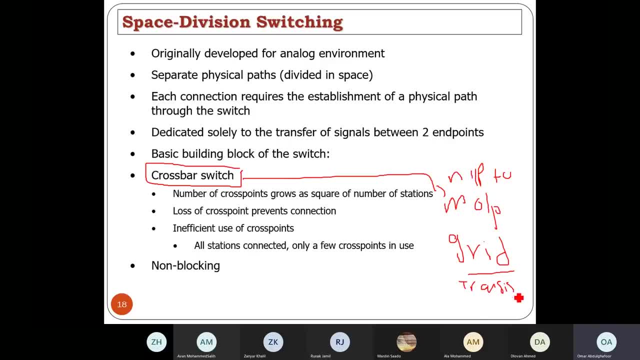 all right, like transistor so they can uh communicate with, uh with each other. so when we said the crossbar switch, that mean the main function. the main features of this one is to connect n input to m output in a grid. all right in a grid. and the way that they can connect this one to this one. 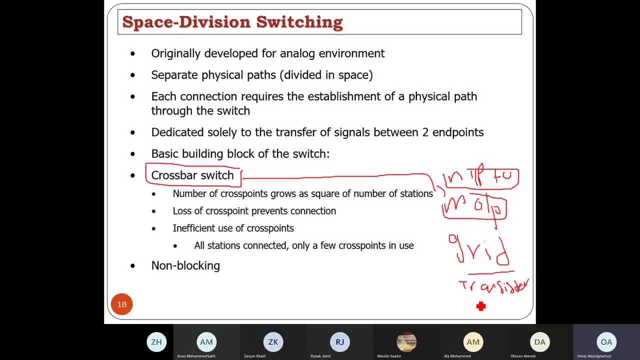 in this unit by using some electronic devices like transistors. all right, and here the uh number of cross points grows as a square of number of stations. this one, actually, in terms of computational complexity- we will highlight it afterward- and the loss of cross point pre-transition. 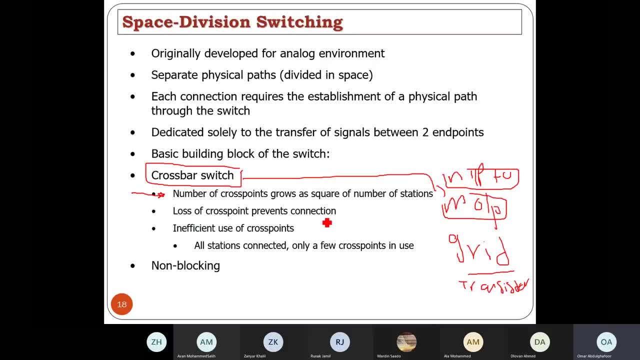 of cross points prevents connections and inefficient use of cross points. all stations connected, only few cross point in use. okay, then we can avoid actually the. the limitation of of, i mean the major limitation of the cross point design, is the number of cross points required. all right, the number of cross points required, the cross point here, for example? let me show you this. 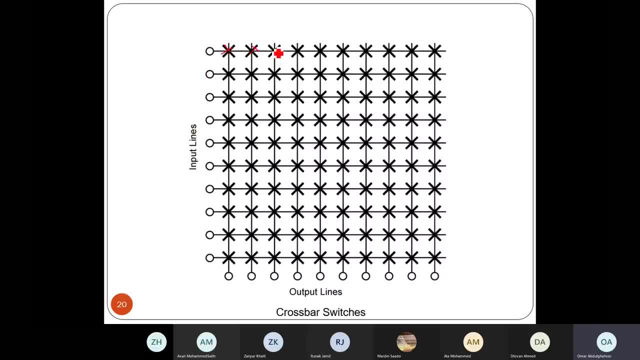 one, the cross parts, which is you can see cross points, cross points, cross points. so that means all the nodes are are connected. if you would like to go for this one to this one, then you will follow, for example, this, this one, and you will connect all the way. all right, so. 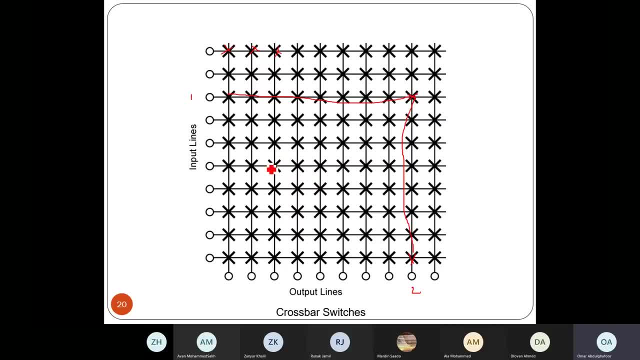 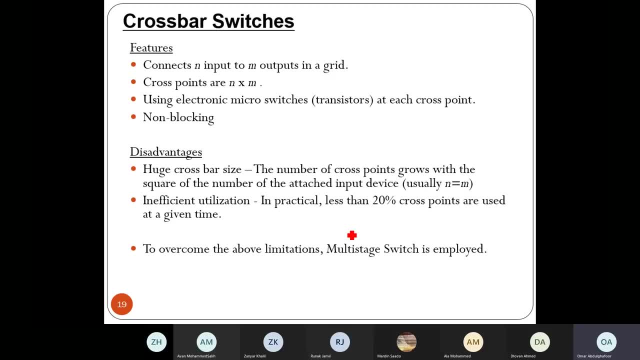 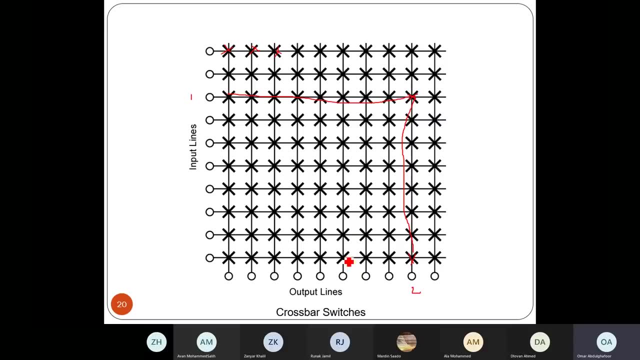 the remaining here. it will be available, okay, and also active. you can, for example, choose different, so it depends. so that's why actually the the main, the major limitation of the of this design is the number of cross points required. this one, the cross point, all right. so in order to connect, for example, n input, this one n, let's say, to m output. 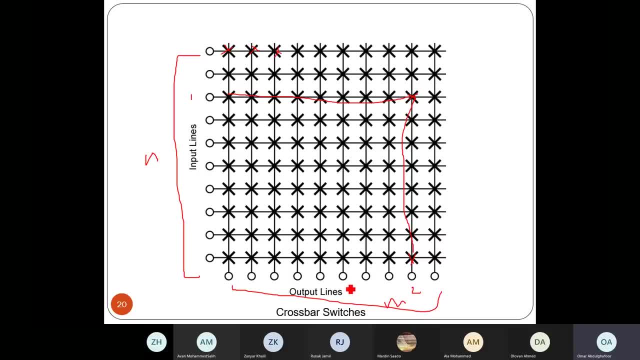 uh, all right, using a cross bar, this one crossbar switch. so we required n times m cross point. this one, all right, n times m cross point. so that means the the computational complexity will be a little bit high. for example, if this one is a thousand, all right, and this one is. and this one is a citizens. 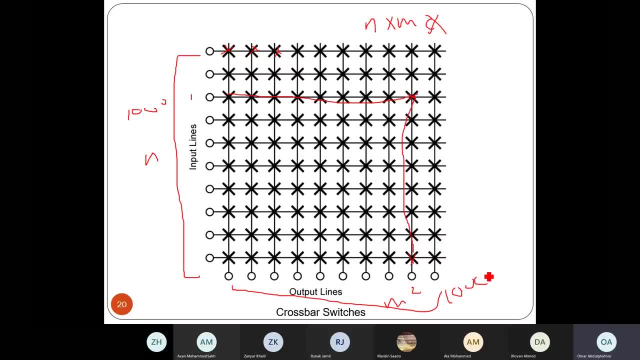 thousand, then you can imagine, requires a switch with with one million cross points. all right, so one million cross points and all these cross points can be a transistor. so you can imagine, I mean the computational complexity can be increased, what the increases of competent and output. all right, so this one we're talking about, about the cross cross bar, all. 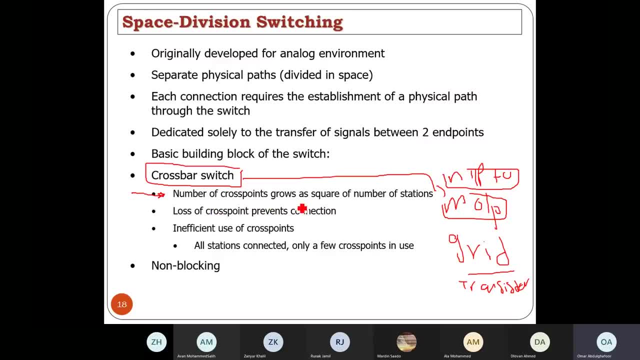 right cross bars, which is, which is the number of cross points cross a square of number of off stations? all right, squares, the number of stations, like, like what we have done previously in times. so we can solve actually this, this problem, by using multi-stage. all right, by using multi-stage switches. this. 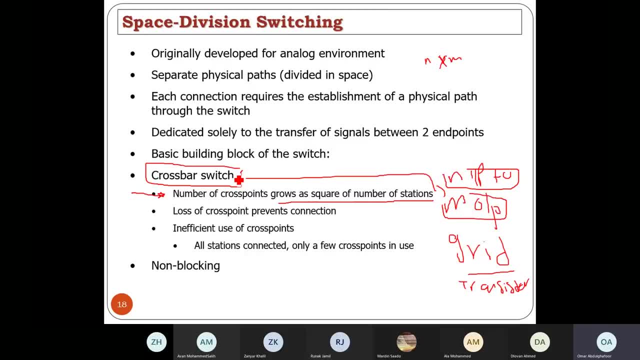 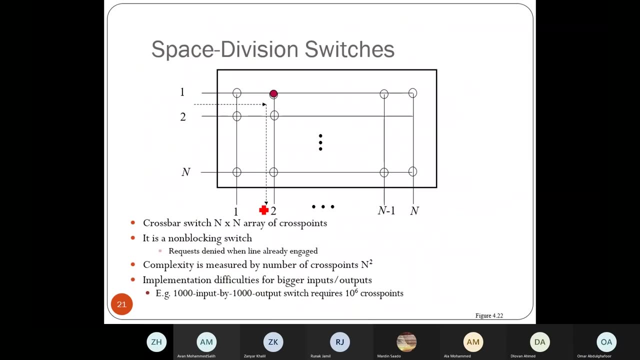 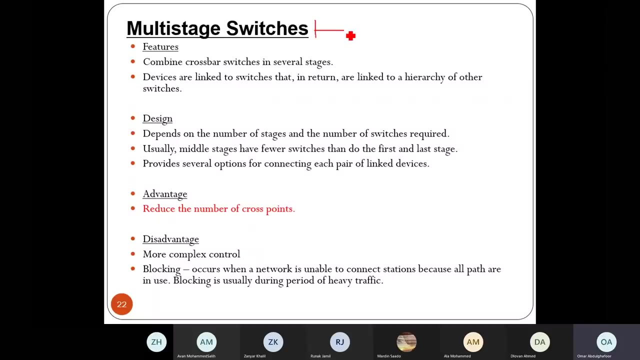 one can be. the limitation of this one can be solved by what you call it the multi-stage switching. all right, the multi-stage switching. we will talk about it afterward. yeah, this one, all right, multi-stage. This one multistage actually comes to solve the limitation of this one: crossbar switches. 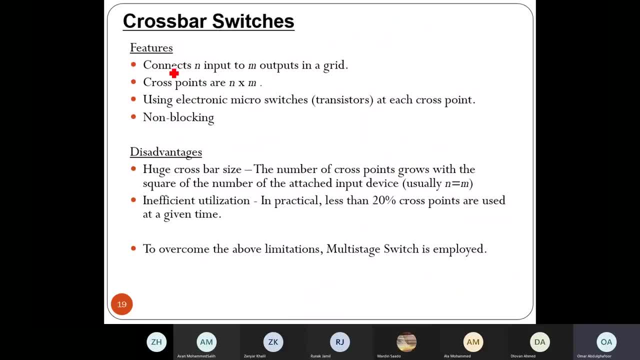 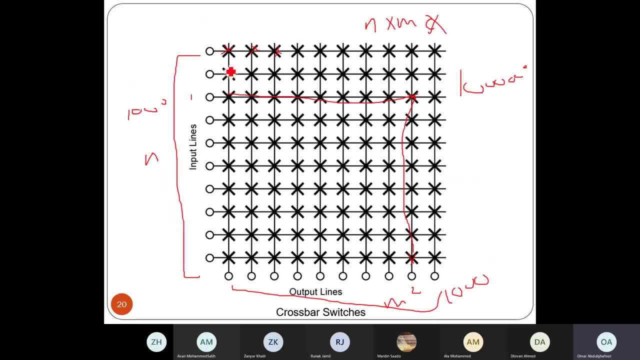 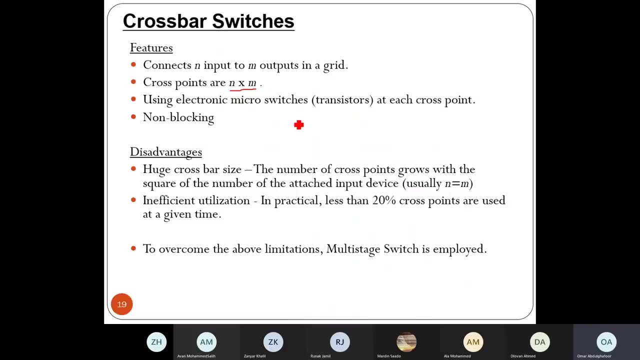 All right, crossbar switches: All right, so the features actually connect in-output to in-output in a grid. All right, so we have this one in-output in a grid, All right, you can see, And crosspoints are n times m. this one n times m. 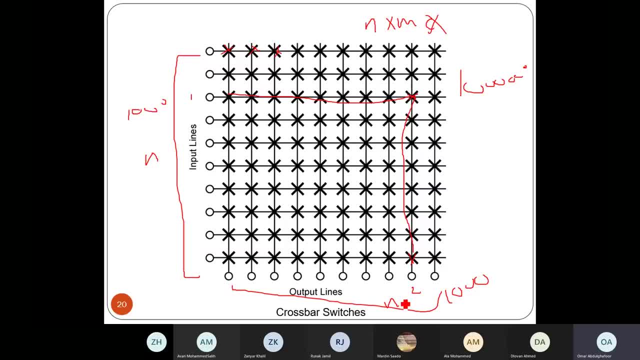 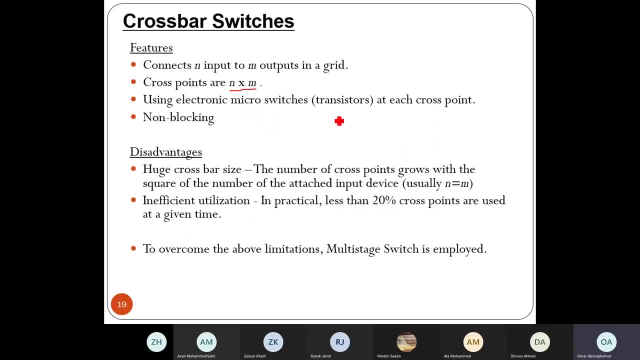 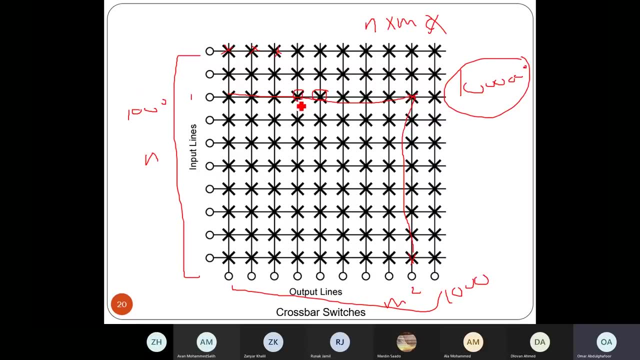 So if we have 1,000, n, 1,000, m, you can see that the crosspoints will be like a million. All right, and use electronic microswitches like a transistor at each crosspoint, All right. so this one, it's a transistor, transistor, transistor transistors and so on and so forth. 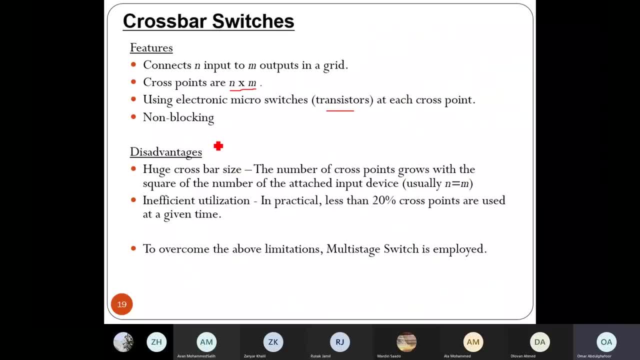 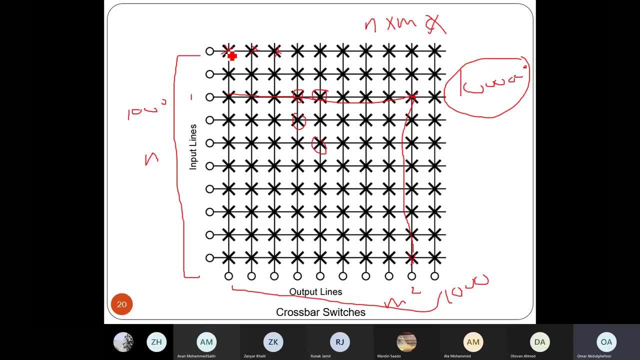 And for this one actually is an example of non-blocking, because each point can connect to To another point in a pair, All right. for example, this point can connect to this point through this, All right, and this one can go through this, and this one can go through this, and so on and so forth. 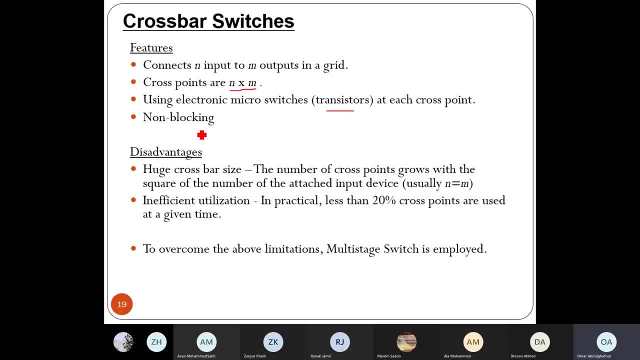 So that means that the blocking actually will be really the percentage or the probability is less compared to, for example, other techniques In terms of disadvantages of Of this one, the crossbar- All right, crossbar switches, We have a huge crossbar size. 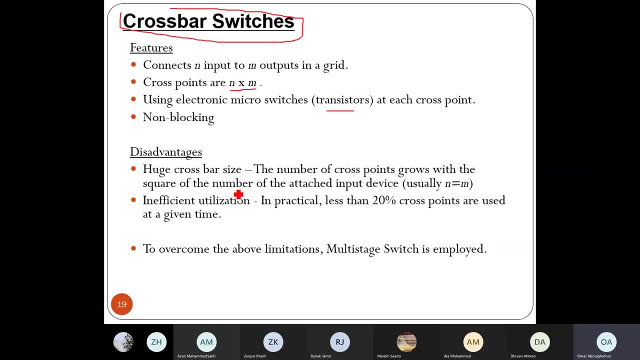 The number of crosspoints grows with the square of the number of the attached output device. All right, this is a normal scenario. N is same as m, So that means, as I mentioned, the complexity will be depend on the output and output. 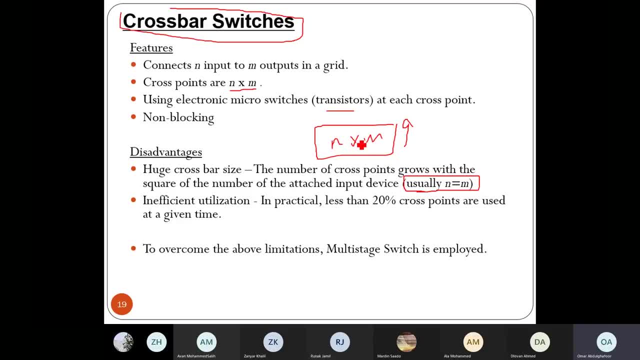 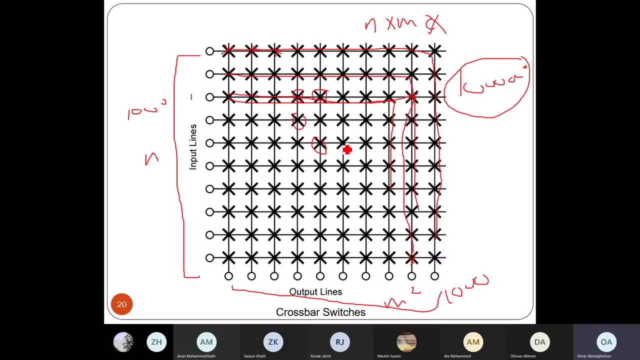 Output and output increased, Then the complexity going to increase And in efficient utilization, in a practical less than 20% crosspoint are used at a given time. So in terms of utilization, In terms of utilization of the available crosspoint, will be. 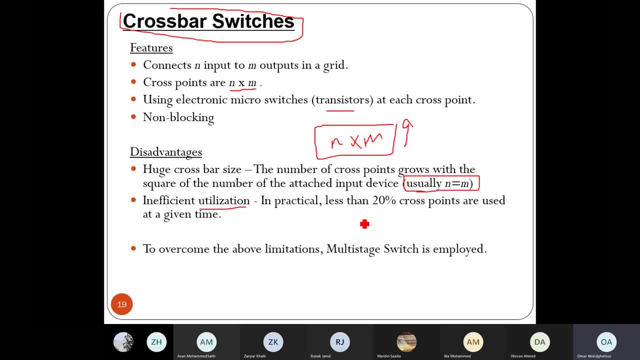 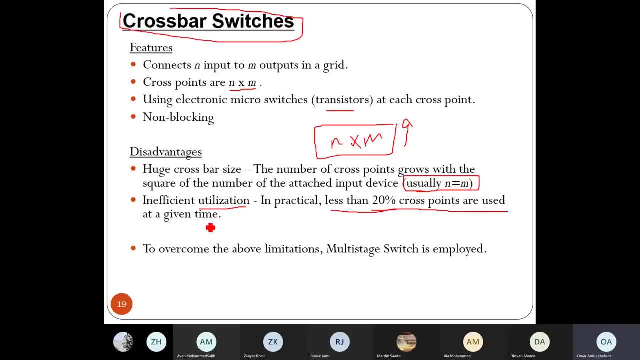 All right, less than 20% crosspoint are used at a given time. So normally this statistical study, Statistical study, normally used in a busy hour, All right, in a busy hour, Similar to mobile communication. So, for example, the busy hour for mobile communication is from 12 to 2 pm. 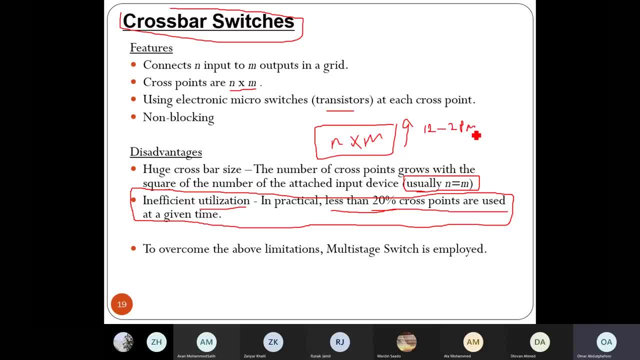 All right, I'm not sure about again the busy hour. So, for example, the busy hour here, for example in Doha or in Kurdistan, Because some other countries from 12 to 1.30.. All right, let's say to 1.30 pm. 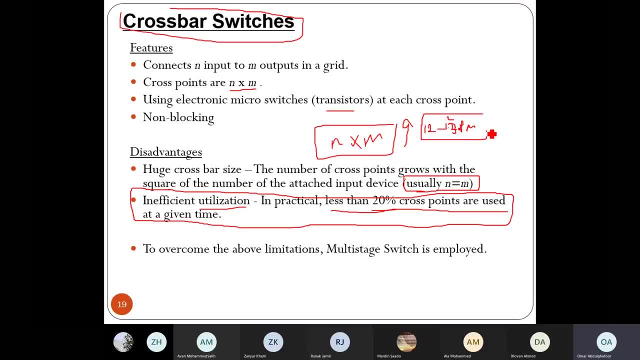 Or to 2 pm. This one actually is a break: Lunch, lunch hour And a break, And after that they continue 2 to 6.. All right, So this one actually is a break. So when we have a break, 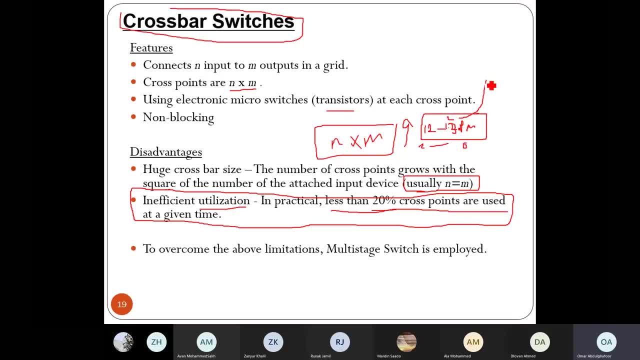 Then the probability that we are going to use our mobile is high. All right, So is this one of this. Up to this peak hour, It's the best time to do some statistical analysis. All right, Statistical analysis, So that means this is the peak where more and more and more people use their mobile to communicate with their friends. 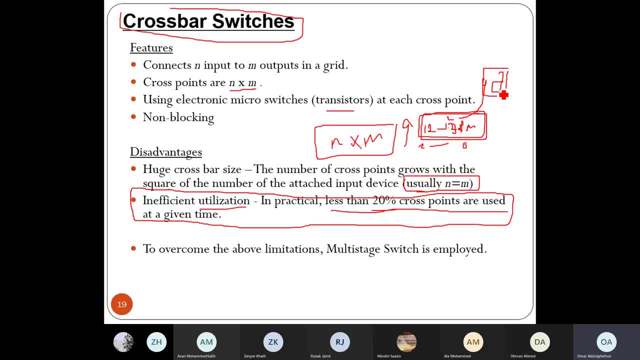 To refer to some missed call or some messages. Okay, So if I do my statistical analysis in this, The remaining will be less than this for sure. So when I said that less than 20% cross points are used at a given time, 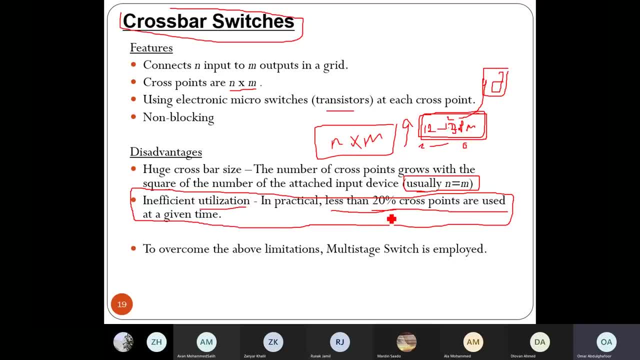 This one, actually during the peak hour or the busiest hour, All right. So to overcome the above limitation, In order to deal with this one limitation, to overcome and to reduce, We have what we call the multi-stage switch is employed, All right. 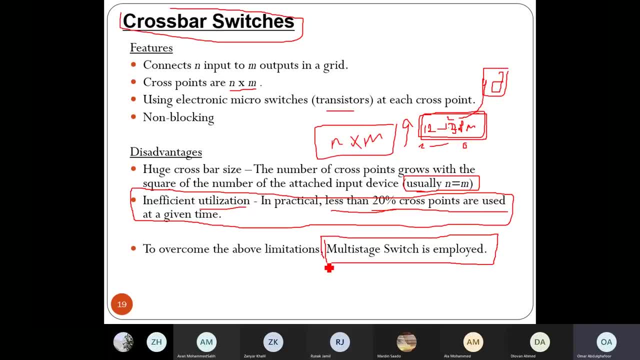 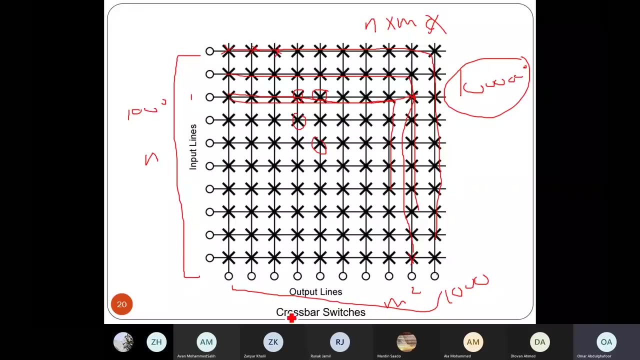 Multi-stage switch Is employed. So when I said multi-stage, the advantages of multi-stage, it's comes to overcome all the disadvantages of crossbar switching. So this is the crossbar. You can see, this is the crossbar switches. all the cross point is the electronic devices, like a, as I mentioned, the transistor. 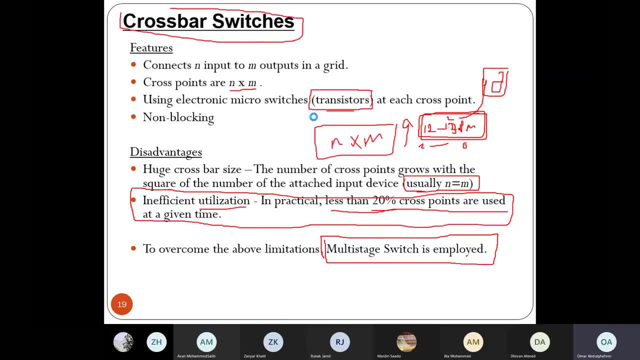 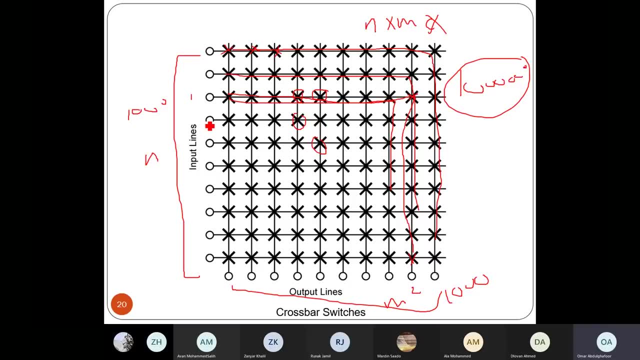 All right. So this is the crossbar switches. all the cross point is the electronic devices, like a, as I mentioned the transistor, like a, as I mentioned the transistor, like an off and on. Okay, And We said that this one, the computational complexity, and will be really high. 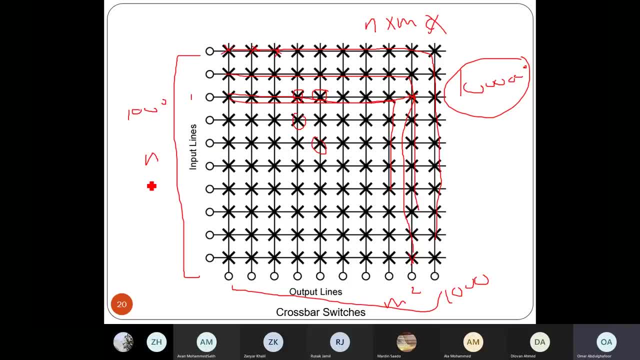 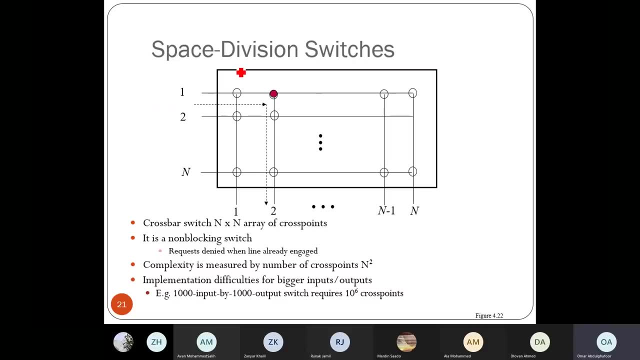 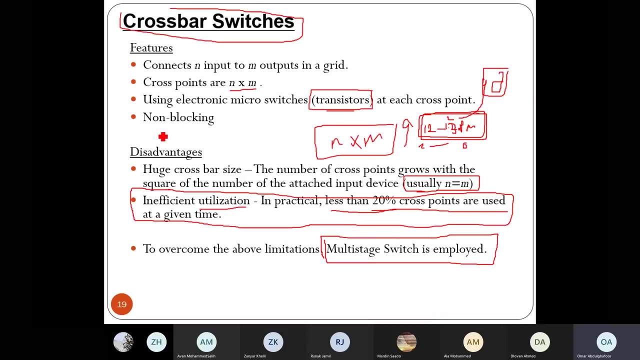 Cost. So, in order to, In order to provide an efficient Techniques, We have Space division- All right, Space Division and multi-stage- all right, multi-stage. so crossbar switch, for example, in times, in array of cross points, it is a non blocking switching request denied when line already engaged- all right, so that means it's another blocking. but we have- I mean, when we said it's another blocking is not, for example, hundred percent not blocking- that in your call will be for sure you reach your destination. 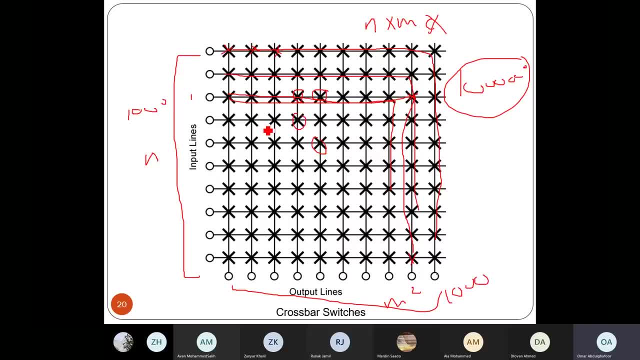 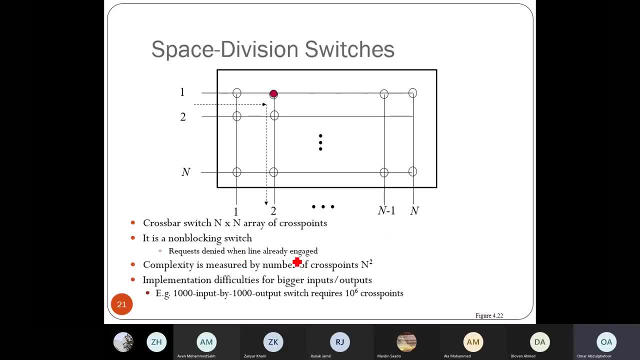 So. So we have, I mean, some probability, but it's very, I mean, Minor. When line actually already engaged, that means all the points are Are engaged, then in this case you will have some What you call it possibility of of a blocking, and the complexity is measured by number of cross points. 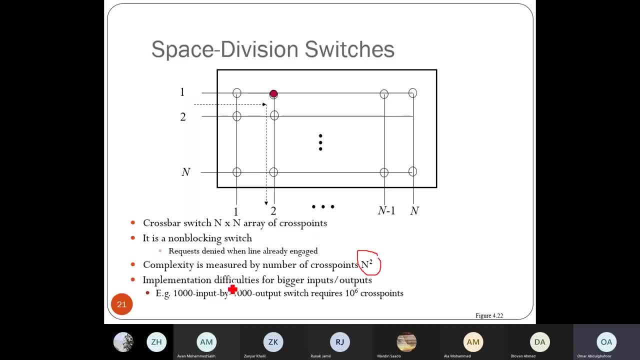 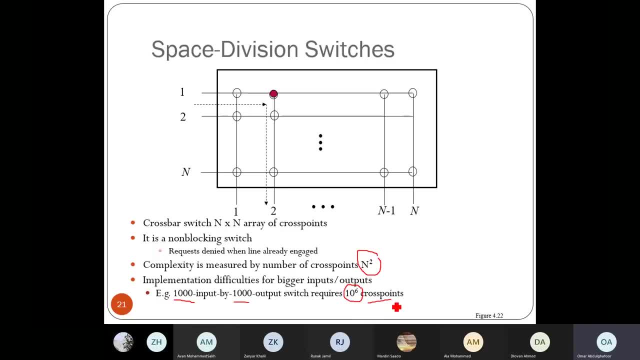 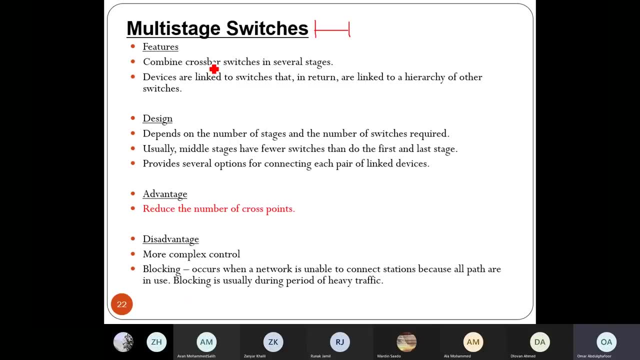 What's then? this one is the work tent to our six crosspoints. All right. So, In terms of our team, is in the features combine cross part, which is in the central stages. like, like it, Jordanense, As مسحول這句次昌才過 Stop Zombie Color Quadrat Method. However, thinking back, there's this XS and it's possible. 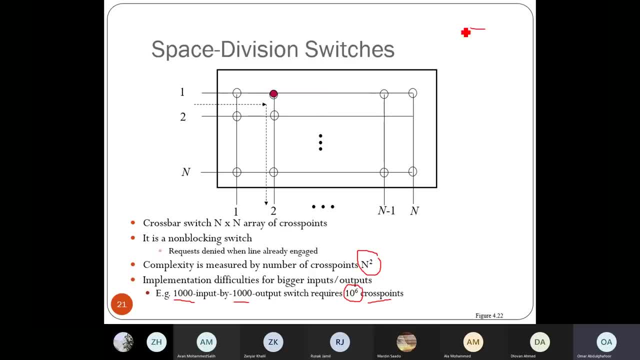 Paquette switching when we said that 101K data gone up, 12." divided into small, small packets and in. if data is divided into small, small packet, the processing time will be faster compared if we are doing processing for the entire message. all right, so 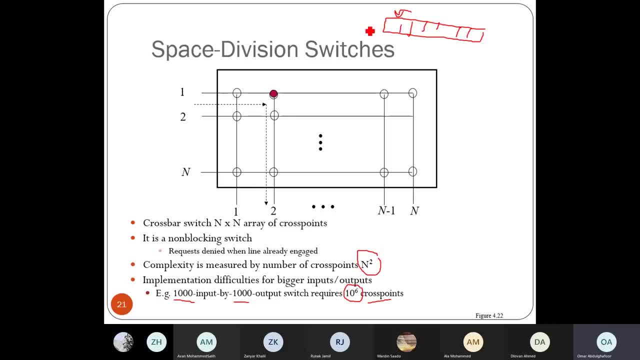 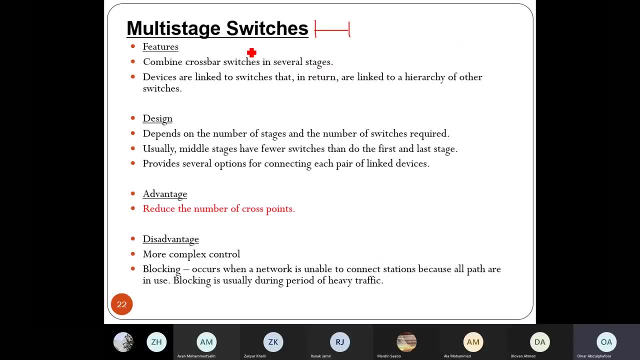 that means in terms of efficiency, this one, the packet, will be much better if we are using one block of of data. so same procedures will apply here, but in terms of multi-stage switches. so that mean combined crossbar switches, but in a several stage. all right, in a several stages and devices. 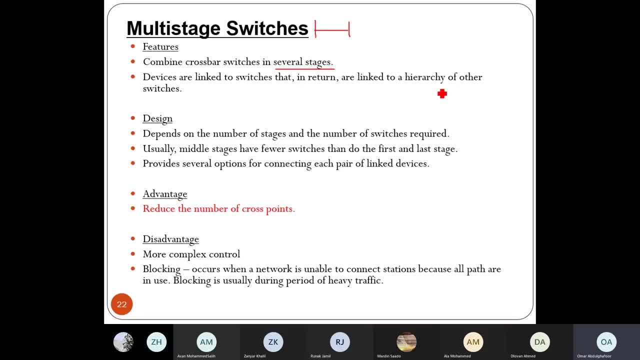 are linked to switches, that's in return, are linked to a hierarchy of other switches. all right, so in terms of of design, so depend on the number of stages and the number of switches required, and usually middle stages have fewer switches than the first and the last stages, as we will see afterward. all right, this one the key features. 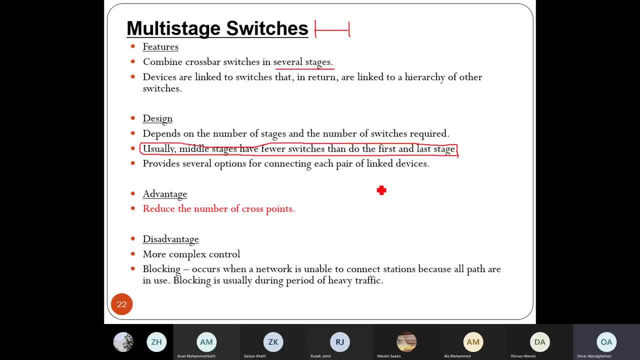 of the design of multi-switches. so we have input and we have output, so this one must be same. for example, if i said 200 times 200, so that mean here is 200- how many blocks, i don't know, depend- and here the output is 200 with same. 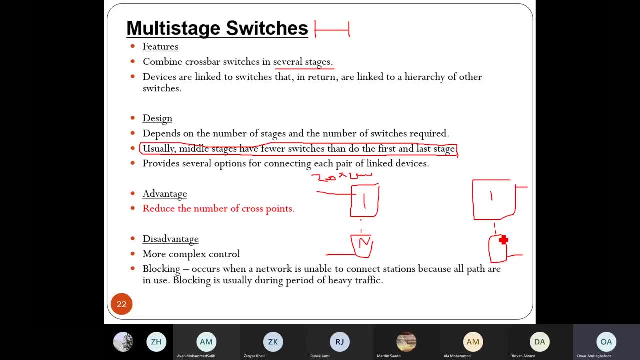 so that mean number of blocks. for example, 1 to n here, also 1 to n here. all together i have 200 here. the output altogether 200, but in between i can play around. previously crossbar, this one will be all together in a grid, but in this case multi-stage switches, i can play around in this. 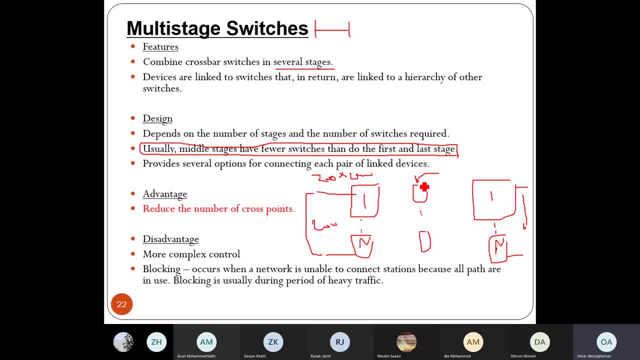 middle stages, which is here middle stages. this one, all right. middle stages have fewer switches than the first and the last stages. all right, fewer switches. but we have some formula actually to some procedures to follow in order to design the entire switching circuit. all right, so provide several options for connecting each pair of link device. 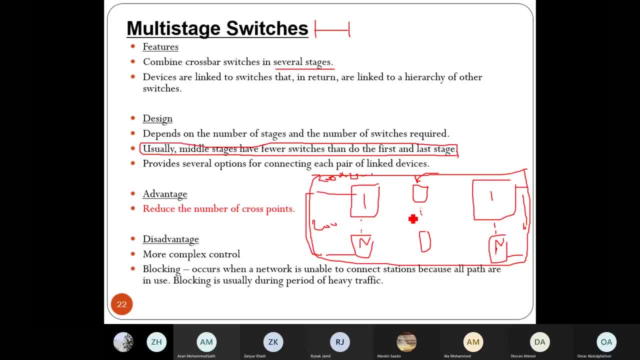 because we have middle stage in between, so we have some options to which blocks we can. we can follow us and the main advantages of the multi stage switches is the reduce the number of cross points, reducing the number of of cross point compared to this one crossbar. 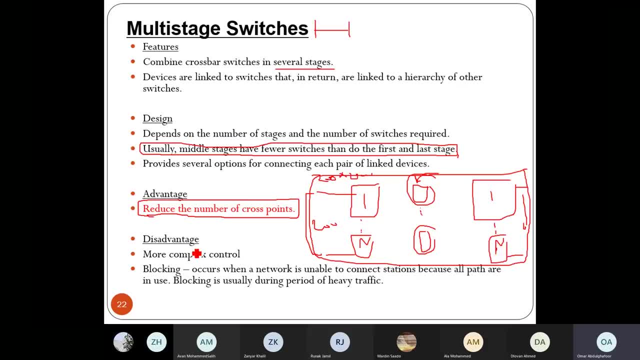 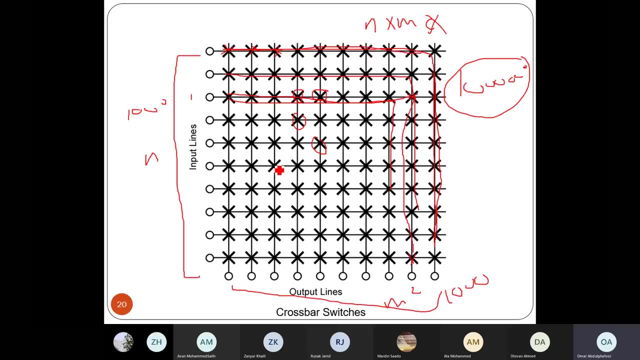 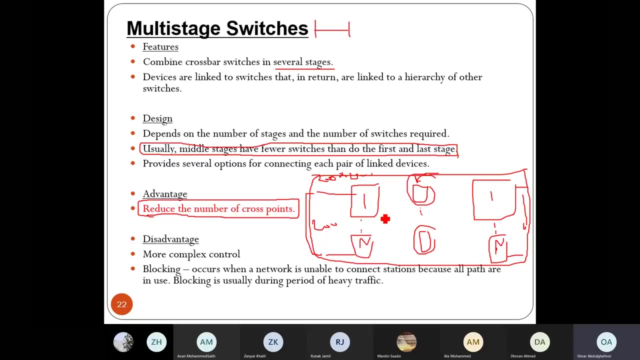 and the disadvantages is more complex than the main advantages. more complex control in terms of controlling units, then, will be complex compared to this one, because this one you can see if you like, it's very straightforward, you can connect. but in this case, in terms of controlling, we have different stages- 1- 23- and each stage has its own switches. 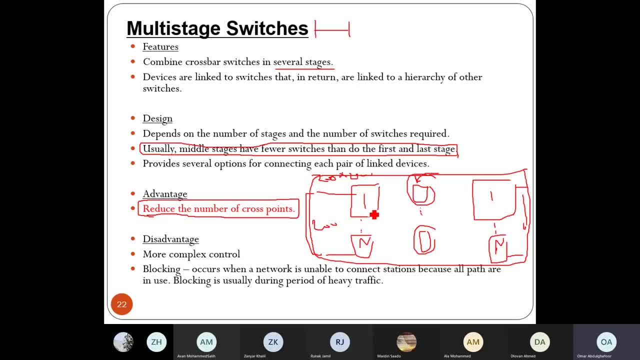 output and output. so the controlling process will be uh, complexity will be high, and the blocking occurs when a network is unable to connect stations because all paths are in use, all right, and this one. the blocking is usually during the period of heavy traffic, this one, the busy hour. 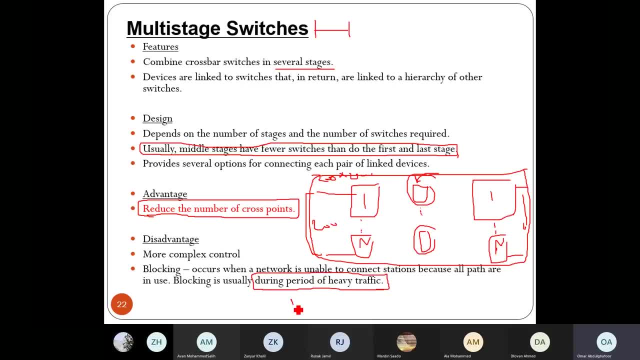 normally in in wired and wireless we have what you call it the busy hour. as i mentioned, in mobile, normally all the statistical studies would be 12, between 12 to 2.. all right, even in washington dc, which is the most crowded city in the world, where both commercial and and government offices are. 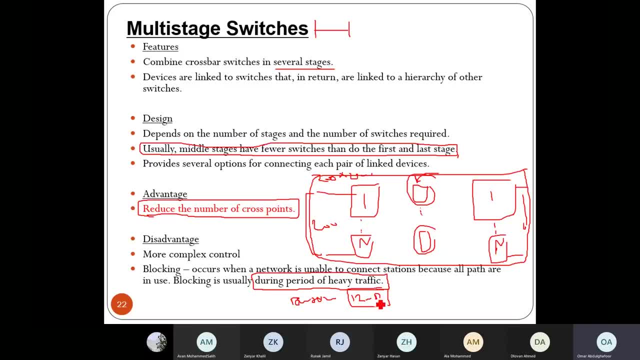 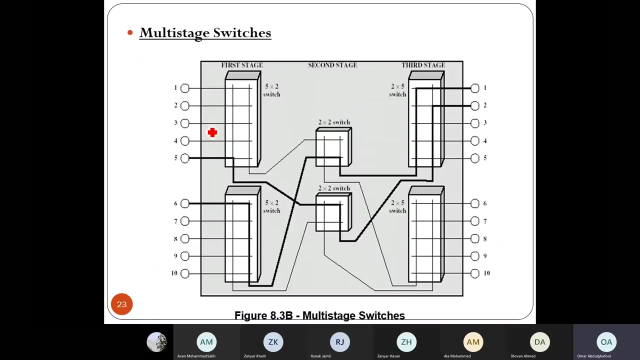 there there are statistical analysis between 12 and and 2 in washington dc. all right, so this is, i mean, general, general uh overview of the multi uh switches, uh techniques. all right, so, for example, here we have multi stages, so now it's this one, it's um. 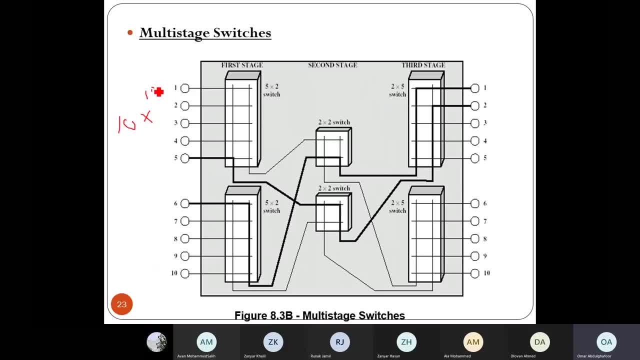 10 times 10. all right, 10 times 10.. you can see how many input i have: one, five, six, ten. so this goes for the input stage, or the first stage, and the last stage or third stage also i have 10.. okay, the input, this one and this one should be same, or usually same. so i have one five. 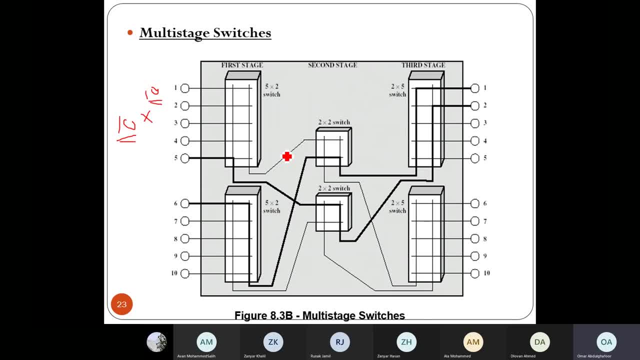 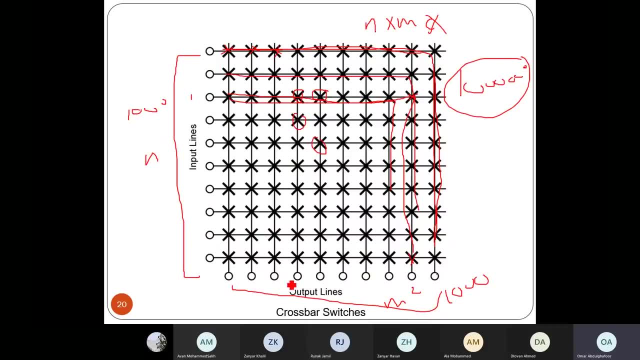 and six, ten. so previously, if i would like to use the crossbar, then i have just one, two, three, four, five, six, seven, eight, nine and ten, and here i have 10 in between, i have transistors in between, i have cross points. all right, which is all. 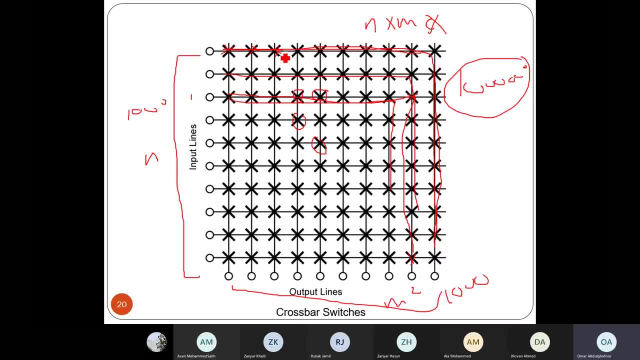 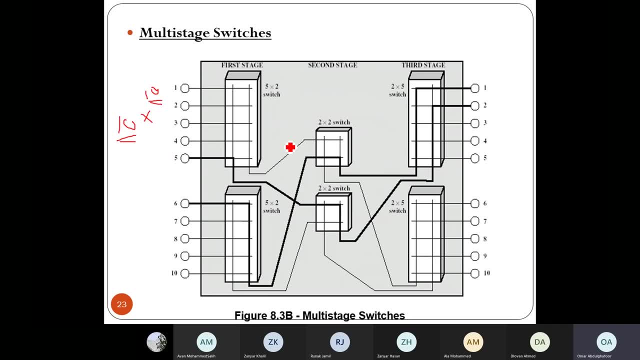 and all we have ten. so each line we have ten, one, two, three, four, five, six, seven, eight, nine and ten, and so on and so forth. but in this scenario we have some stage in between. all right, we have some stage in between. so i divided the first stage into two blocks. so each have five. 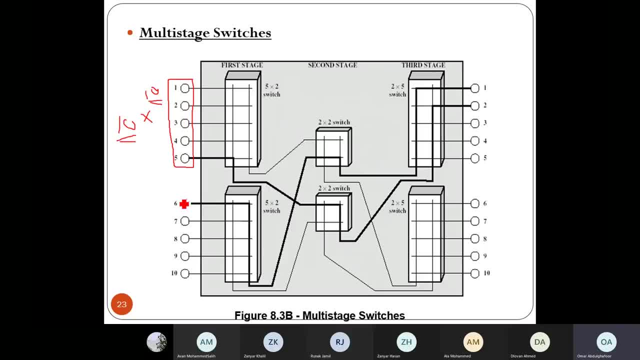 inputs. for example, this one, one block is five and another block is is five. all right, so since i have two, then this one will be five times two. all right, five times two, all right. so in this particular scenario, in between the second stage or the middle stage, 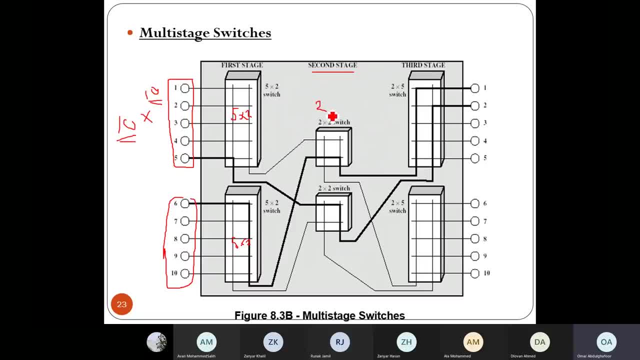 so i have two, then this one must be two times two because the last stage should be same. so if i have five times two, the last should be two times five, because i need to generate five for each blocks because, again, as i have agreed, i have tens times tens. so in this case, in between i have two times two and two times two, so two blocks. 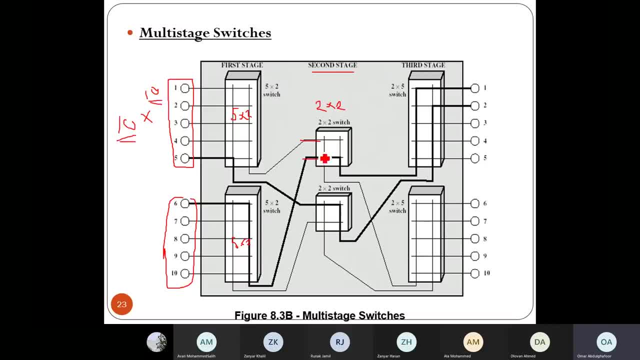 two times two, all right. so that means this one will be two and two. all right, two and two. and this one will be also two times two. so this one should be same. you can see, for example, five times two. here i can start by two, all right, and here five times two. i can just put it here: two. 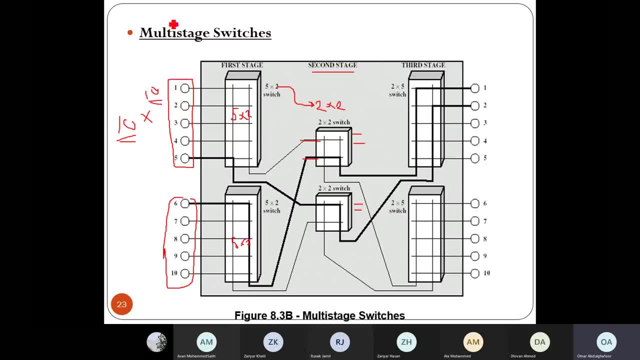 times five. all right, because the output and output must be identical. output and output. for example, here i have 10, combination of two blocks. here also i have 10, which is combination of two blocks. all right. so if i design this one five times two and this one the, the information i mean provided by 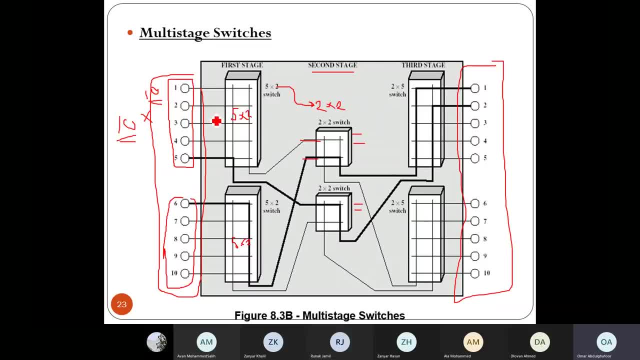 by, by a formula- we will, we will check it afterward, but i mean generally speaking. all right, so five times two, this one should be two, all right, and this one should be two times two. why? because here i have two and here i have two, all right. so this one will be two times two, all right. so here is two, then two. 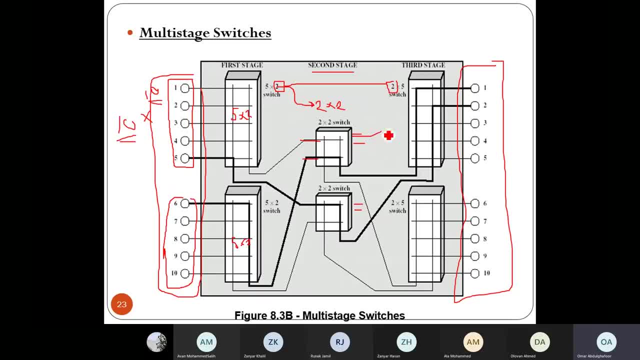 then here is two times five. all right, then the output from here, for example, will, for example, five will go to this uh blocks, and from this will goes to to this one, for example, all right, and from this one can comes to this blocks and go down until reach to six. so from six to one and from five from this work upper. 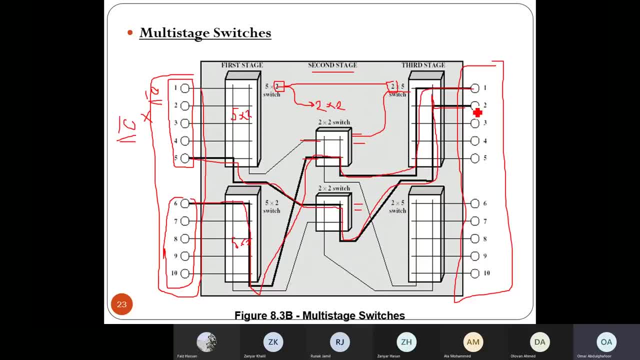 block to the to two in the upper block of the output stage. all right, so this is the way i mean. the general scenarios in the in the model is like this: okay, so that means when i have a doctor here with me, um, i'm making an, would like a one-hehe. 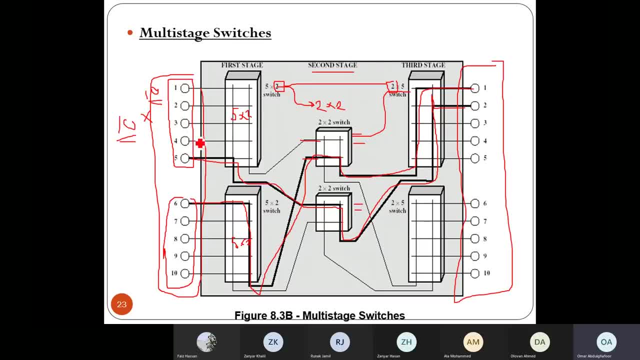 and i will tell the has to são so if i want to know interesting in how to divide this and to do this. we have ten, so many multiple color shapes. that is mean i need to re-organize or regroup the output and output in in a way that i can. they can improve the processing, all right, they can improve this processing so they can improve the efficiency of the overall switching center. 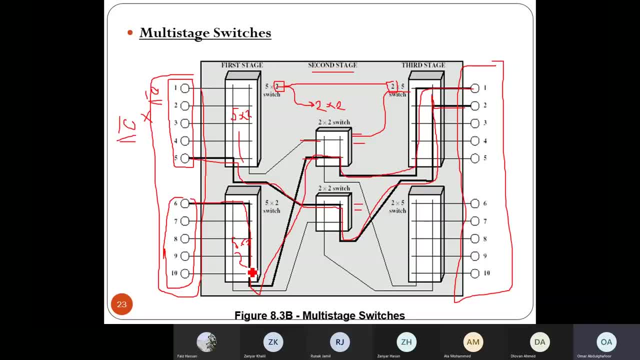 mean this block. i have one and two blocks. all right, one and two blocks, so each blocks, because i have 10. so that mean one, two, three, four and five. one, two, three, four and five. five plus five will be 10. so this one i said is five times two. then the last stage should be the other way: two. 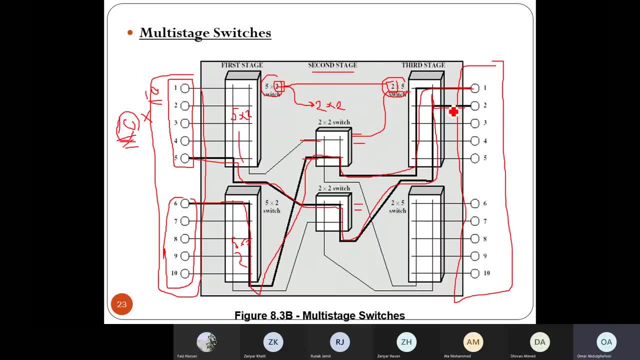 times five, and each one- two, three, four, five, plus one, two, three, four, five will be 10. so this one, 10 and 10 will be same. all right, 10 and 10 will be same and in between again should be also match with the outputs of the first stage, for example, two. then i have two times two. 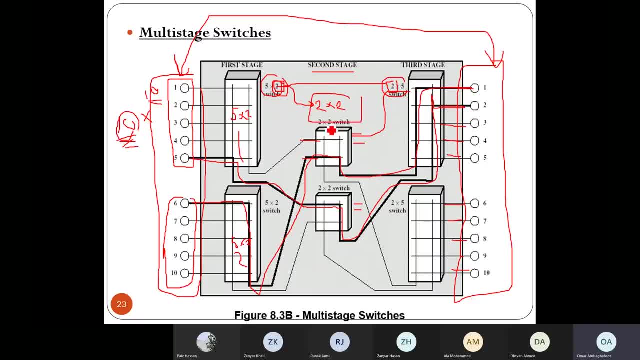 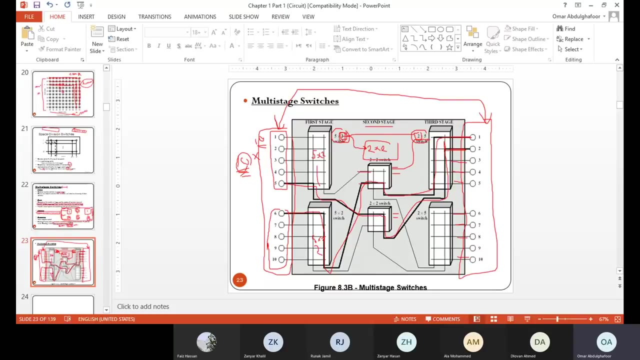 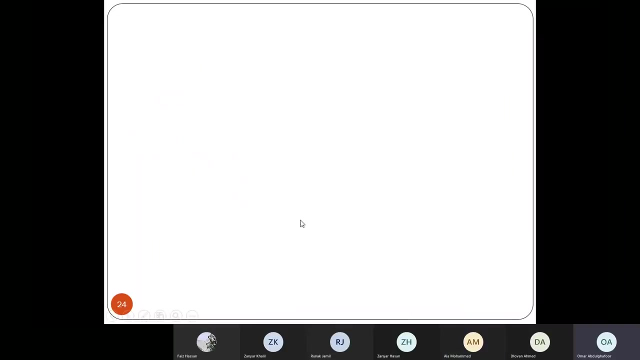 here two and here two, then this one, two times two. um, all right guys, this one is a. the general description is: is it clear? yes, sir, all right. all right. so here, if i said, like i have similar to what i have done times, times 10, all right, so i can divide into two groups: one, two, each, one two, three, four and five. one, two, three. 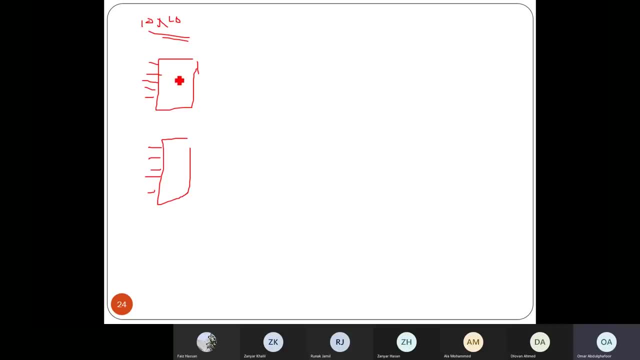 four and five, all right, and here in between. so this one will be five times two, five times two. here i have two times two, one, two, Alright, this one one and this one, two, and this one one and this one too, And this one also. 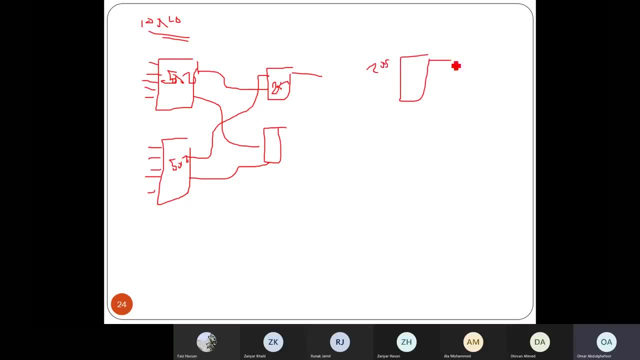 Uh, two times five. So here 12345.. And here one, two, three, four and five two times five. So that means this one went from here and went from here and went from here and went from here. Then this is my all. 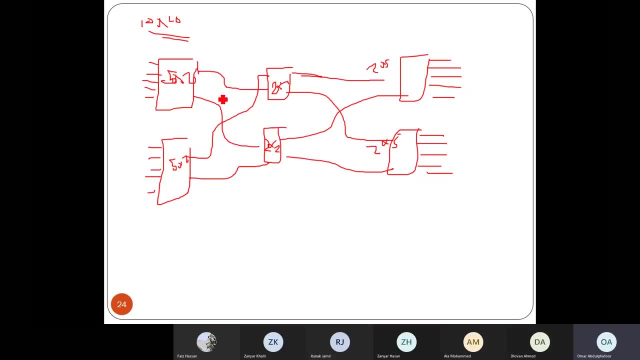 Uh, switching circuits. Alright, all switching circuit. OK, so this is multistage: stage one, stage middle, stage two and the last, the last stage. five times two I have five and I have outputs two, and two times two That mean I have two. 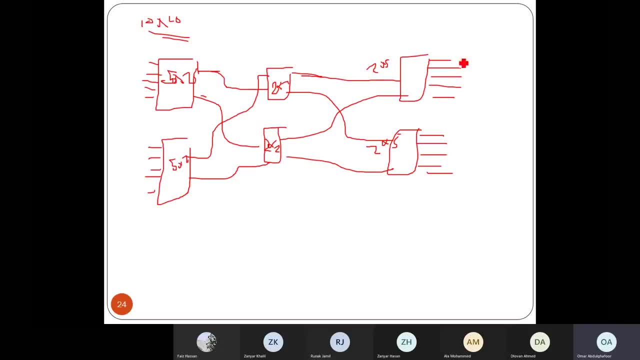 inputs to output, two inputs to output and two times five. I have two input, five outputs to input, five out. So I will take this one, So I can connect both and this one. Also, you can take one from this and And one from the second. Alright, the second block, the lower. 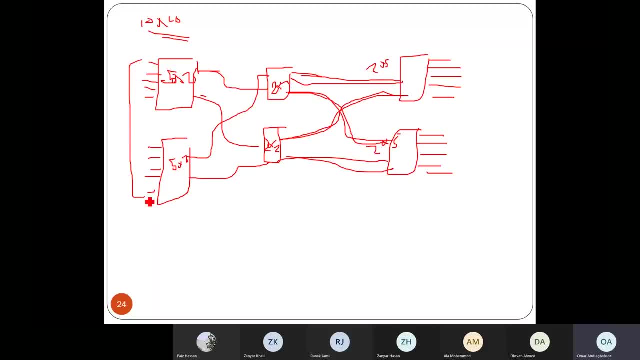 block. So in this case we have, we have altogether, here is a 10.. The output altogether is a 10 and in between we have designed some, some blocks that refer to what you call it, the multistage. Uh, I'm on stage technique. 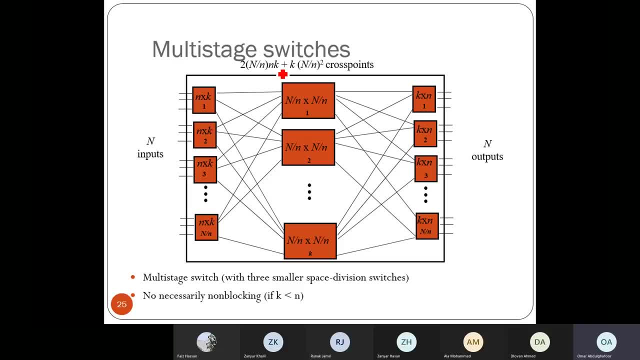 Or multistage crossbar, or switching. Alright, so here we We have some, some formula to check the cross points. For example, if you'd like to calculate the cross point, then, Uh, then you can see this one to end, divided by small N and K, and. 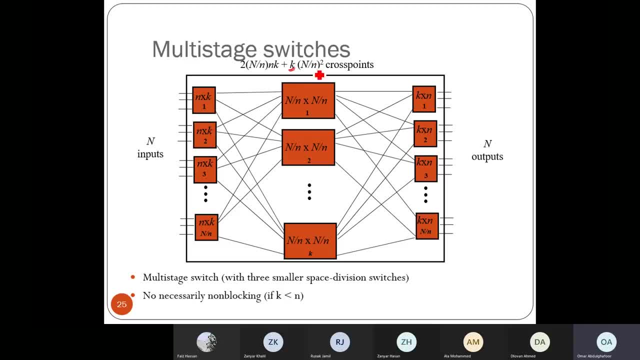 this one will be provided K, alright and N and capital N. So when I said capital N is the output, Alright, input is here and will be same. output is is here, Alright. so in between this one, the output and output will be N times K. 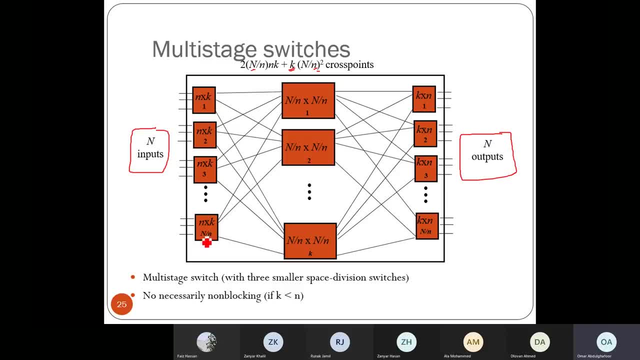 Alright N, times K and times K until we reach to N, divided by small N. alright, and divided by small N. So this one will be provided, alright for the design procedures And depend on the scenarios. will be provided That mean, for example, should like to design, the manager will. 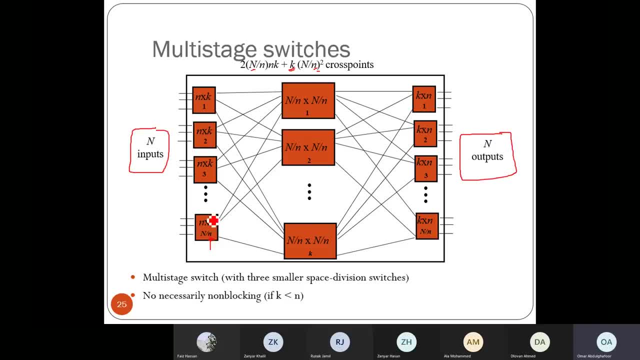 Will ask you that these the blocks that is required and this is the number of of input and output- small input and output in a K. Then you can, You can, You can go ahead and and design your own Uh multistage switches. 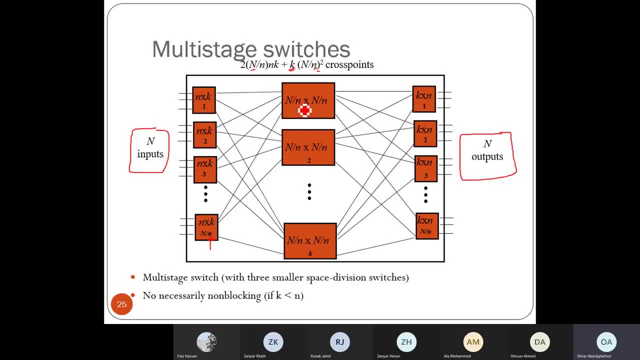 Alright, so in between, here we have N divided by N, times N divided by N, So this one, it's identical. Alright, so for example, I have: here is 200.. Alright, so for example, I have: here is 200.. Alright, so for example, I have: here is 200. 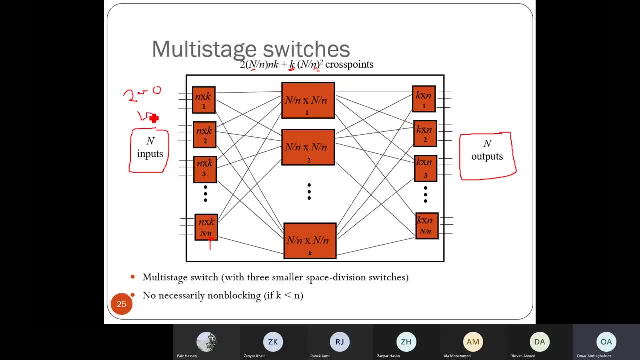 And here small, and I have as 10, then 200 divided by 10 is 20.. Then this one will be 20 times 20.. Alright, 20 times 20, and in terms of the blocks, 12 until I reach 2.. 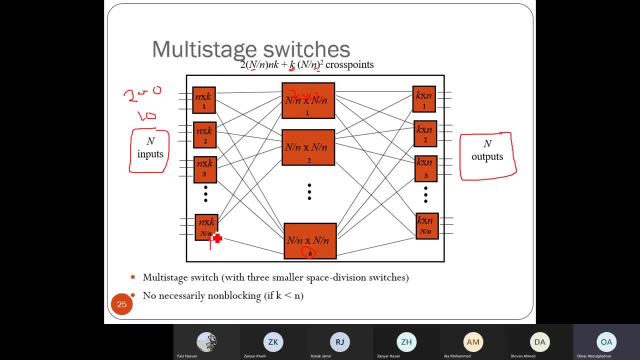 K, small K, and this one 123 until I reach 2.. And divided by N. So if I have 2010, then this one until 20.. That mean 1234567.. Until I reach 220.. And if I have 200, then how many inputs for each? 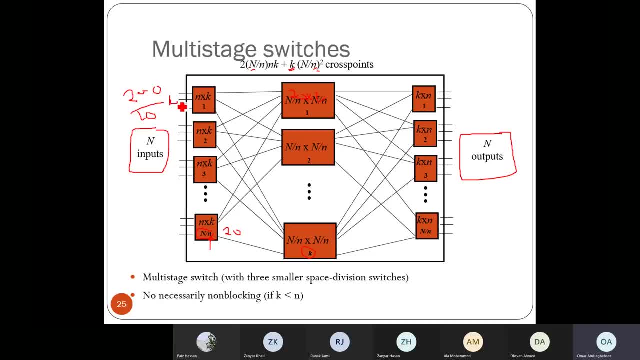 How many input for each would be 10?. Alright, so this one will be 10.. This one will be 10.. This will be 10 until I reach 20.. This one will be 10.. So 20 times times 10.. 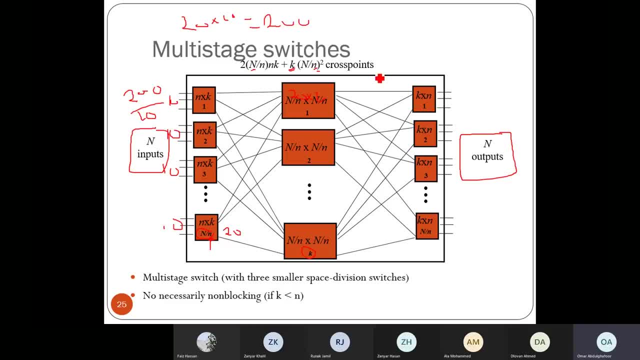 20 times 10 will be 200.. Alright, and same goes for for the output. Same goes for the output, but this one you can see, and times K. This will be K times N. Alright, K times N. Alright, K times N. 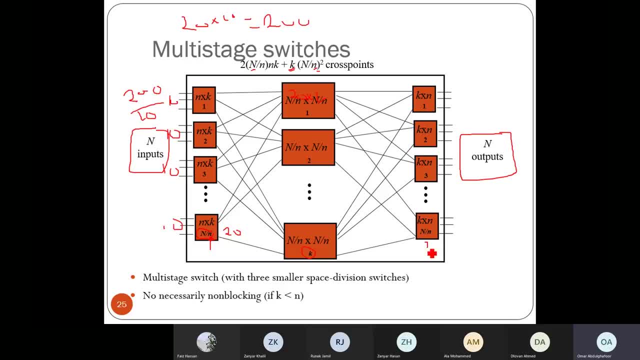 So from 1234,, for example, until I reach 220.. Alright, until I reach 220, because N divided by N- I assume that they have The 200 for for hand capital and for N Small, which is the output for the, each blocks would be 10.. Then I have 20, so 20.. That means each blocks about 10.. 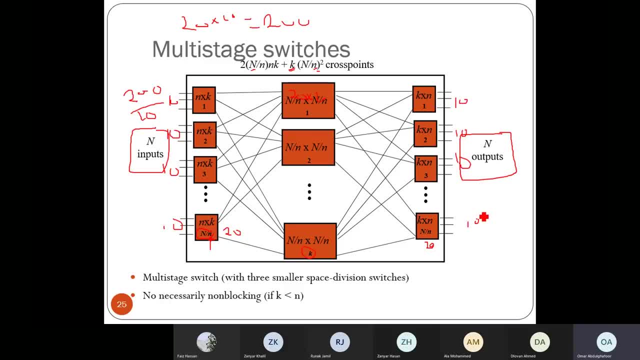 Alright, this 110 and this one altogether 10.. And Can take: Alright, so this one actually is Depend on the value of K PCI. Then I can take, For example, this one 10 times By 20 and this one would be 20. this 110, then this 120 times 2018 is 110 times. 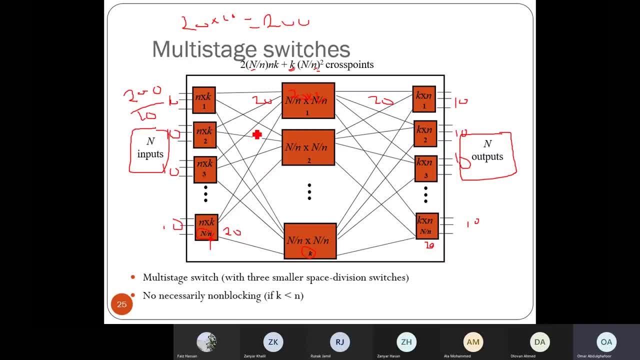 20 and so on and so forth. Alright, so we have, We have such a procedure. I will some example and try to solve it step by step. but this is the way how we can calculate the cross points. all right, cross cross points will be, i mean, less compared to the cross bar. 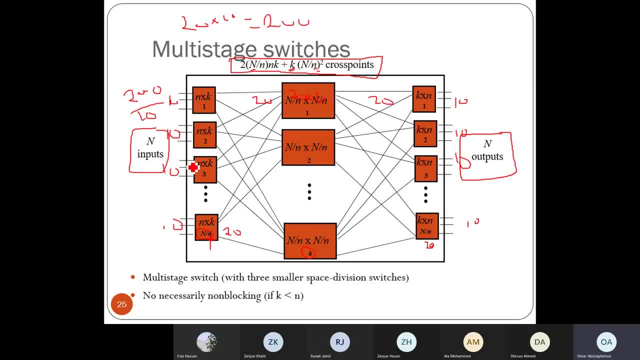 all right, less compared to the cross bar, all right. so multistage switch with this me uh three smaller space division, uh switches and no unnecessarily non-blocking if k less than n. so if you would like to go for uh non-blocking, all right, k is less than n or we have some close. 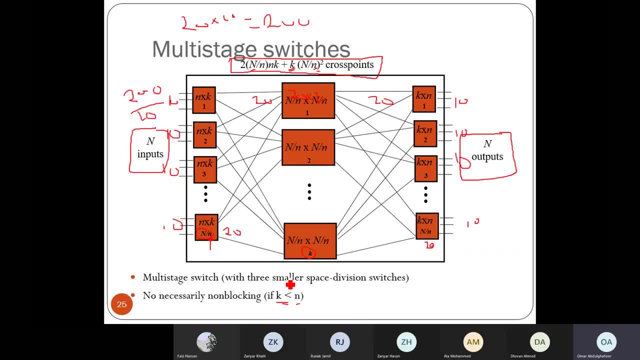 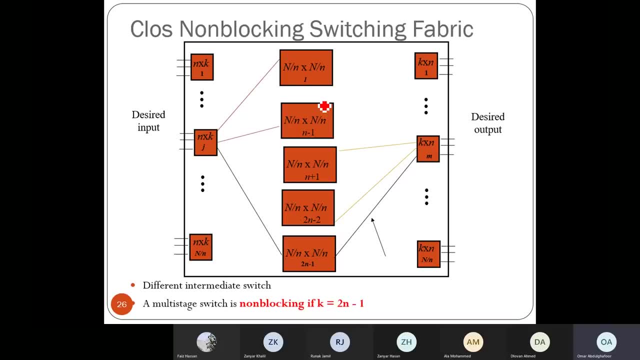 uh, we call it the close condition. all right, close condition if we would like to. i mean design our, our circuit switching without, or assuming or making sure that non-blocking all right. so we have what we call it close, non-blocking, switching uh fabric. so the class has its own uh condition. 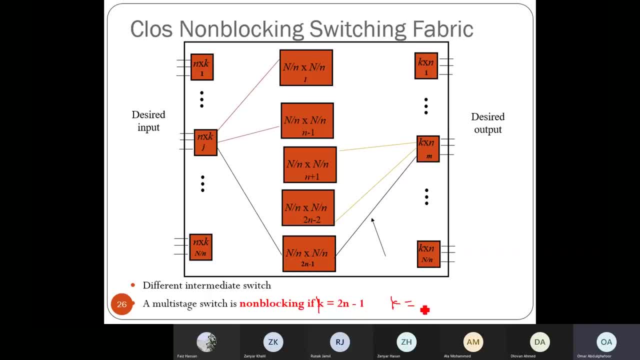 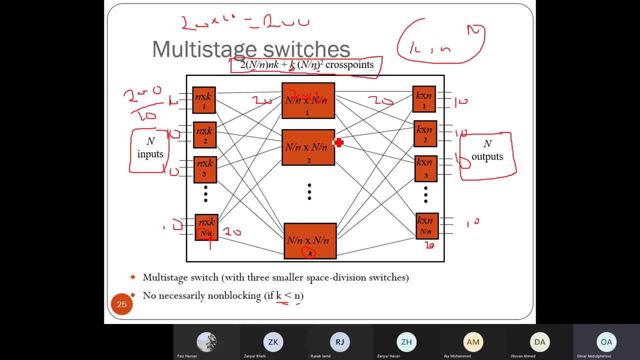 making that k should be equal all right to 2n minus 1.. so from the given n we can determine k, all right. but in the previous one all are provided k and and n, n can be. also we can straightforward calculate, but in this particular case we might experience some. 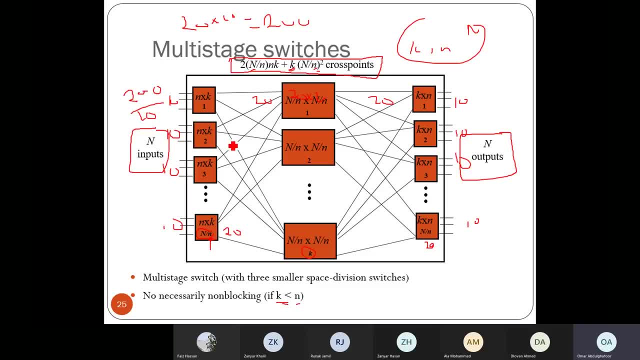 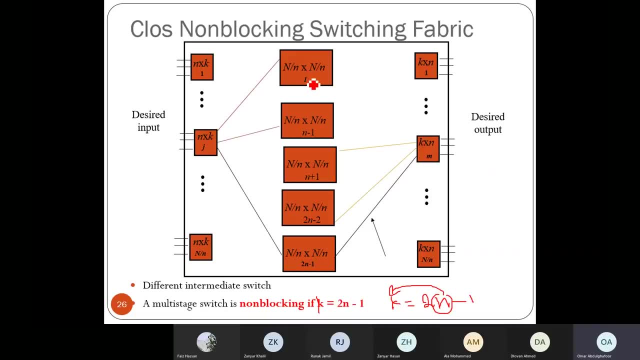 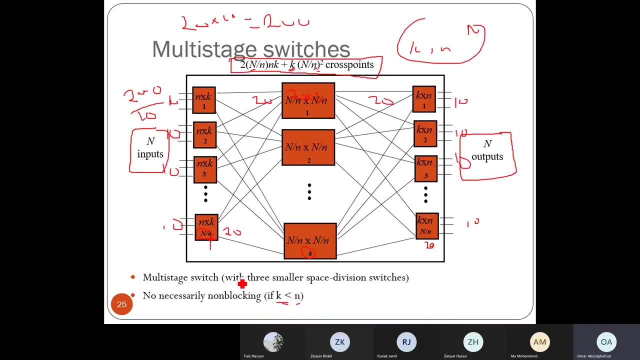 somewhat. you call it blocking, but if you would like to make it non-blocking, all right, non-blocking, switching uh networks or telecommunication network, then we can follow what we call it the class clause condition. again and again this one. actually the blocking probability is really reduced compared to this one. we cannot say we don't, we have, i mean, such a great network. 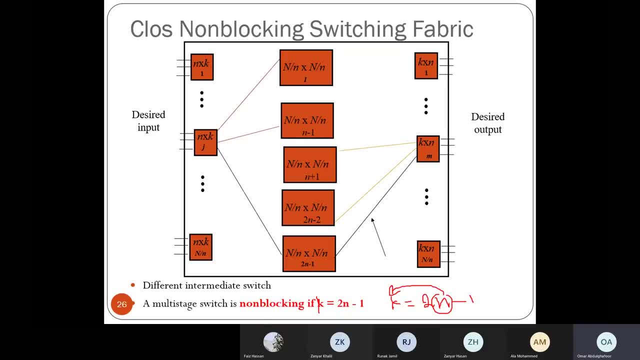 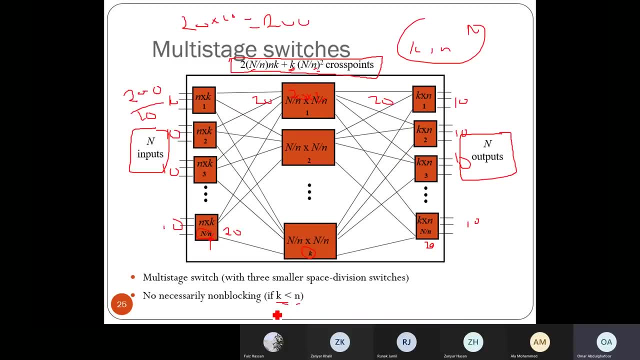 there is no blocking, hundred percent, all right, but maybe the blocking here will be really, um, i mean less or few compared to them, to the previous one, all right. so this is how the the switch inside. you remember the first slide, or second slide. we said: we have one, two, three. 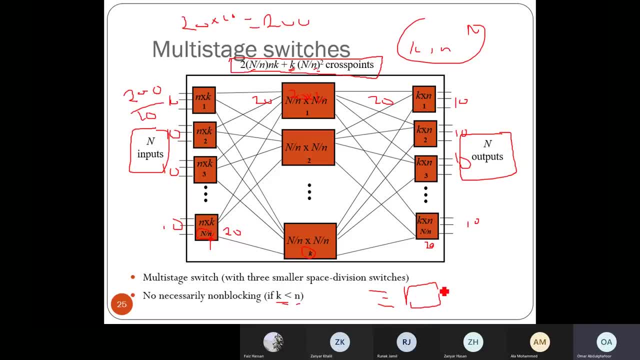 all right, and we have switch and we have one, two, three, all right, we have three nodes: a, b and c would like to communicate d, e and f. so in between here we said we have some switching, all right. so now we are, we are discovering this one. 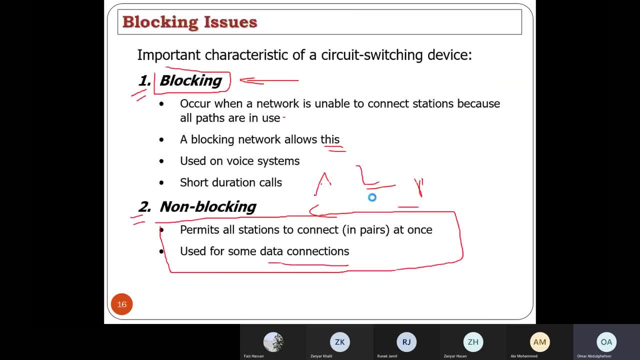 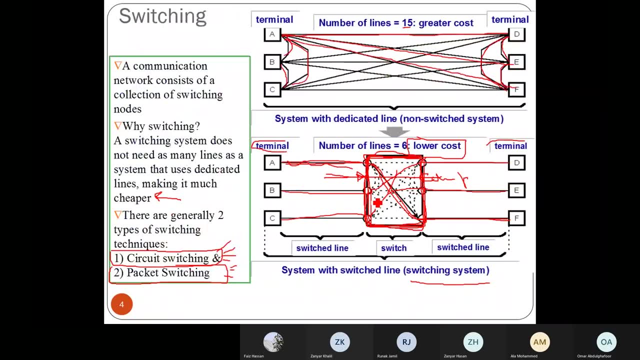 all right, we are discovering this one. if you remember here, what is it? um, yes, this one, you remember this one. terminal a, b and c would like to communicate with this one and we said: here, we have, we have, we have switches. so now we are, we are here, actually, we are, we are gonna. 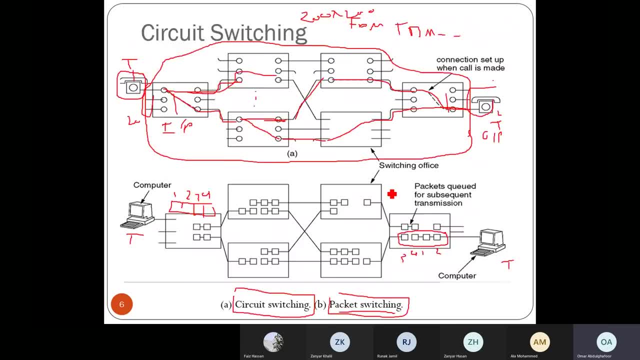 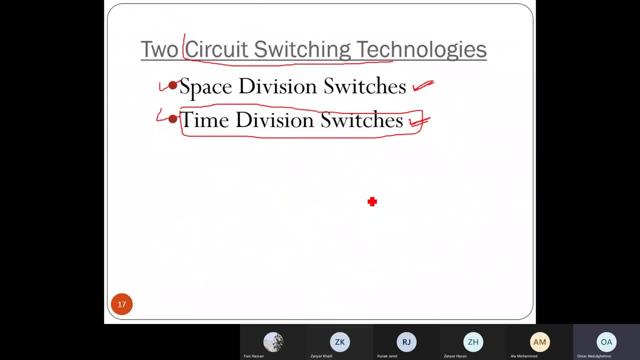 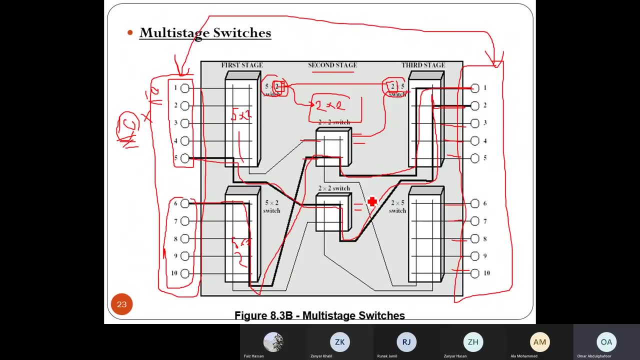 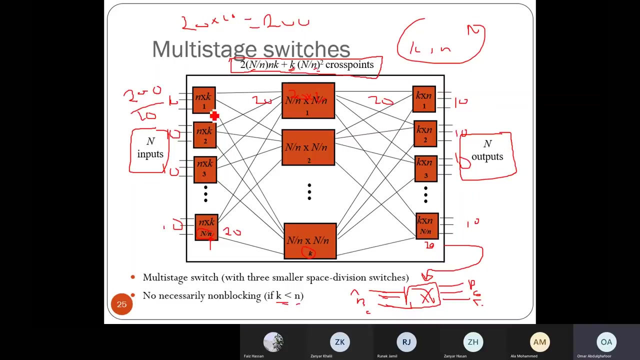 design this one and we're gonna discover, all right, we're gonna discover even the- uh- multiplexing, even the multiplexing, all right. so this one actually is the block that we have highlighted previously. uh, yeah, all right, this one, the block that we we have highlighted previously- what happened inside. 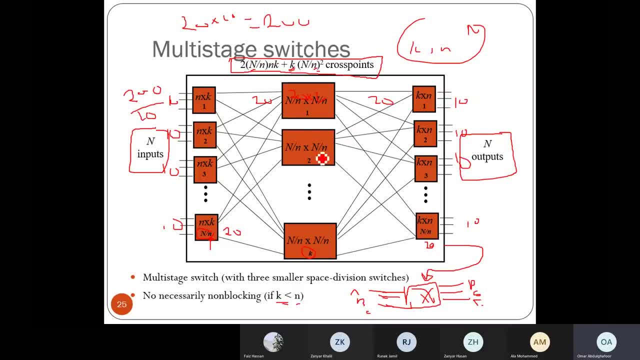 all right, what, what's what's what inside? so we are, we are zooming here. okay, zoom in to see what is inside the- uh, the switching center, or what is inside the exchange office or the switching office. all right, so again this one. if you'd like to compare the complexity, if you'd like, 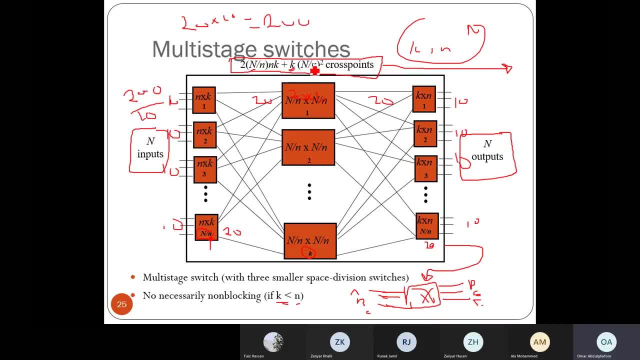 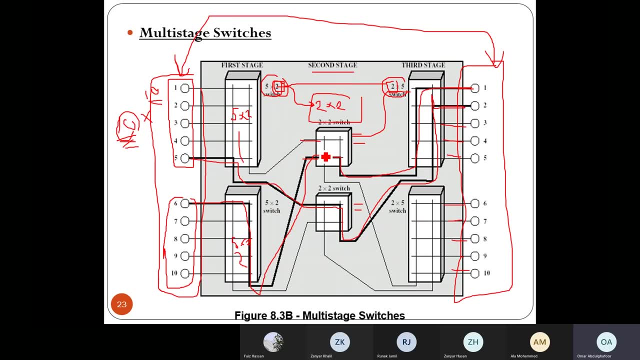 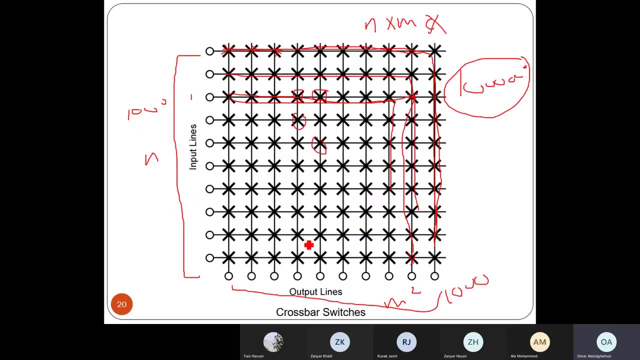 to compare the complexity. so for any given n and n and k, we can calculate the cross points. how many cross points? so we can compare, for example, this one with uh, um, with this one, all right, with the crossbar, because this one we call it the crossbar. you have to be careful, because in 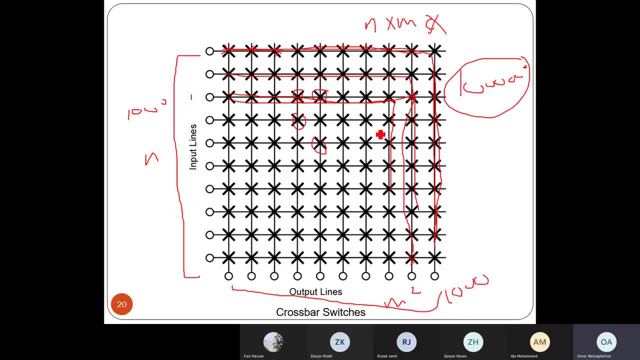 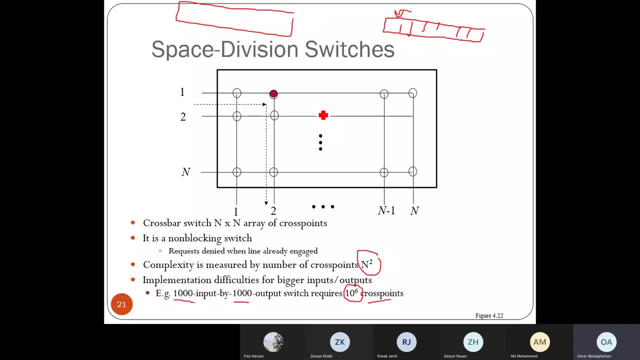 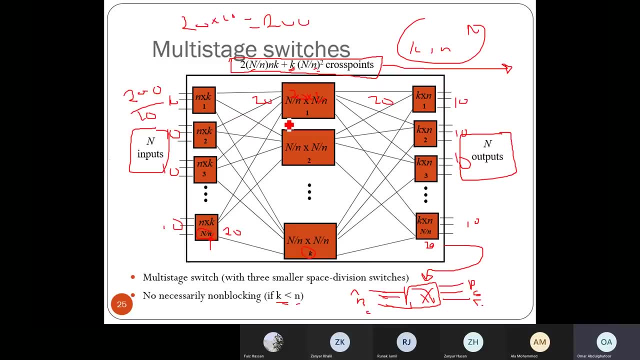 design. if i ask you to use crossbar, then then you have to generate such a grid and all the cross points, or you can just draw a small transistor and if if ask you to design using multi-stage, then we have to follow this multi-stage procedure. all right, multi-stage switch procedures. 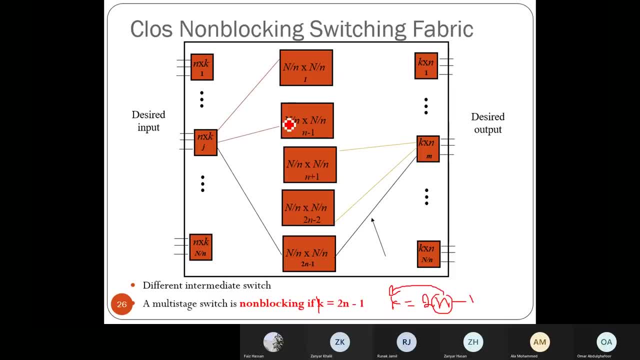 all right, all right. so here we have, for example, desired inputs and desired output. this is the condition. so sometimes the question asks you to design using this one and redesign. all right, for same, for same scenario, using non-blocking. so, for example, if i ask you to design, 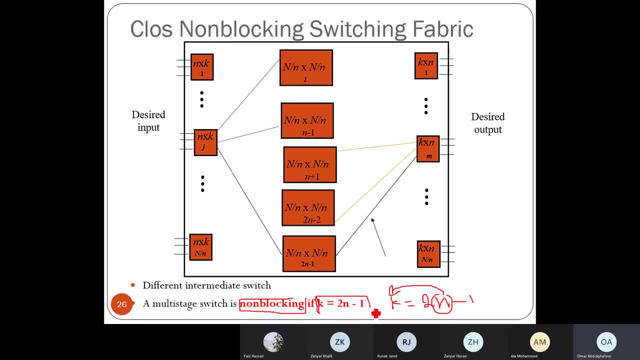 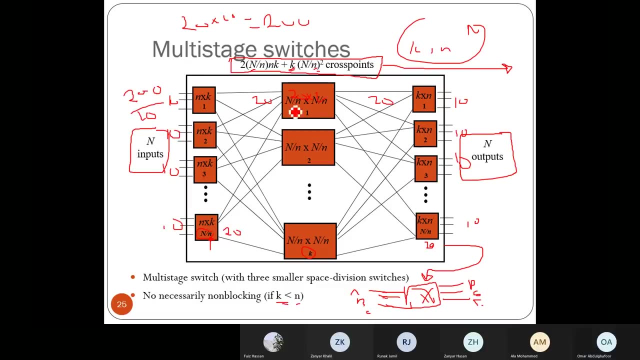 using non-blocking, then you have to take this one clause condition or clause criteria. we call it this one clause criteria or clause conditions. all right, so the way that we determine decay will be different, all right, from here n times k, all right, and here we can. you can see n times. n times k will be. 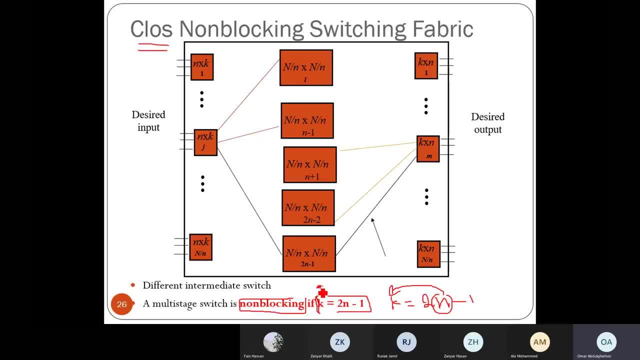 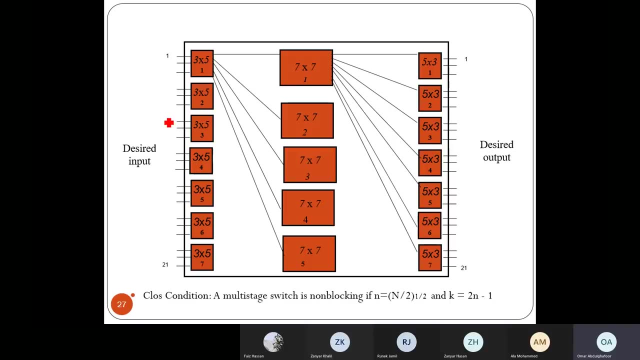 different the number of of k's, all right. number of k's will be different. if we would like to design using the clause criteria or non-blocking switching criteria, all right, non-blocking switching criteria, okay. so, for example, here we have um multi-stage switches, non-blocking if n. yeah, all right. so the small n. 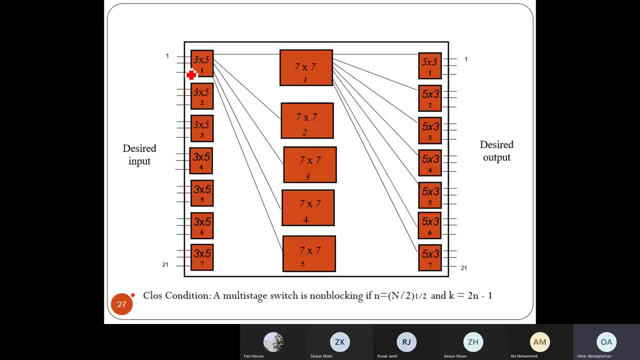 uh come. so for example, this one actually is: we have: uh, each block is three times five. and how many blocks i have? one, two, three, four, five, six and seven. so that means i have 21, all right times 21.. here i have five times three, all right. and how many block i have? one. 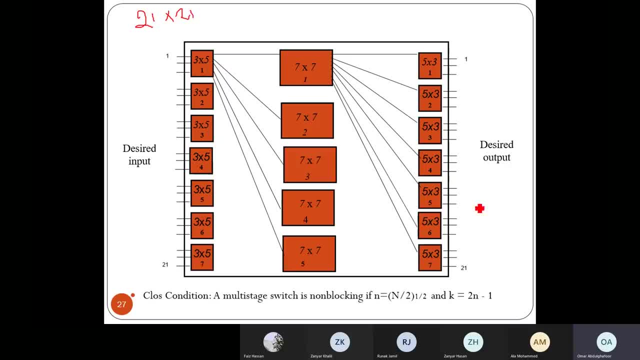 two, three, four, five, six and seven, so i have 21.. so you can see this one, the output. all right, and this is the output is: uh, is same, all right, three times five and five times three. but in between, here, since i'm i'm following, for example, the, the close columns, you'll see there's three. 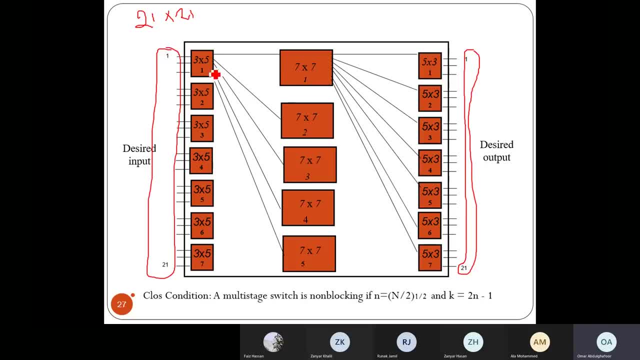 in between. here, since i'm, i'm following, for example, the close columns you can see here, for example, seven times seven. So I have one, two, three, four, five, six and seven. Then I put: here is a seven. 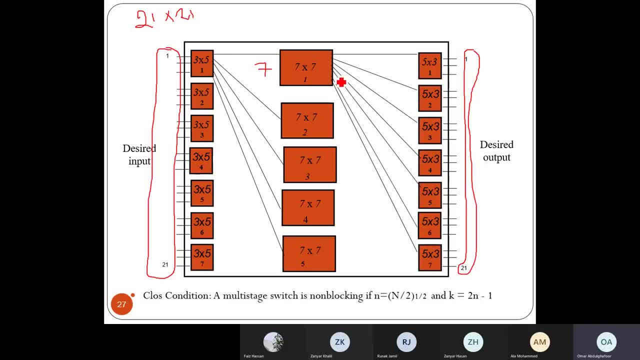 All right, and here one, two, three, four, five, six and seven. then I put: here is a seven, All right. so how many I have here? for example seven times seven and here is three times five. So that means one, two, three, four and five. 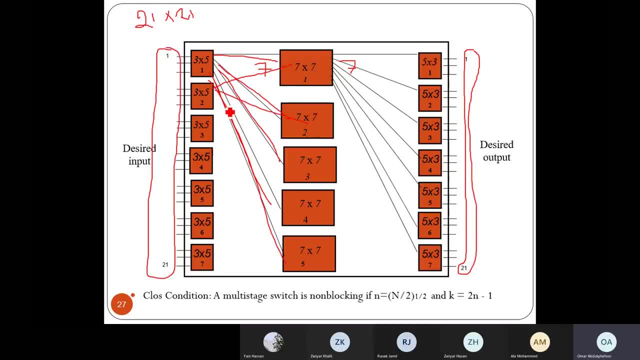 So each will be five. Here is one, two, three, four and five. But here how many output output? I have Seven, So that means from each block one, two, three, four, five, seven. I have one output to make sure that I can follow. 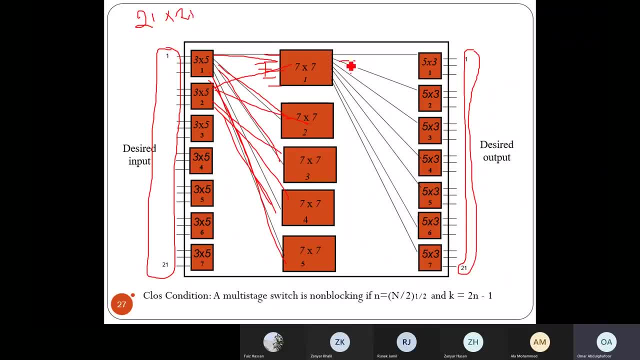 and I can fill for all the paths, And same goes for this one. Here I have seven. So how many blocks I have One, two, three, four, five, six and seven, and also got for this one: One, two, three, four, five, six and seven. 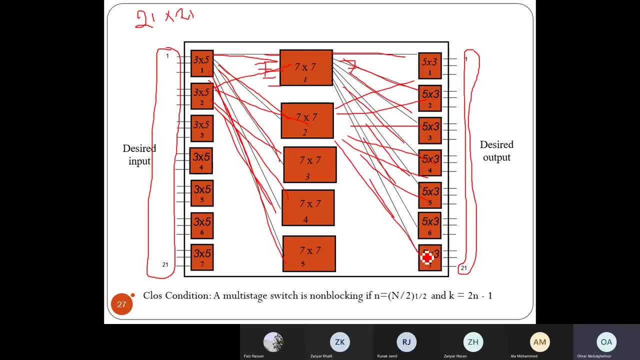 All right. So here I have one, two, three, four and five blocks. Same to this one. five blocks, All right, five blocks. and the number of output. output depend on the blocks of the first stage and the second stage, which are seven. 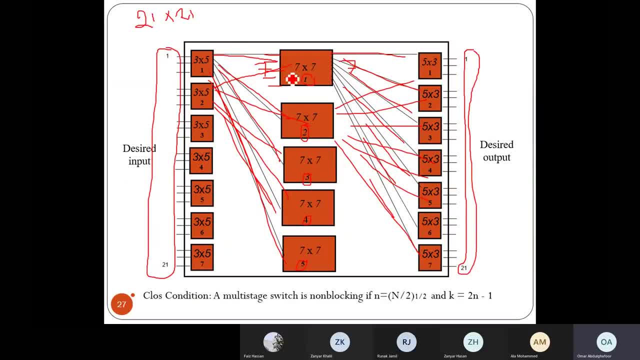 So I need to make sure this one actually has identical seven times seven or three times three or four times four. This one will be same according to the number of blocks converted later on. All right, number of blocks years and number of blocks years. 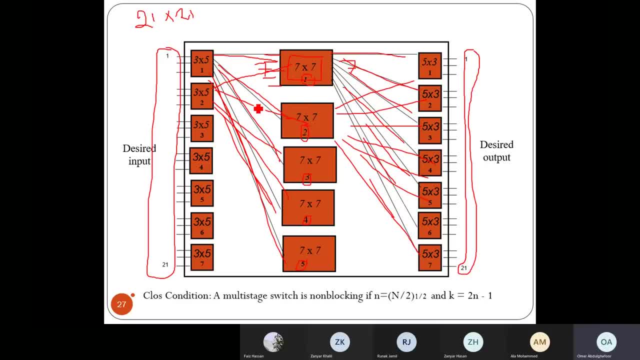 Alright. so this is actually. it's the How looks like the multistage. but if I would like to follow the clause conditions, non blocking. here, non blocking- I can say that the small N- alright, you can see here, and times K, I can determine. 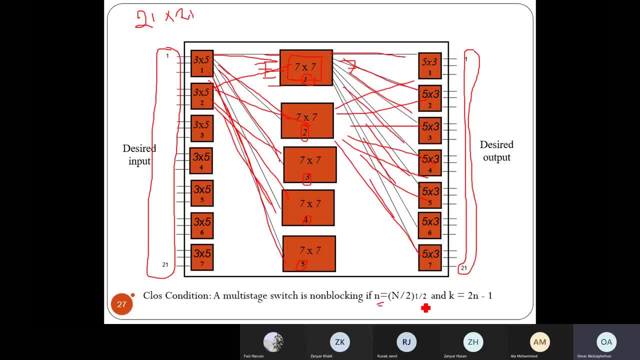 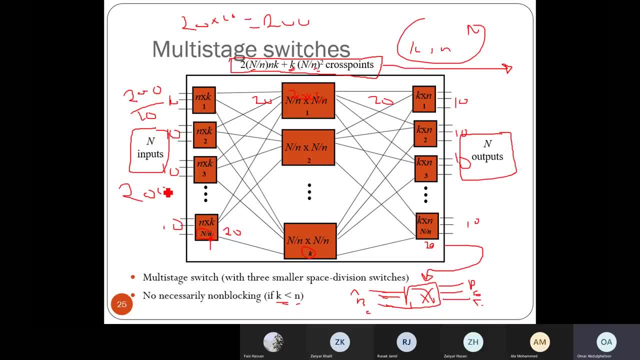 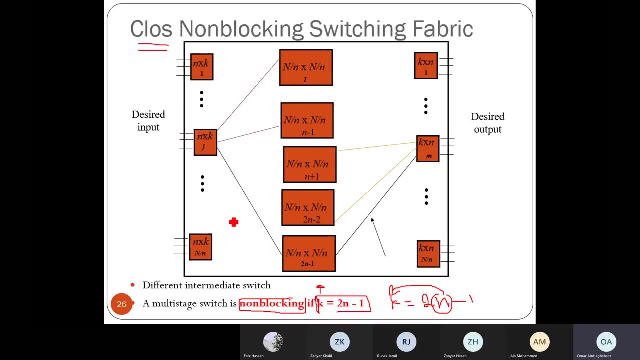 which is capital N divided by 2, half Alright. so, for example, if I said that here I can say I have 200, alright, here I have 200. and I would like to determine the small N according to clause Non blocking Switches. what I need to find here is 200. 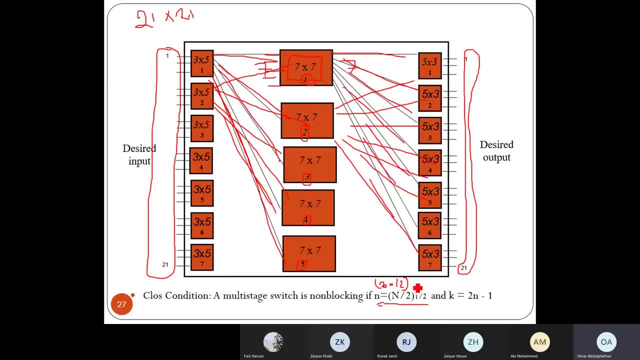 Alright, 200 divided by two, and I need to take half of this one. So what's? 200 divided by two is 20? Is the sorry? is one is 100, I'm right. So half of this one, half of this one will be. 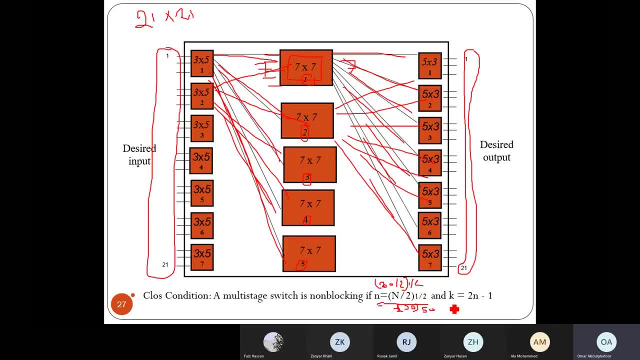 50, alright. and also I can determine K according, based on the value of of N. alright, based on the value of of N. So this one you have to Alright, you have to, what you call it, Memorize. this one actually is a small. 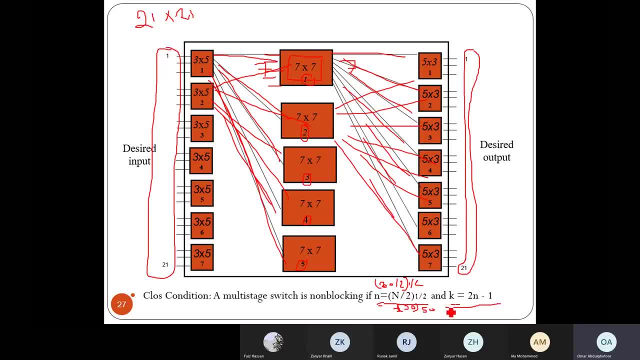 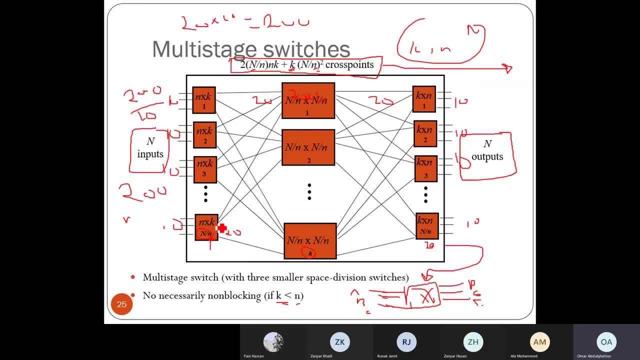 small formula. It's not, It's not difficult, But it's. it's very important in terms of in terms of design, because we have two types of design, either by using the normal one- we call the blocking scenarios, or multistage, Or if I said, for example, 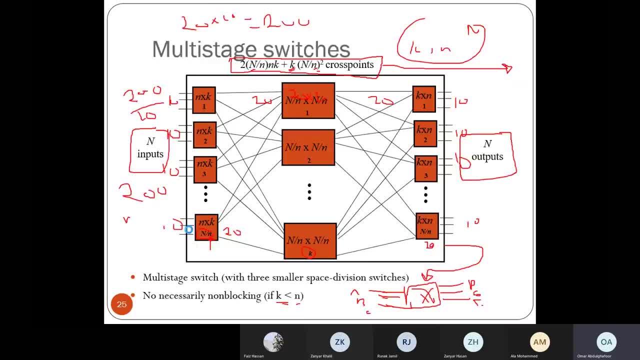 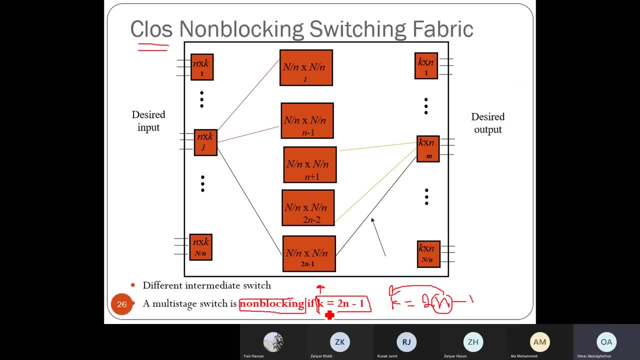 the clause criteria, redesign or design your clause criteria, then You have to fulfill these two conditions: K, two small N minus one. This one, it's provided, which is the input of of the first stage and the output of the Last stage, and also K can be determined. 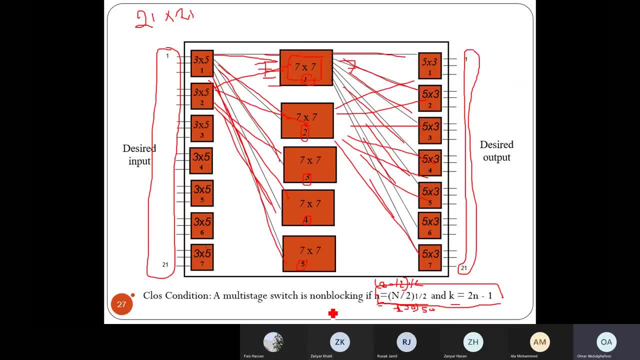 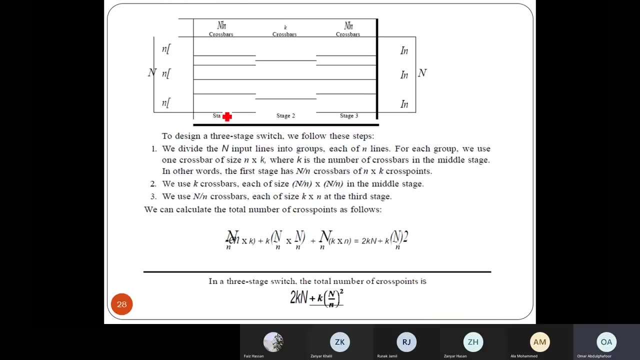 from this formula, and also small and can be determined from this condition, which is N capital divided by 2.. Half of that, Alright. So these are actually the most, the most important, alright. so, Uh, Uh, for example, here we have. 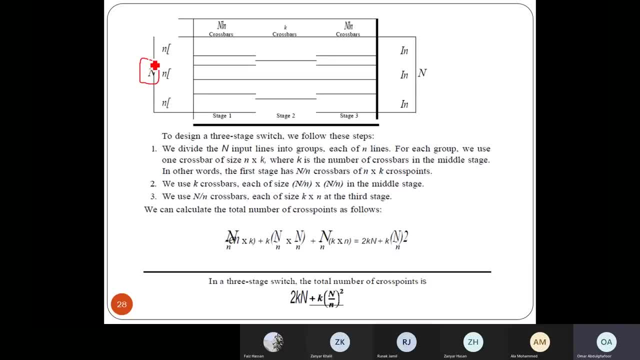 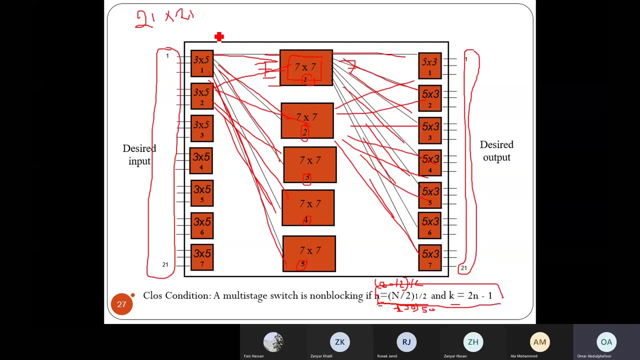 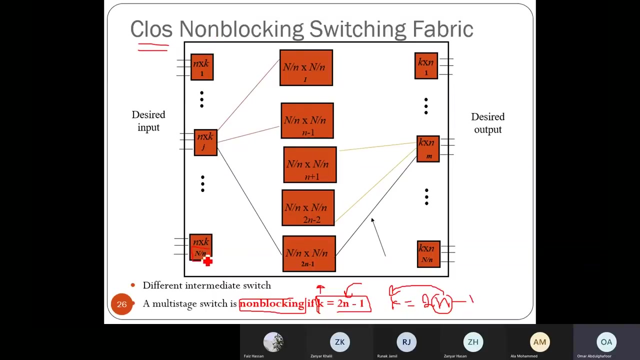 We have N capital- you can see Alright- grouped into small, small N. alright, The N capital actually is divided into small, small N, divided on how many blocks we have. And here we have N capital divided by N crossbars. You can see Here This one divided by this one. 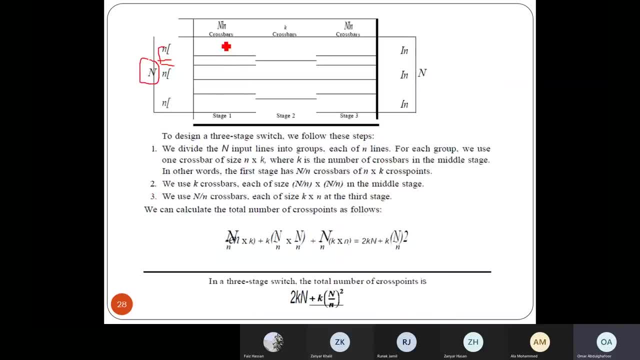 OK, so it depends. So I can determine stage one. So in stage two we have K crossbars, Alright, K crossbar, which is here we have N times, K Alright. so K crossbar, K crossbar, and here we have. 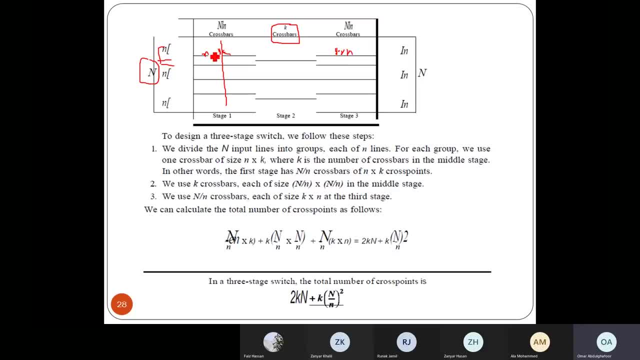 K times N, because we said N and N here must be same, and for sure the total capital N and capital N will be same. Alright, so here we have N capital divided by N crossbar, Here we have K crossbar and here we have N divided by capital. 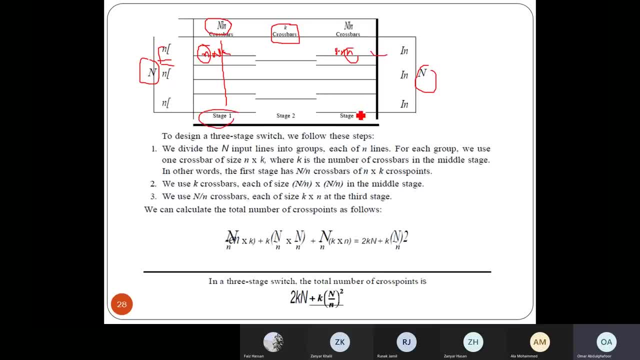 and divided by small N crossbar. That means stage one and stage two, same and in between depend on the case. One minute, guys. I need to Recharge my laptops. One minute, please. One minute, please. Alright, then, to design a three stages switches, for sure we can increase, actually, and 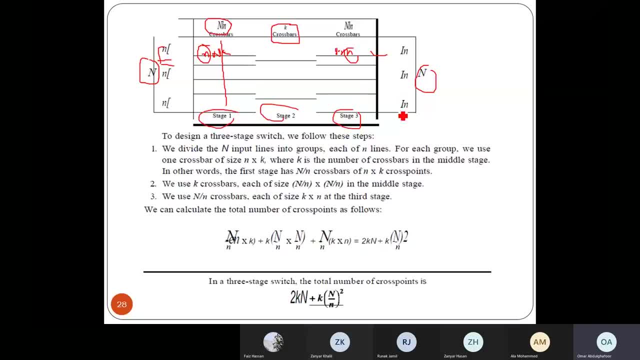 As I mentioned, the design can start by very simple design and we can have advice, really advanced design and complicated design. But this one actually it's similar to. I mean, the design of the switching is similar to the, the, what you call it, The concept of, of the design of the switch. 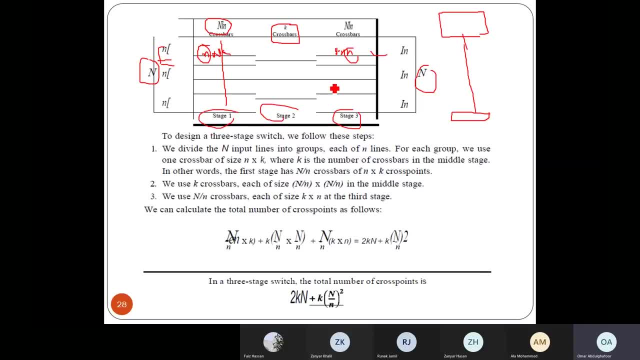 Of multiplexer. alright, so in microprocessor and in digital technologies, that that you have done, Then you can use- I mean, different type of multiplexers with input, output in order to link between the two different stages. alright, so same. I mean concept, almost same concept here. 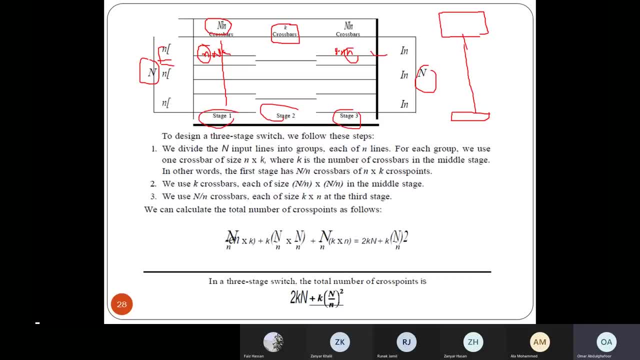 But in here, in this case, we have this: switches, alright, in terms of, let's say, flip flop, so, or, or what you call it, For the registers, So anyway. so we divide the input lines into groups, each of n lines. this one, alright. so for each group we use one crossbar size. this, this is the size, alright, crossbar, this is this, this one. 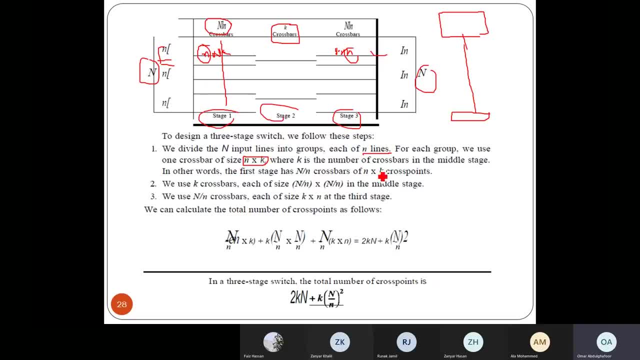 Alright, this is the size of crossbar. Well case, the number of crossbars in the middle, In the middle stage. alright, so another world, the first stage, has This one, capital divided by n crossbar of n times n cross points. all right, this one, this is, you can see, this is. 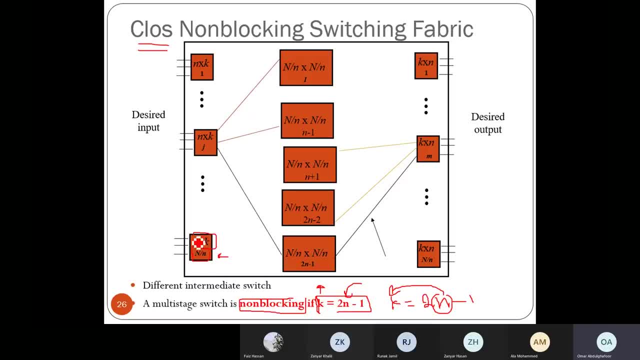 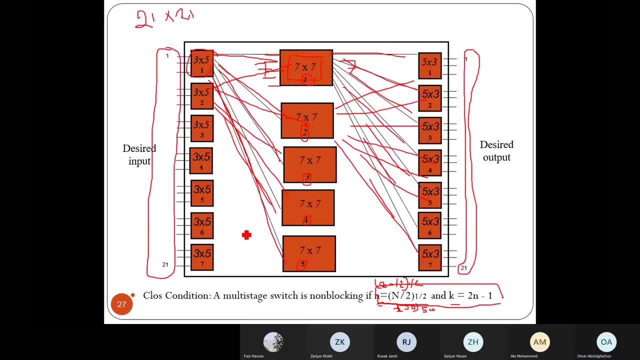 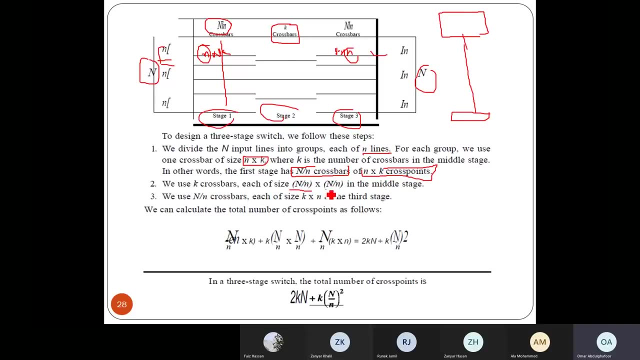 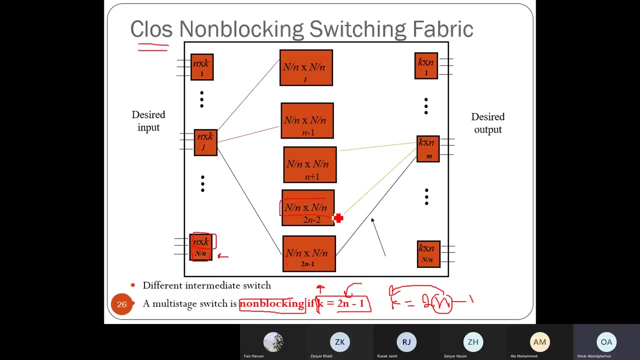 crossbar of what's n times k. all right, so this is input output: how many blocks we have and capital divided by small, n and k crossbar each size. is this one the size and capital divided by n? and capital divide by in the middle stage? this one, all right, this one n. capital divided by small. 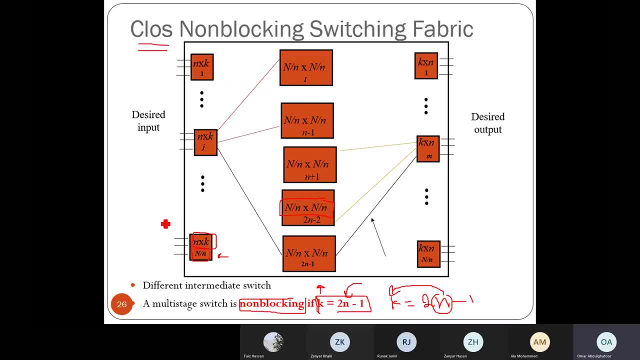 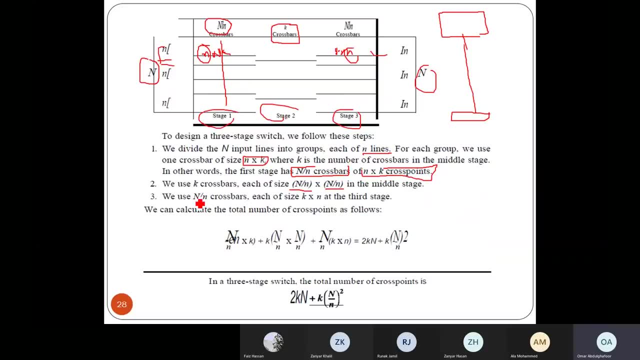 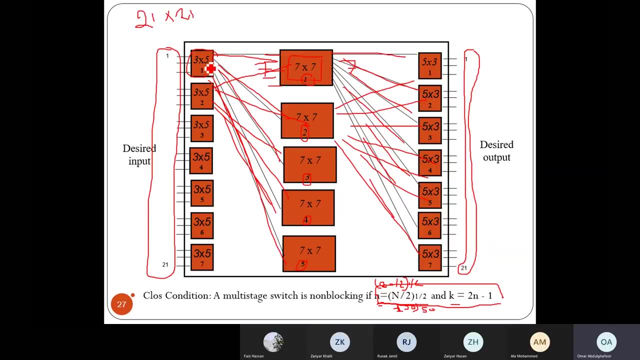 n the size, all right. so whatever we have, whatever small hand we have, we can, all right. and what else? we use n over n across bar, each size, k over n. on the third state, which is, i mean, same, all right, but this one n times k, this one k times n. all right, because we need n here. 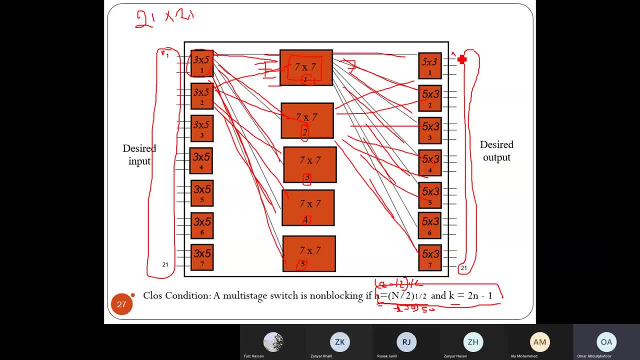 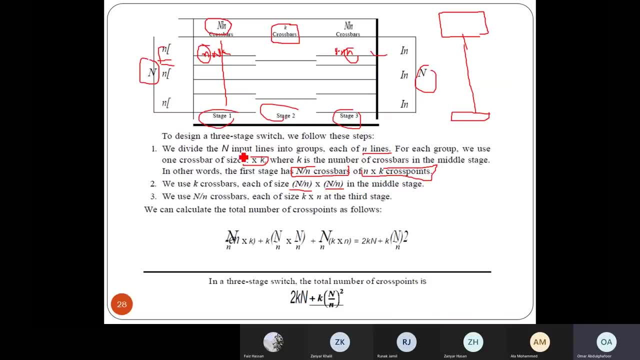 and n here, since we have n inputs, we have n outputs, all together will be n capital and all together will be n capital. same here we said that the n inputs, we divide n input, which is the capital, into groups of each n lines. all right, each n lines and the size will be in terms of 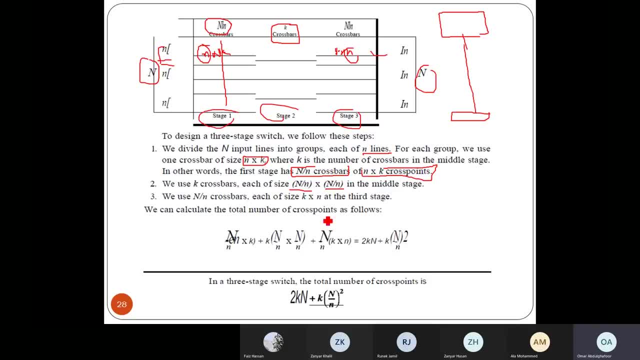 crossbar and times k, so we can calculate the total number. this one, the total number, all right, total number in terms of: if i ask for complexity, determine the complexity of the crossbar and and so on and so forth, then this one will be the total uh number of cross, of cross point 2 k. 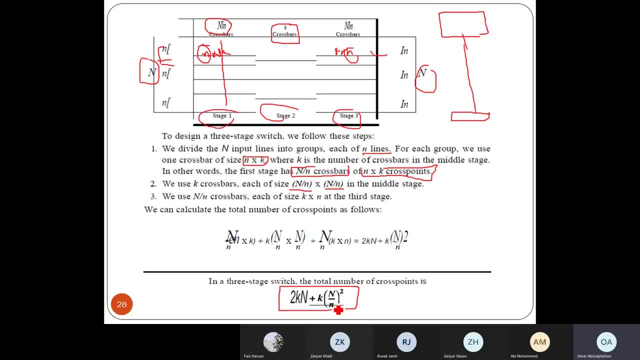 capital n plus k, n over n. capital over n small, all square. so this one in terms of the com complexity, all right. complexity, or computational complexity. computational complexity- and you can compare for any other technique, like like crossbar, the one that we have used for the grid- all right, this one. 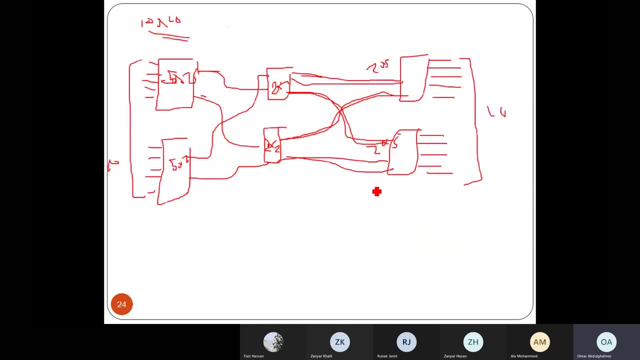 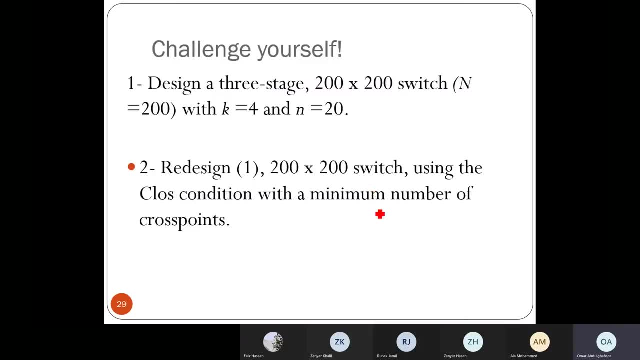 the one that we use for the grid- and multi-stage and how many stage we have. so you can, i mean you can- compare, all right. so here we have some, some, some examples. for example: design a three stage. design a three stage: 200 time, 200 switch- all right, here is n capital provided 200, with k equal, 4- all right, and n- equal. 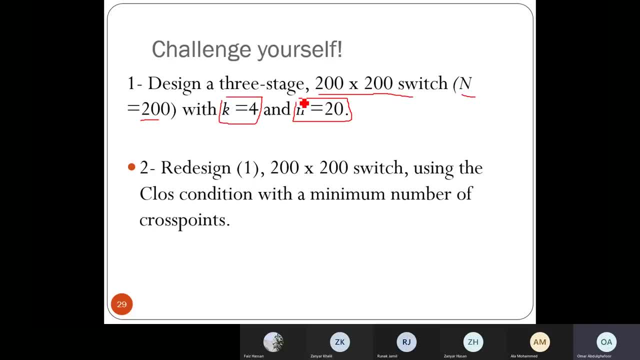 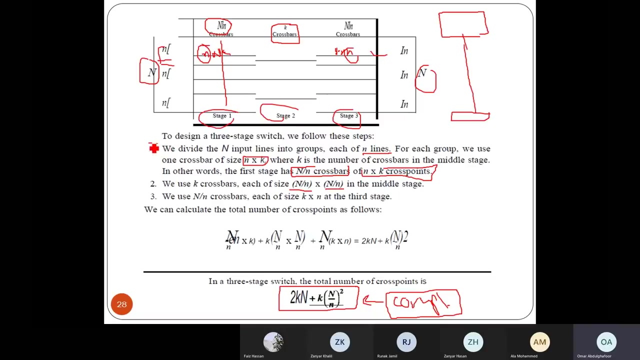 equal 20, all right, n equal 20.. so, so, how we can, how we can solve this one, uh guys, so let's um the. the procedure actually is provided here. you can see number one, all right. number two and number number three. so number one, we divide n on both line into groups. 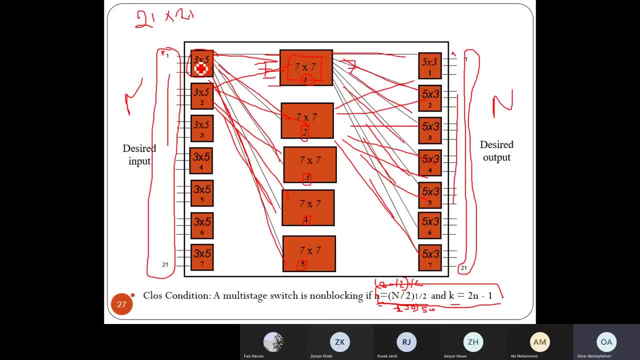 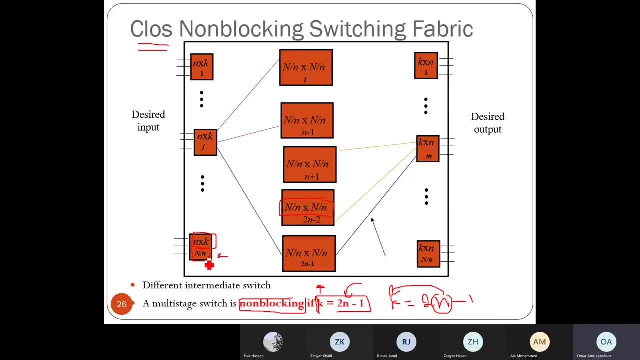 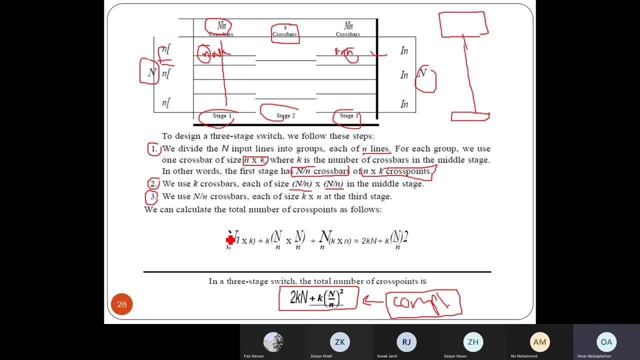 so each n lines, all right. so into groups. this one groups: group one, two, three, four, five, six, seven, for example. so what's the types of groups? this one: we start from one until n capital divided by smaller. so for this one, if i would like to follow this, the point number one: 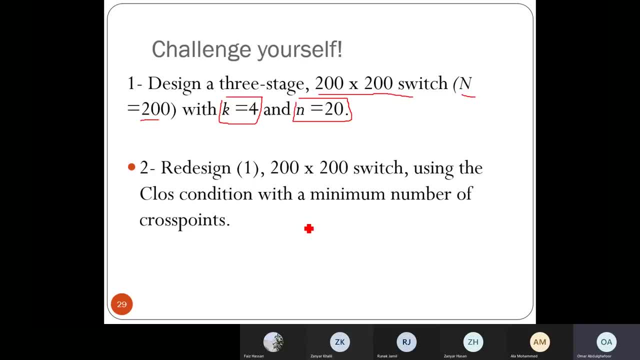 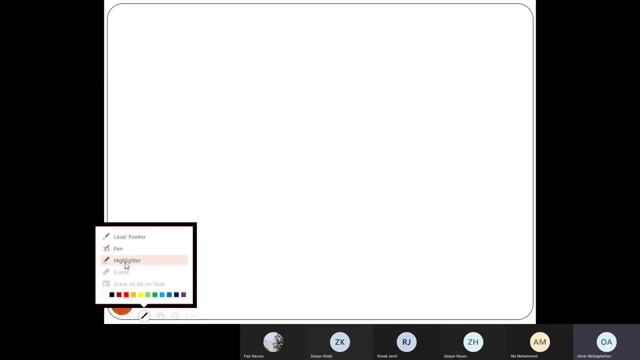 so i need to make a groups. come right, let me, all right, keep this one, okay. so, for example, here i have 200 and small and easy 20.. all right, 220. so if i would like to set the inputs, all right, group one, two, until until i reach to. 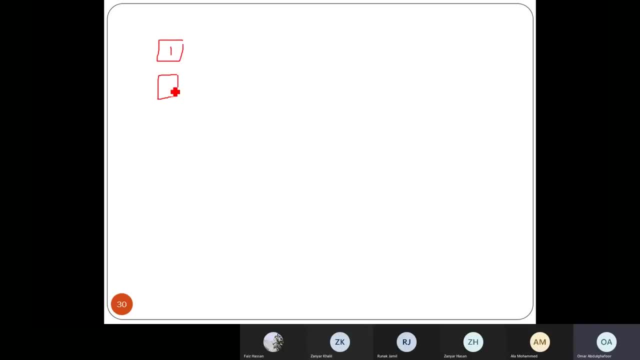 n capital divided by n control group, one until until i reach to N capital divided by N. So what is N capital? N capital actually is 200.. 200 divided by 20.. Then what I have, 10. Am I right? So I supposed to have here is 10.. From 1 to 10.. Then each one how many input I have. 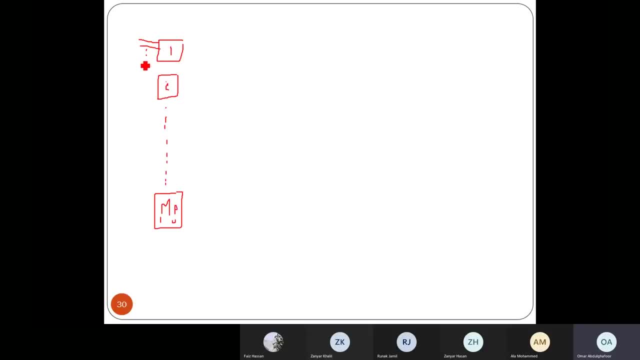 100.. So 1,, 2, until 20.. Am I right? Then 20, 20 times 10 will be 200. So all together here will be 200.. So I divide it into how many crossbar. 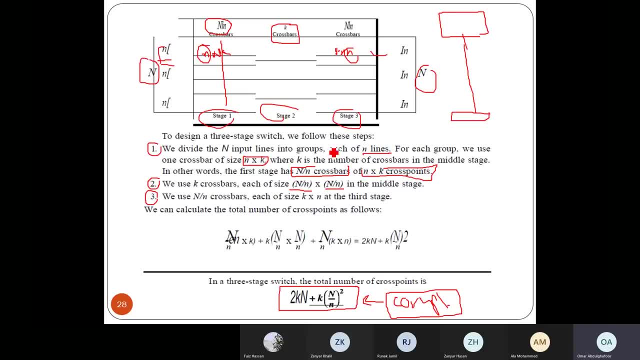 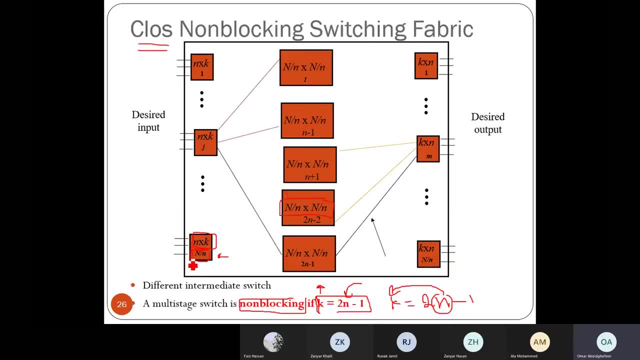 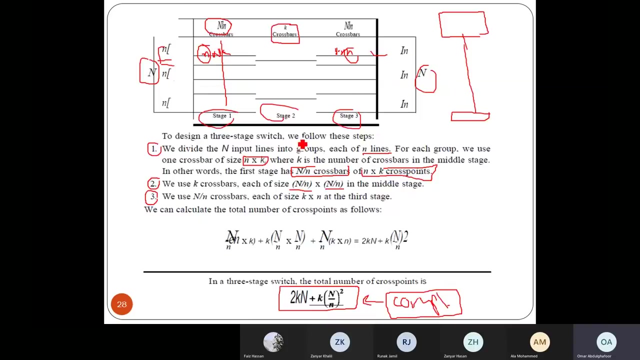 This one, how many crossbar You can see Where is this one: N capital divided by N. N capital divided by N small. So my N capital is 200 divided by 20.. Then will be 10. So I have from 1 until I reach 10.. So here will be N times K. So it's very simple, this one, because it's provided. 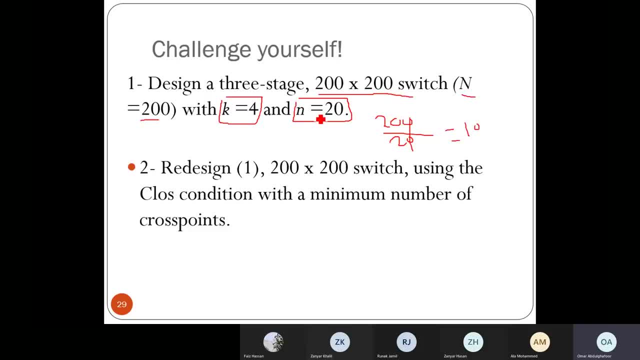 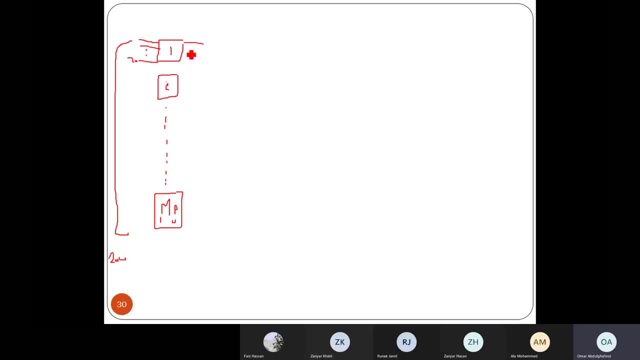 So N times K, which is 20 times 4.. All right, 20 times 4.. So that means I have: here is 20.. All right, And here is 4.. 1,, 2,, 3, and 4.. 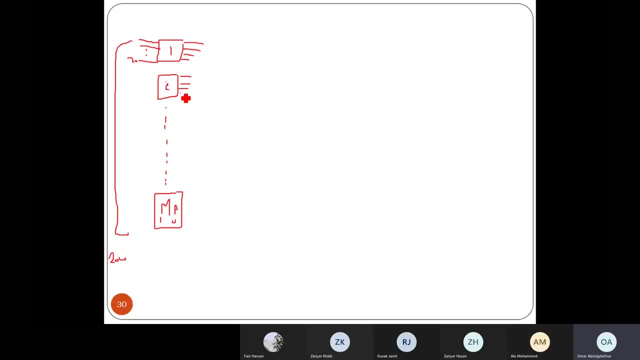 All right, 1,, 2,, 3, and 4.. Until I reach 1,, 2,, 3, and 4.. So in between, here I have how many I have: 20.. All right, 20.. 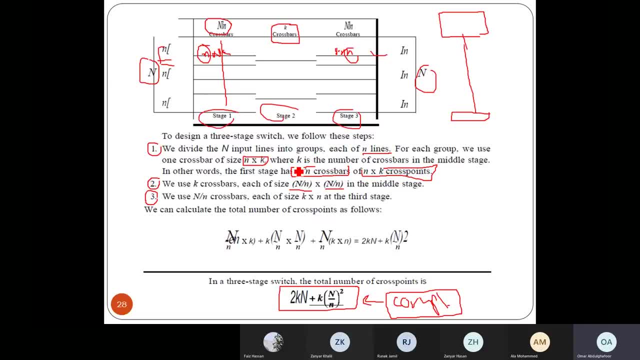 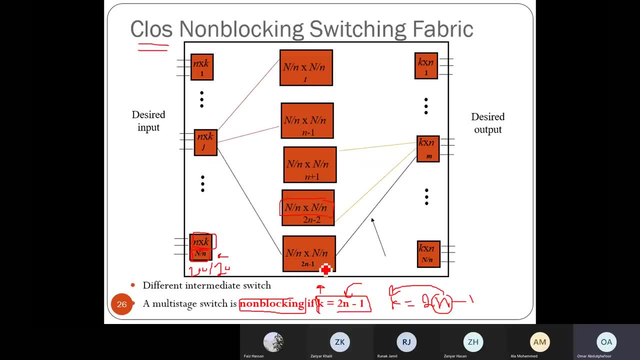 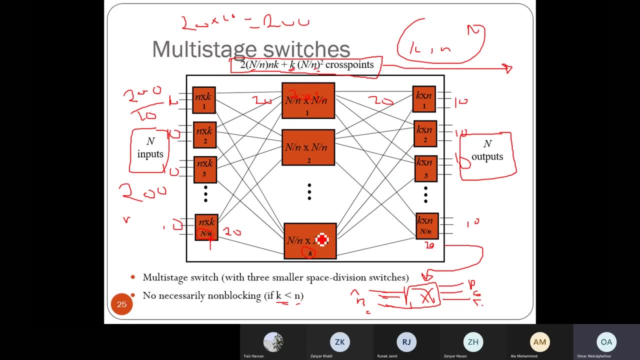 This one, the stages. you can see. This one: All right, Until 2 and minus 1.. For you, For example, All right. Or this one is the cross, This one Until K. All right, 1 until K. All right. So 1 until K. So what's the value of K? 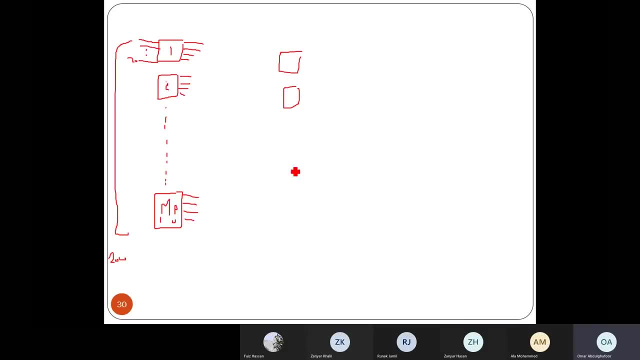 What's the value of K Here is 4.. Then I 1,, 2,, 3, and 4. And each the input. how many inputs? N capital divided by small, n. So that means 20.. All right, So 20 times 20.. All right, 1,, 20,, 1.. 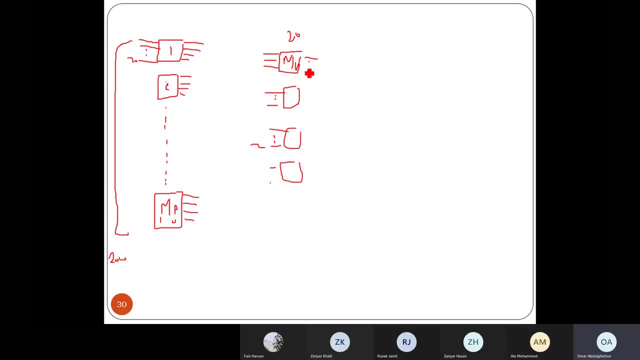 21,, 20.. And here also is 1., 21,, 20.. So here you can see is 20. Times 4.. I said the last stage, which is this one. You can see, this one is: 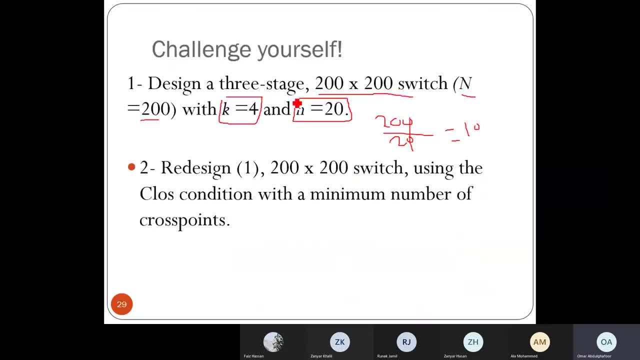 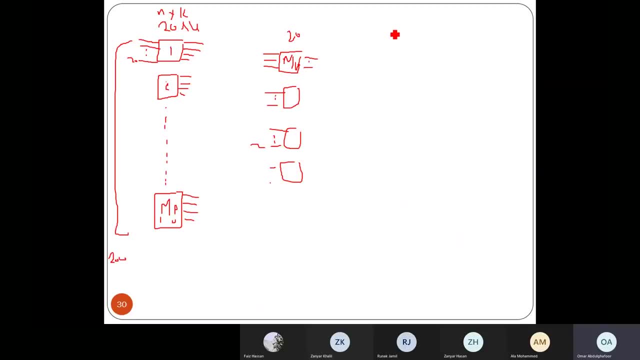 N times K, All right. N, which is 20 times K 4. This one N times K, All right. And in the last stage, what I need to do, I need to say K times N, Because N. 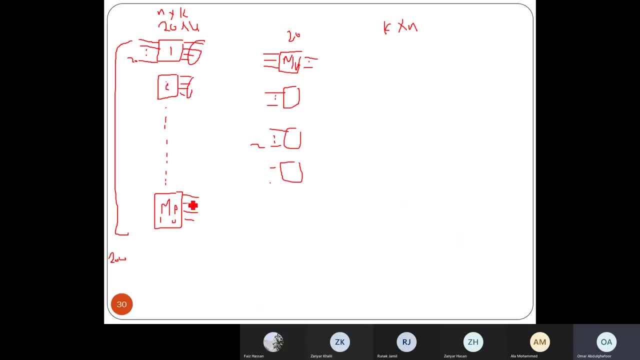 must be same, n, n, until the last one will be n and the total capital n will be same. so here i have 1, 2, 3 and 4, the size of each, which is n capital divided by small n, so 20 times 20. so in this case, 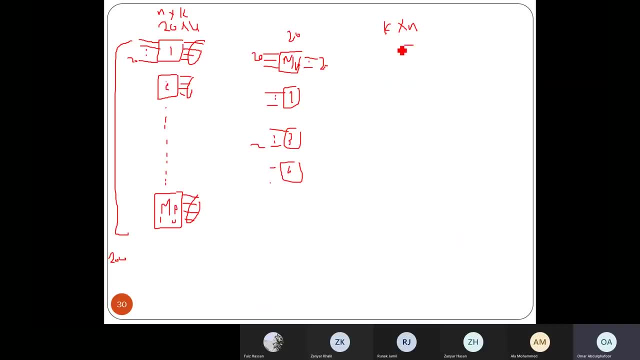 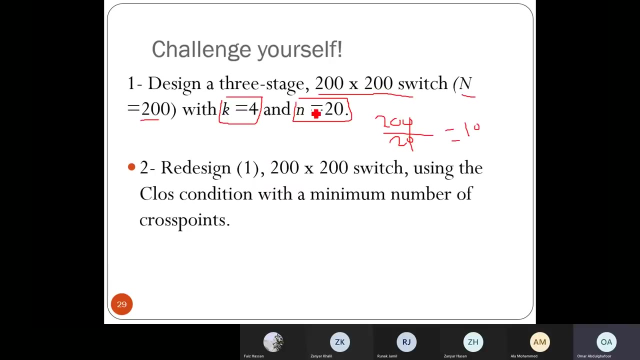 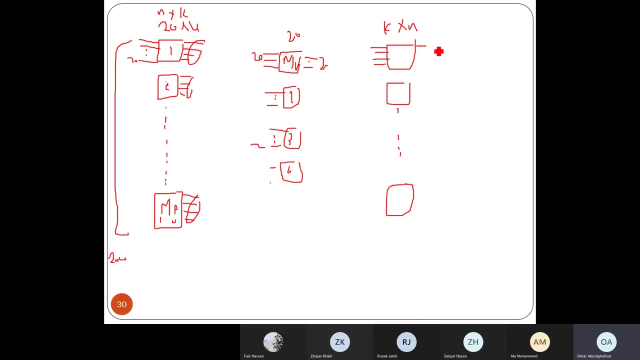 what's the value of uh. the blocks actually will be will be same, number of cross bar will be same, which is 10, and the size is k times uh times n, which is 4 times 20. all right, so that mean i have 1, 2, 3 and 4, and here i have all right. 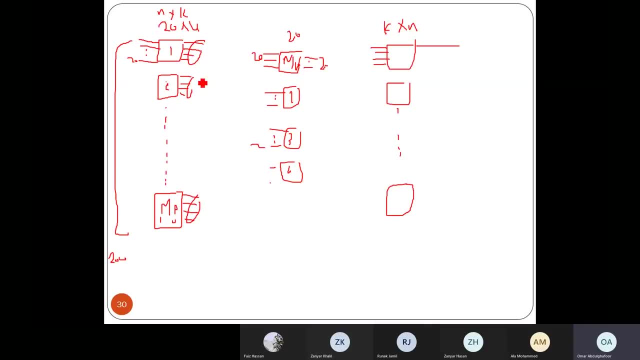 20, all right, 20 until i reach to the block 10, which is 20. so all all together, this one will be 200 and all together, this one will be 200 and this one, for example, one, two, three and four, and comes and comes and all together can be all connected. 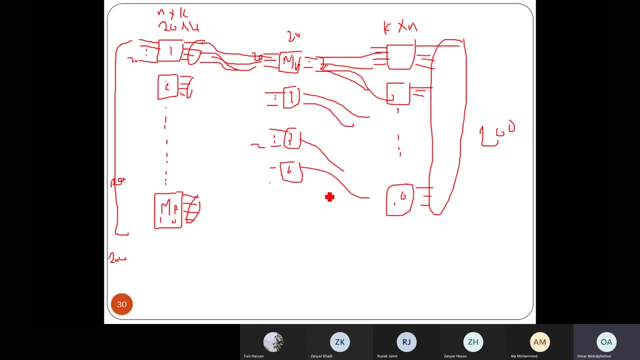 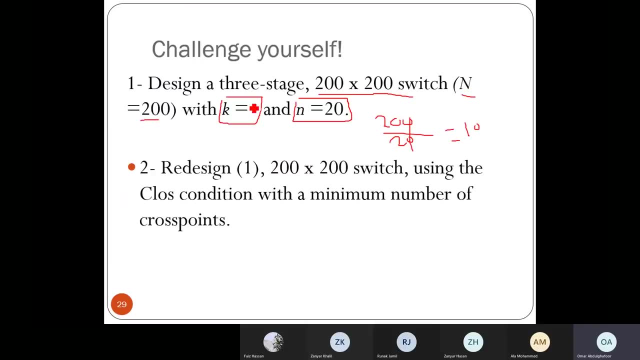 all right connected to this one and that one and that one and this one and that one and this one and that one and this one, and from here we can draw a multi-stage circuit switching for this, uh question, for example, design: actually this one, actually this exercise. 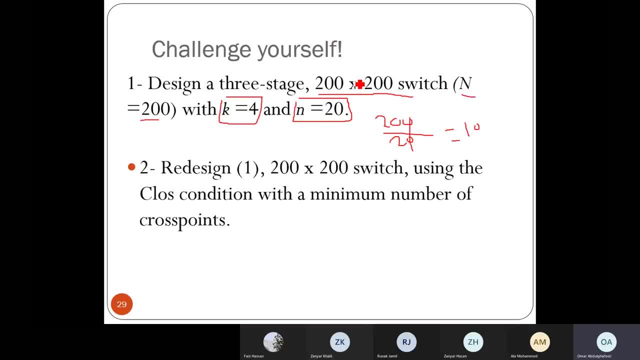 we're going to solve it in in details again, in in in our tutorial class. next class will be at auk for more, for more details and better understanding. but, um, here put it, just challenge yourself once. i mean after this class. you can try your best. you can try your best so. 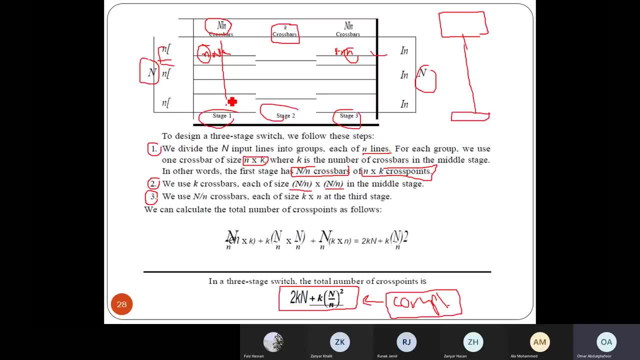 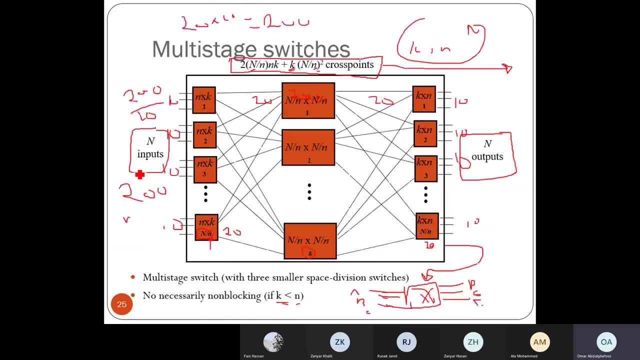 so i'm here putting: just challenge yourself once, i mean after this class, you can try your best. you can try your best so you can try your best on and you can follow them. this, this algorithm, all right, and the blocks here provided all right. for example, here, how many, how many blocks i need to use this one? 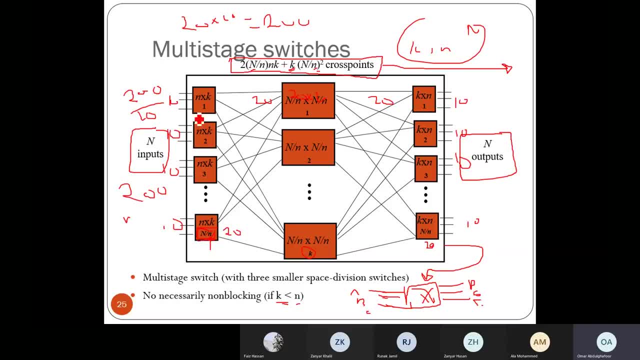 n capital divided by small n and n times k. so depend on the value of n and k. so this one, actually we have n capital divided by small, n times n capital divided by small n. for how many cross bar i have i have? until i reach k, all right, and this one will be the other way. we have n times. 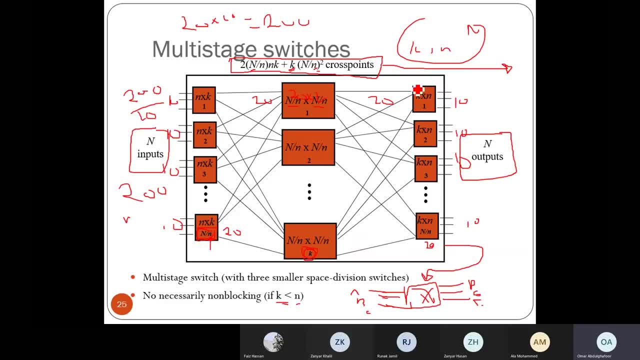 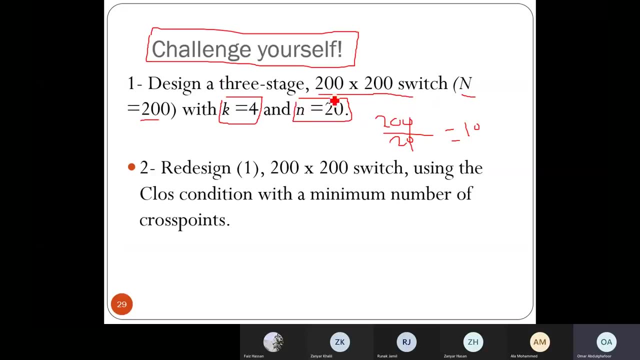 k. here we have k times n and the number of blocks and the number of cross cross points. we have same, all right. and capital divided by n, all right. so then for this one design, a three stage, 200 times 200. so that means, when i said 200 times 200, that means this one will be. 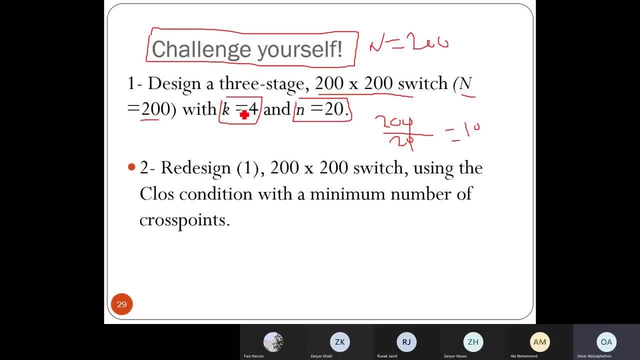 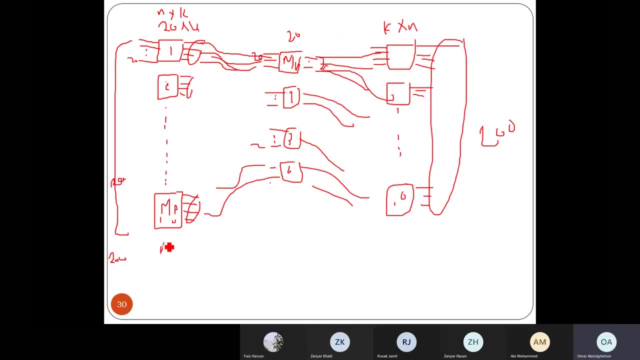 and capital 200. all right, so depend on the arrangement: k equal 4 and n equal 20. from k and n. i can design. all right from k and n. i can design because, because this one actually will be one, two until i reach n capital divided by smaller and this one. 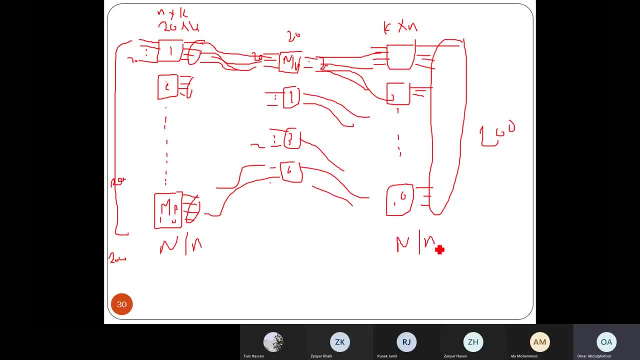 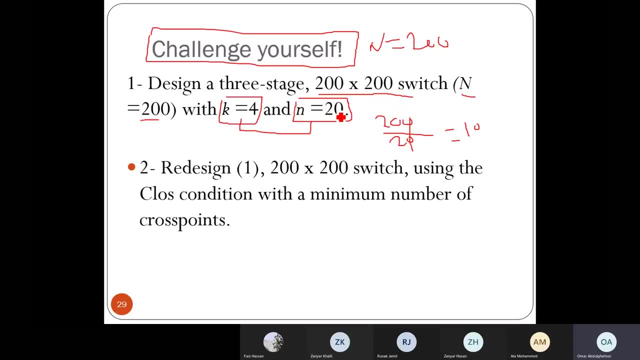 one, two until i reach n capital divided by smaller. so n capital is provided 20 and small is 10, so k is divided by 20, that means this one will be 10.. all right, this one will be will be 10.. and for sure, n is 20. all right, actually it's no need to provide, for example, and series 20.. the 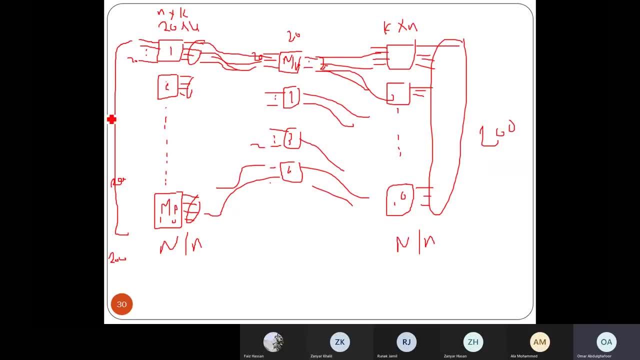 reason why? because if i have 10 blocks here and i have all together 200 inputs, so that means for sure, each block will be 20 inputs. so 20, 20, 20 times 10, all right, 20 times 10 will be 200.. all right, so for sure, this one will be. for sure, this one will be 20 for. 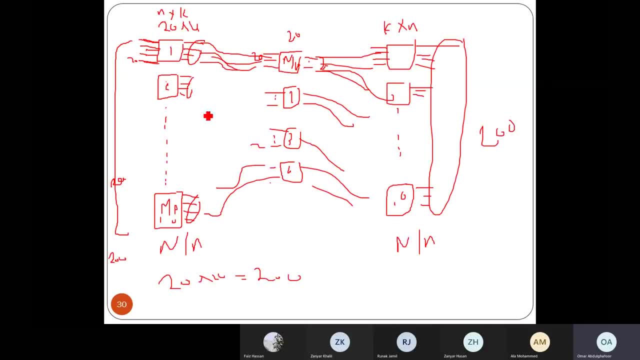 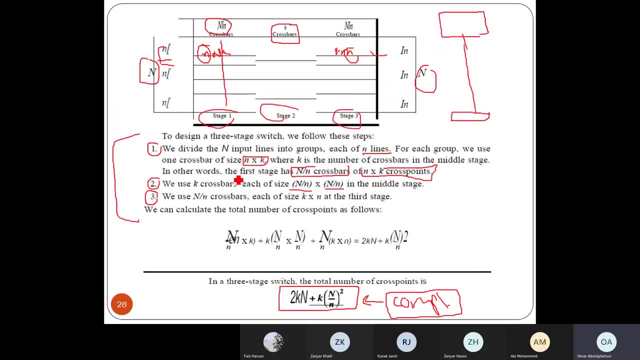 each block and 4k is provided. is four, then this one will generate 4. this won't generate 4 until this wanted it. four and for the middle stage. all right, you can see, at middle stage we have um and capital divided by n times and capital divided by by small n, which is 20 times 20.. All. 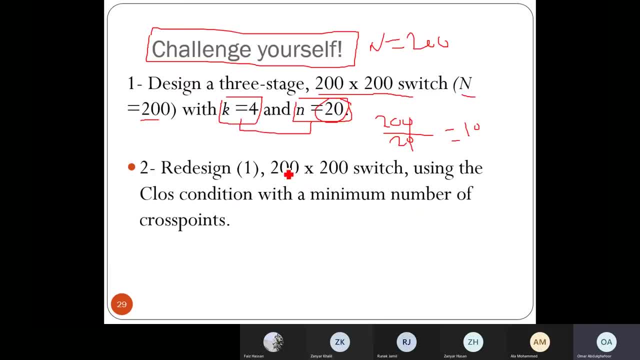 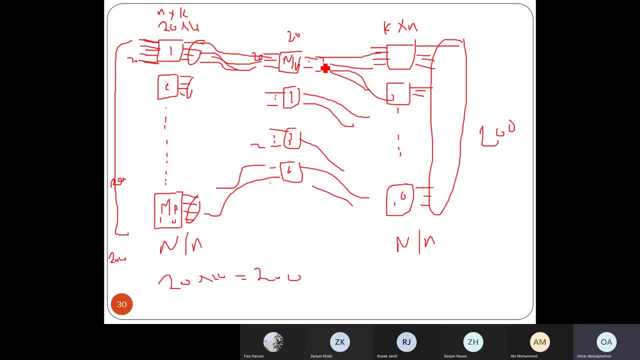 right how many blocks i have have. all right, so I have until I reach K. all right, which is four. so that means one, two, three, four each 20 times 20. all right, each 20 times 20. and the last stage, which is the opposite of the first. 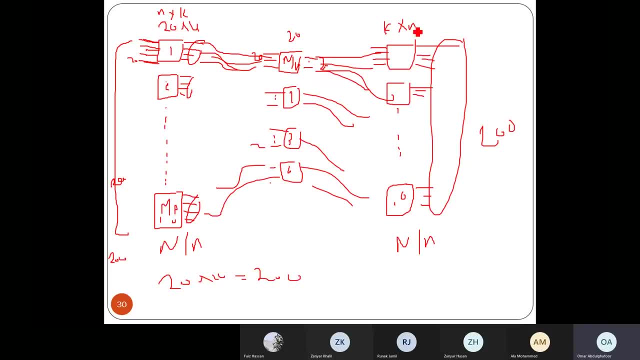 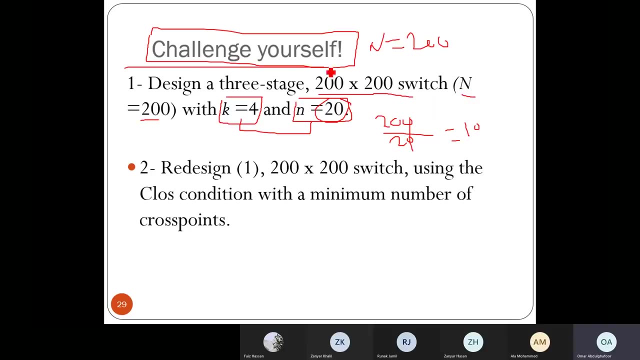 so we have 20 times n times K. here we have K times n, so 20 times 4. so we have 4 times times 20, because I need to make sure that the output stage will be same at the uh output stage. all right, guys, this one is clear. guys for you, this uh, this question, because you're going to 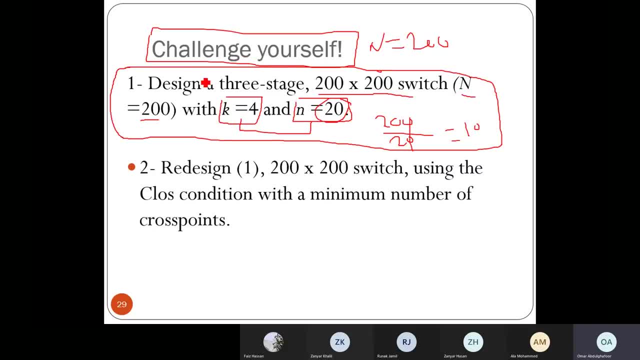 solve it after the class and also in coming tutorial we're going to discuss it in in details. we're going to draw the blocks in in details again. all right. so if I would like to redesign, all right, if you remember I I keep mentioned that and in the question. maybe I ask you to. 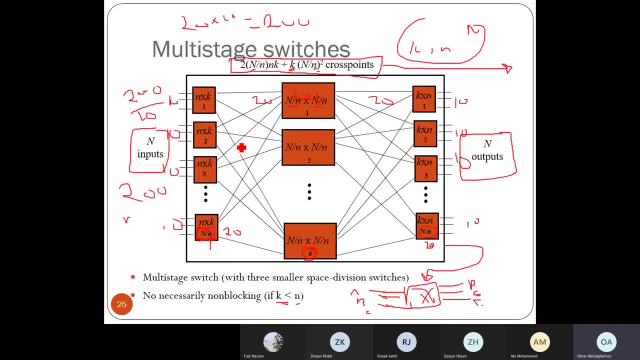 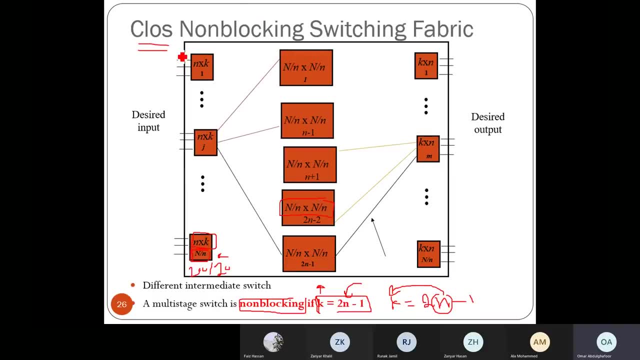 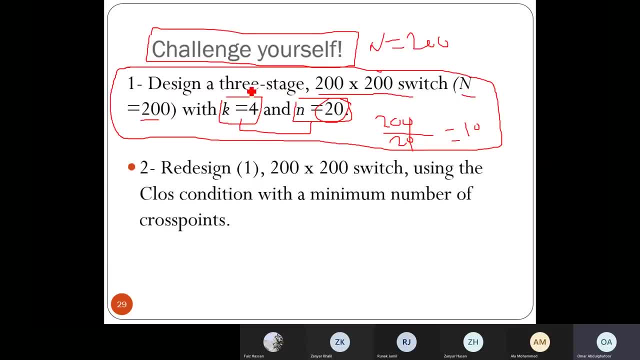 design three stage. that means this one is a multi-stage, all right, normal multi-stage. and in two i ask you redesign one. so that means redesign this one, all right. two times 200, 200 times 200, switch using the close condition with a minimum number of cross point. so that means: 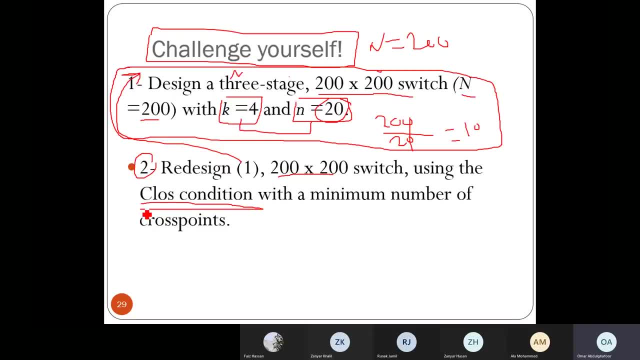 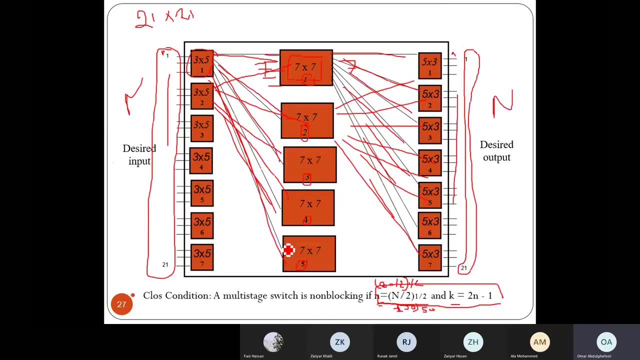 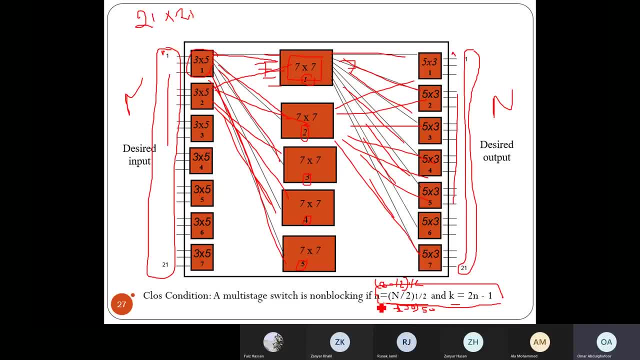 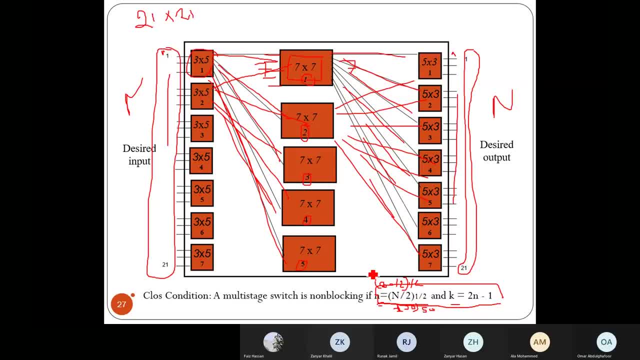 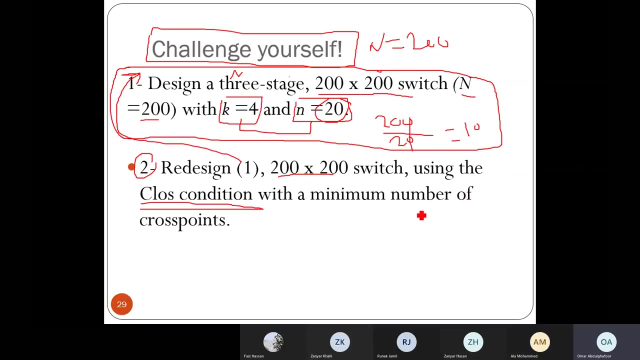 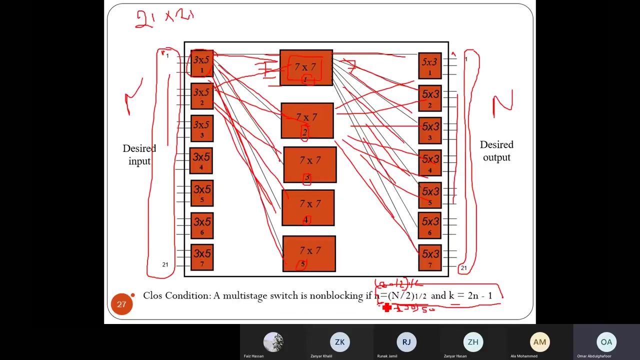 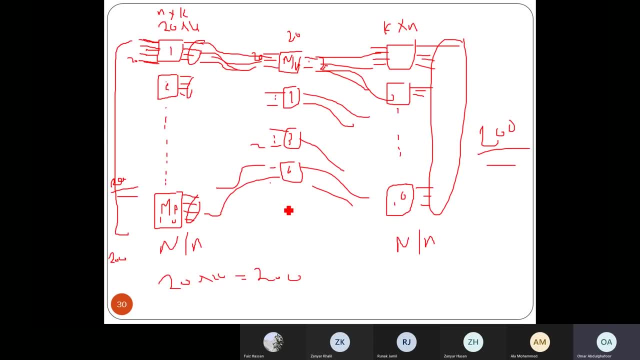 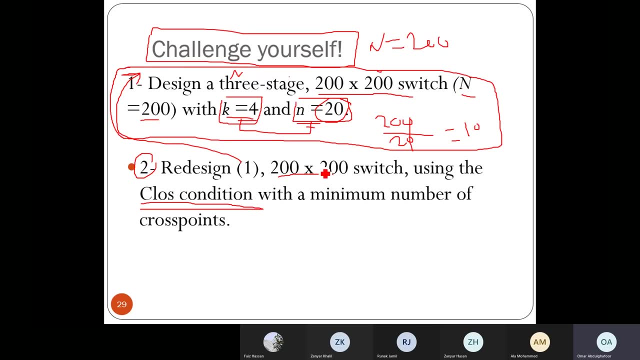 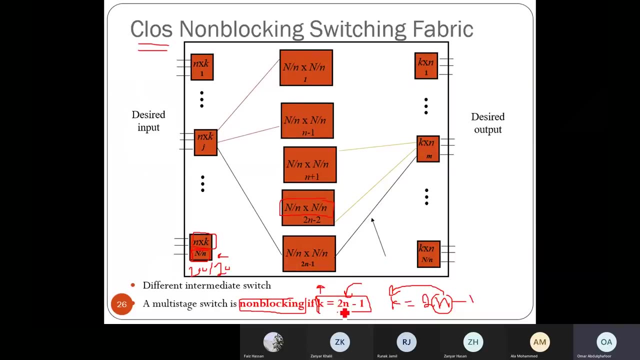 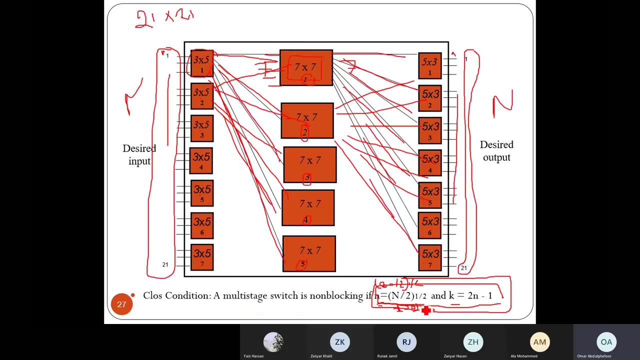 condition here in order so you can see the difference between between this one and this one. this one actually is provided. k and n. here i don't provide any k and n because k and n we have to determine according to the, according to the clause clause condition, k can be determined from 2n minus 1 if n small n is provided. if not provided, we can determine from this uh condition, this one we call the clause criteria. all right, 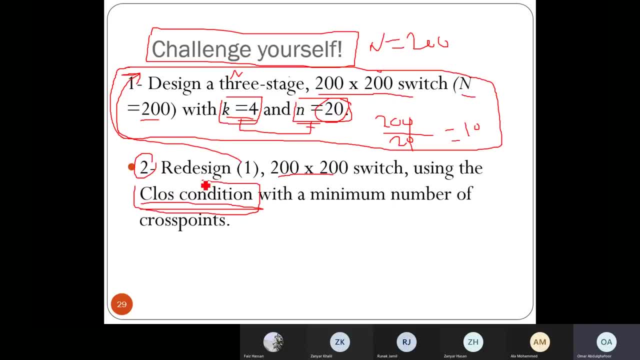 clause criteria or clause condition, or sometimes we call it non-blocking, non-blocking condition. so same procedure, same procedure that we have followed in order to design this multi-stage. we have to redesign, but in using clause condition, we have to determine both k and n, and after that, 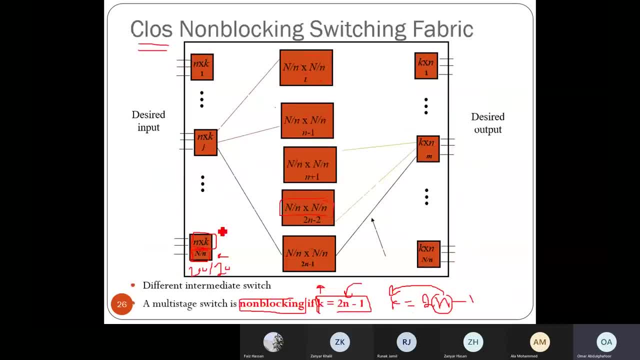 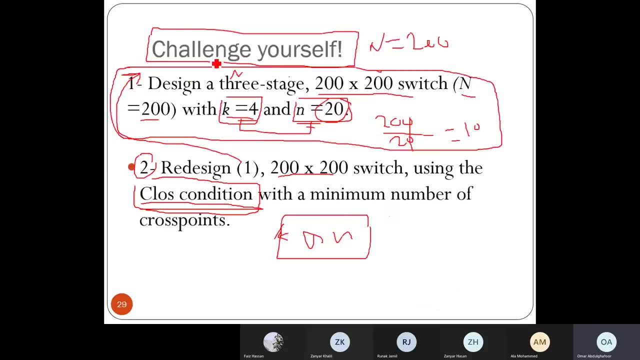 simply, we can follow the steps here. all right, same one, two, uh, because here you can see n capital divided by and here, for example, two small n minus one and n capital divided by by small n. all right, so this one actually is: challenge yourself. um, you have to challenge yourself until 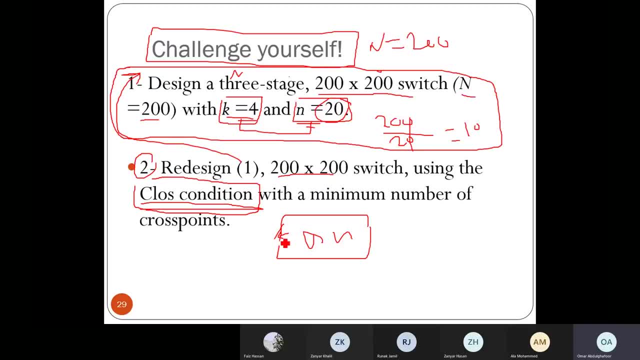 the next um the next class. again, guys. next class will be at at a uk campus at in the morning, 9 am, or if you would like to start by 9: 30, we can start 9: 9: 30, but it's very important. 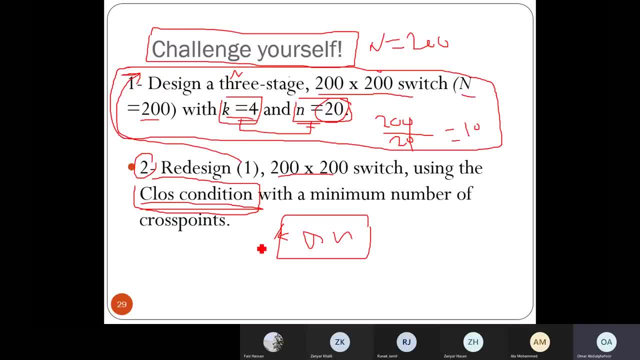 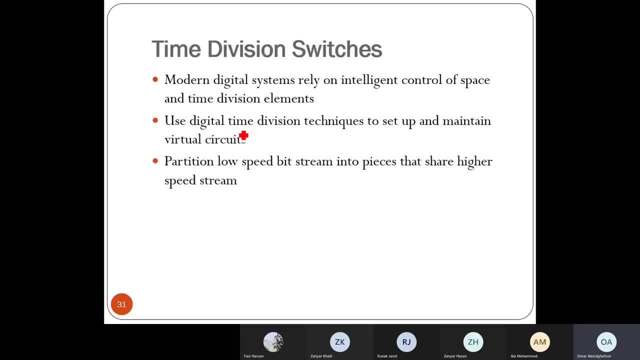 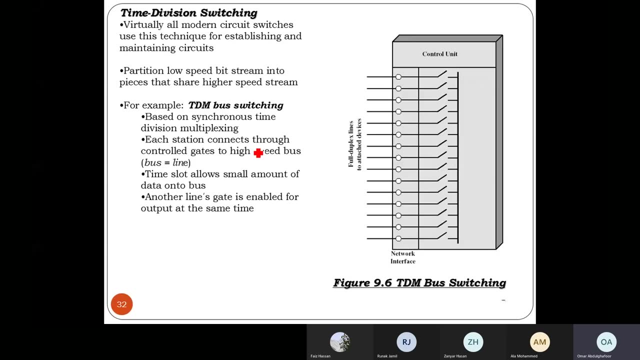 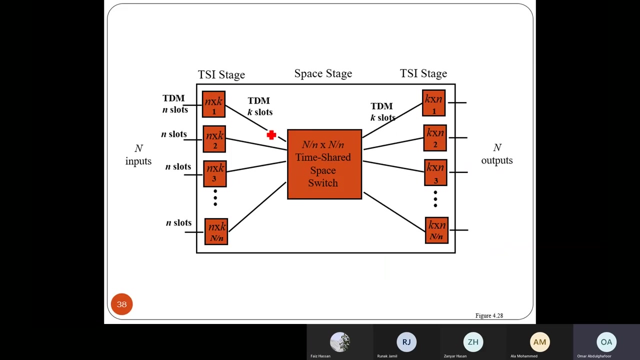 to to make yourself available for better understanding again, guys. all right, so i will stop here, guys, as i, as i mentioned, all right, and we will continue by next class at a uk. we can i mean explain for the time division, i mean the, the multiplexing. 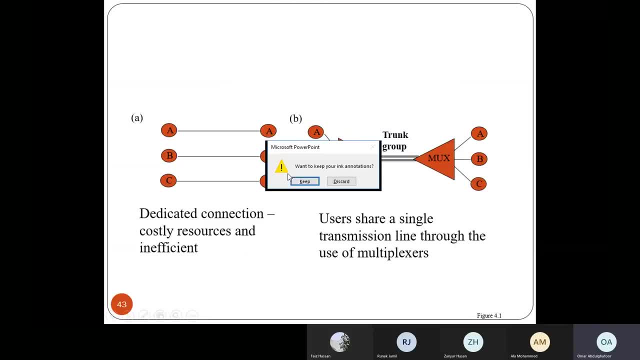 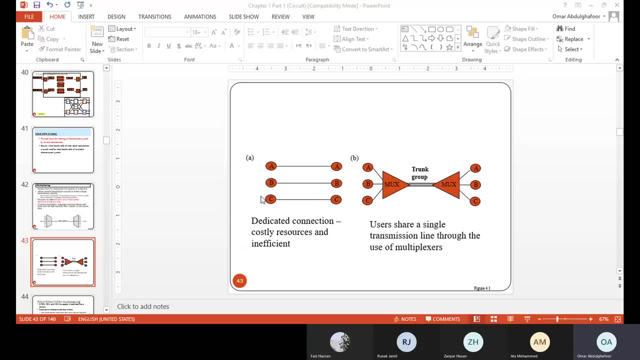 and after that we will have some, some design uh exercises. okay, guys. so, um, i hope that you can. you can join uh next class at a uk campus. i will make an announcement and again, it's um, it's compulsory actually, guys, to to make yourself available at campus because this course should be, i mean, available for uh face to face. so we are.